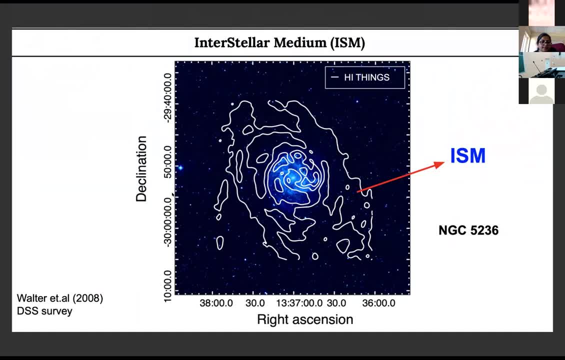 atomic hydrogen atom, or in short, H1.. So here is the optical image. what you see in the background is the optical image of the NGC 5236 galaxy obtained from VSS survey, And this white quantus represent the H1 column density H1 profile of the NGC 5236 galaxy from Tink. 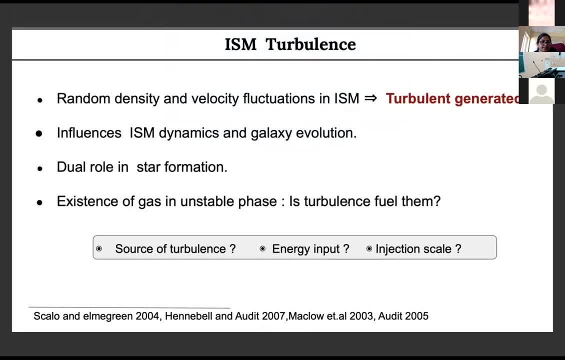 survey. So it is a well known thing that is found to happen in the turbulent dynamics because of the presence of random density and velocity fluctuations. ISM turbulence plays several roles in the different activities in the galaxy. For example, it plays a dual role in the star formation activity. like it, sometimes it triggers the 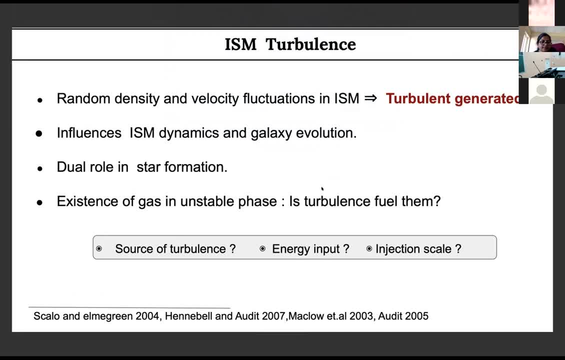 star formations, and sometimes it can hindrance the star formation too. So people have found the existence of unstable phase in the ISM between the cold neutral medium and warm neutral media, and there are hints that turbulence is the fueling factor for the continuous generation of this. 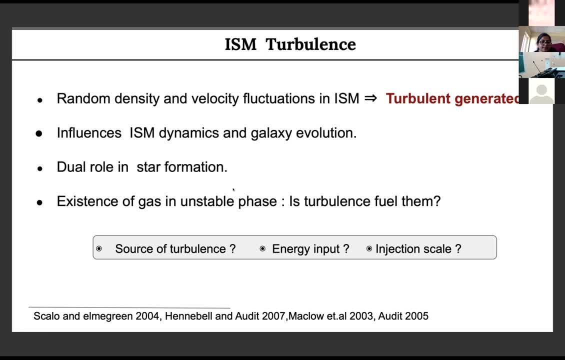 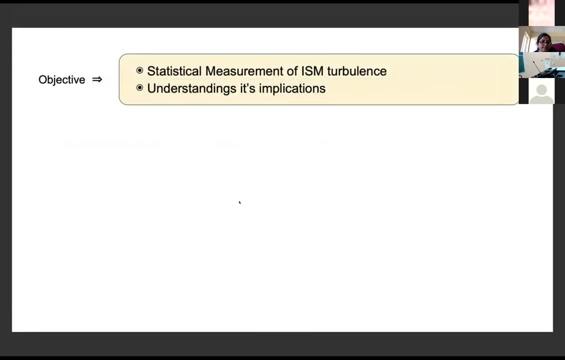 unstable phase. So, even though we know all of this, there are still some questions unanswered, like: what is the source of the turbulence, what is its energy input, at what scale it is injected, etc. So in this work, we are motivated by this question to do this work where we would like to do the statistical 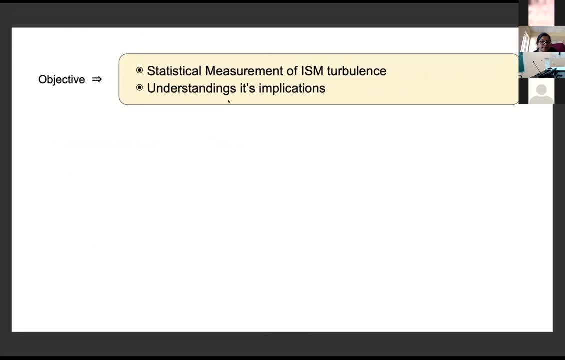 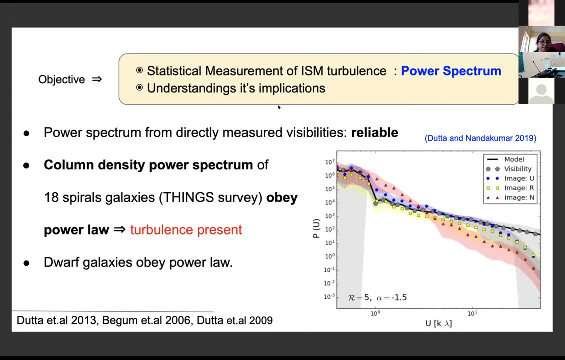 measurement of ISM turbulence and understand its influences. So it is observed from several studies that the ISM have density fluctuations, which are- and these density fluctuations found to have coherent structures that exist from the scales of galaxies to the scales of giant molecular clouds, and these density fluctuations, or the velocity fluctuations can 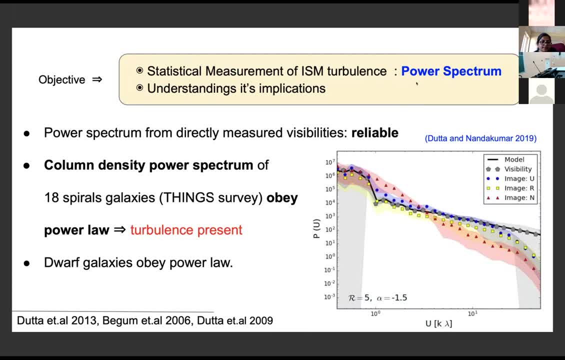 be brought by a tool: power spectrum. So power spectrum is a two-point statistical quantity and the power spectrum of the turbulent generated fluctuations are expected to obey a power law. Datta and Nantagoma 2019 has done a comparative study between the several power spectrums. 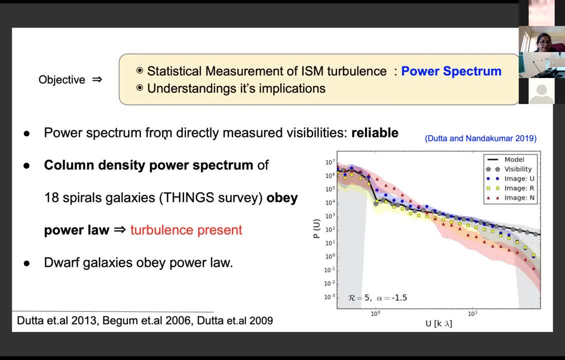 that are available in the literatures and they found out that power spectrums from directly measured visibilities are reliable where visibilities is the quantity that a radio interferometers measures during the observation. So their comparative studies results are basically depicted in this plot. So this is not the first study on the density and 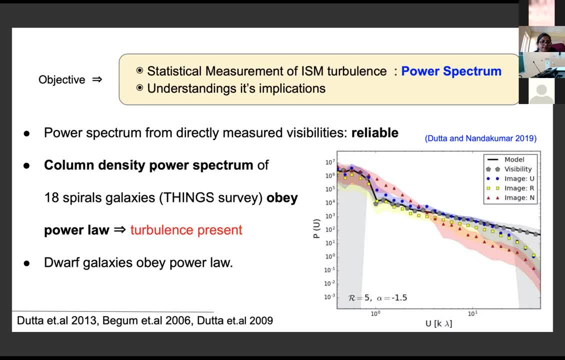 the velocity power spectrum. so there are several studies of densities and velocity power spectrum at a part-second scale, but they are not the first study on density and velocity power spectrum. So scales in our galaxy, Milky Way and recently the title 2013- has estimated the column density. 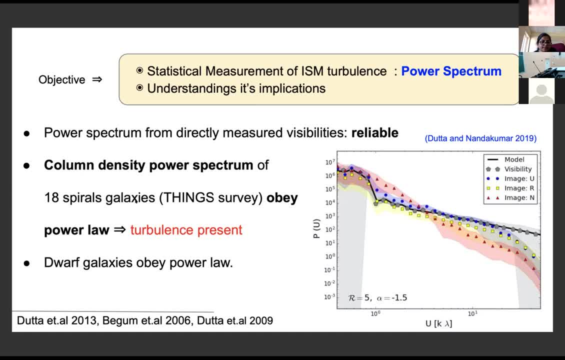 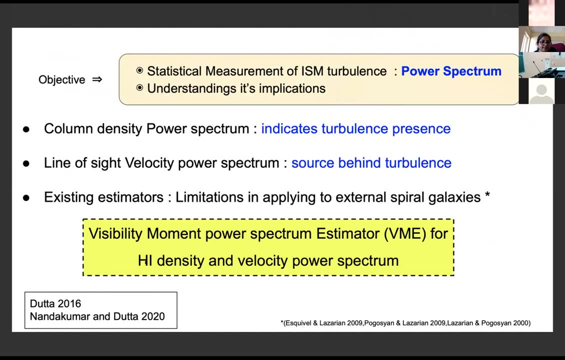 power spectrum of around 18 spiral galaxy and they found that all of them is obeying a nice power law which is indicating the presence of turbulence there. they also found that the power spectrum of dwarf galaxy is also obey power law. So the by the estimation of column density power spectrum, we can indicate the turbulence. 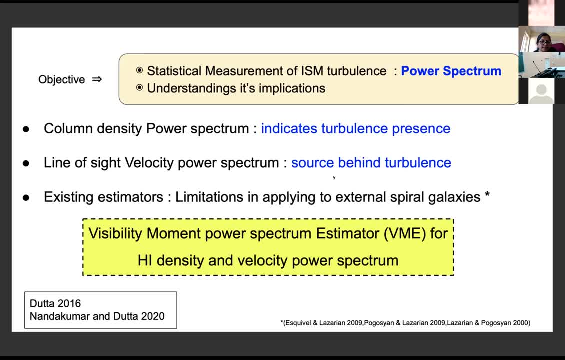 dynamics. but to really understand the source behind the turbulence we need line of sight velocity power spectrum. So finding out. there are several estimators which do the velocity power spectrum estimations in our galaxy, but estimating the power spectrum of velocity in external galaxies rather difficult and DETA 2016 has introduced a method to find the H1 velocity power spectra using the visibility. 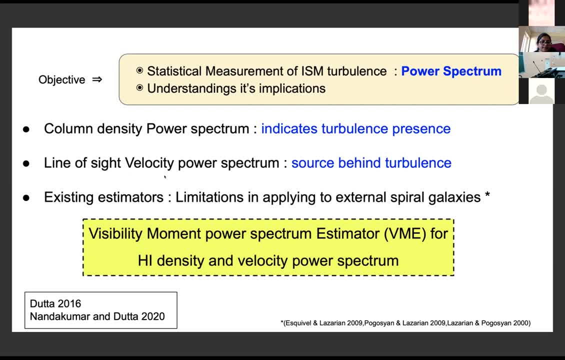 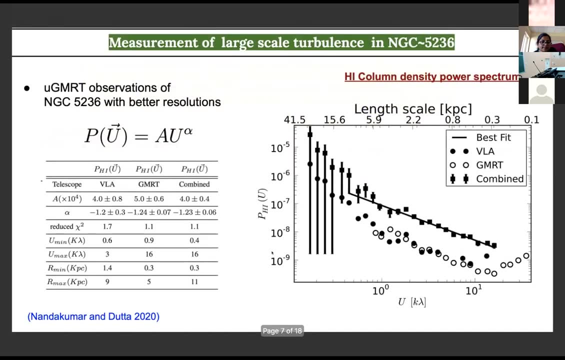 moments. So based on that we did and we implemented a new estimator- visibility moment power spectrum estimator, in short VME, which does the power spectrum estimation for H1 density and velocity, And our first sample for the implementation was NGC 5236 or MISER 83. it is a nice barred. 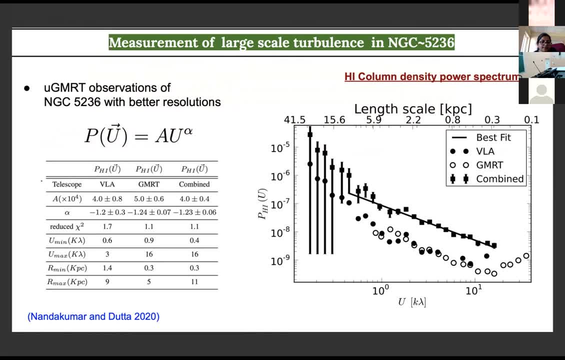 spiral galaxy, which is almost nearly a phase zone galaxy, and we freshly observed the 21cm frequency. So we are able to estimate the column density power spectrum from that observation. so this plot basically represent the results of that estimations. So here the white open circles are representing the power spectrum: column density power spectrum. 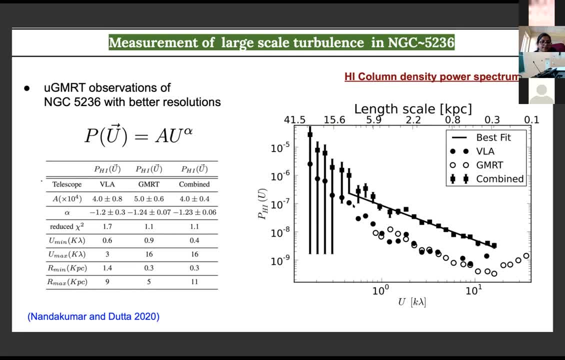 obtained from UGMRT observations and the black circles are representing the previously estimated power spectrum from things data. So we combine these two data to obtain a better power spectrum. So the final combined power spectrum is what given with error bars. So we can clearly see a nice power law is following here which is indicating the presence. 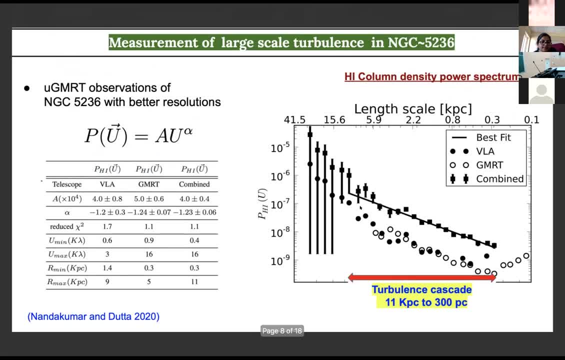 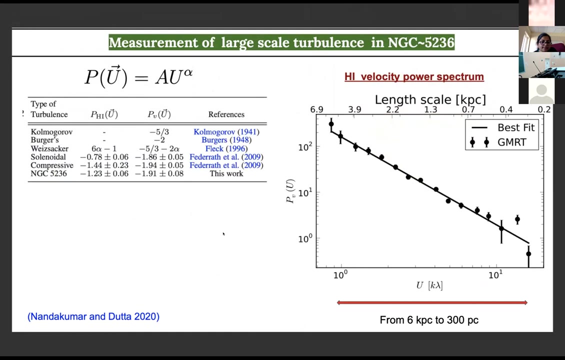 of turbulence cascade, that ranging from 11 kpc to 300%, which is almost around two decades of length. scale And The slope of the power spectrum is around minus 1.23, which is consistent with the previous results. So by doing this estimation, we were able to crop the column density power spectrum to 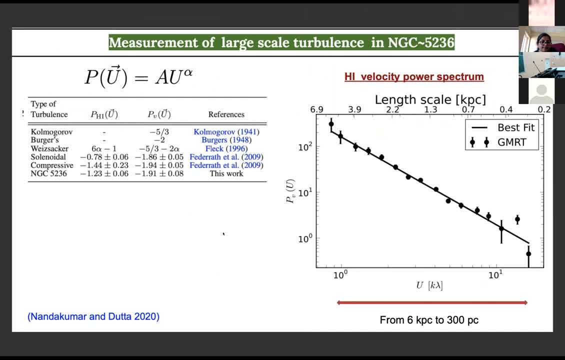 an extra one more decade of length scale compared to the previous results and we, using the visibility moment estimator, be able to measure H1 velocity power spectrum also and, to the best of our knowledge, So this is the first ever measurement of H1 velocity power spectrum in any of the external. 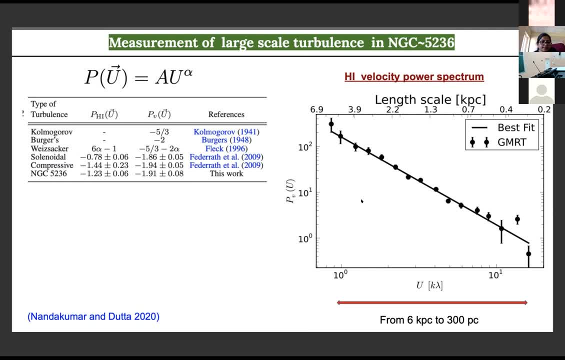 spiral galaxy. Not surprisingly, here also it is obeying a nice power law that, as you see in this plot, which ranging from around 6 kpc to 300%. so there are several simulation to see how, how, what values of slopes you can get for the density and velocity power spectrum for different. 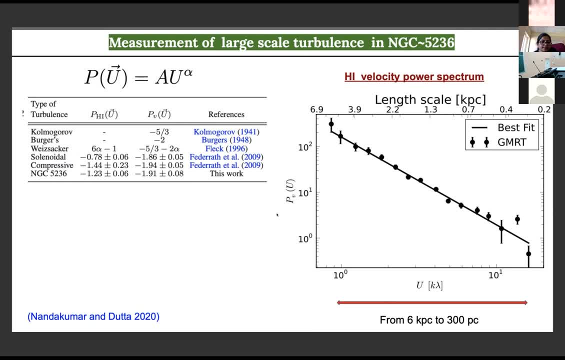 cases of compressible turbulence, like different types of forces. So this is the first ever measurement of H1 velocity power spectrum in any of the external spiral galaxy. We are now on the fourth step, so I will show you how we can get so many different types. 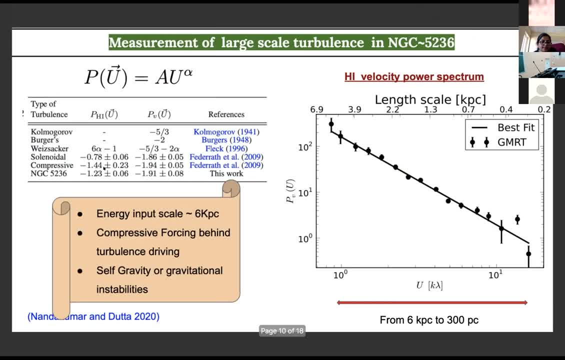 of forcing, like solenoid, compressive forcing. so those slope values are given in this table. So these are the slope values that we okay. so comparing the results, from comparing our results, from this simulation result, we able to conclude that the forcing behind the turbulence that we measured here is compressive in nature. so the possible origin for the this measured, 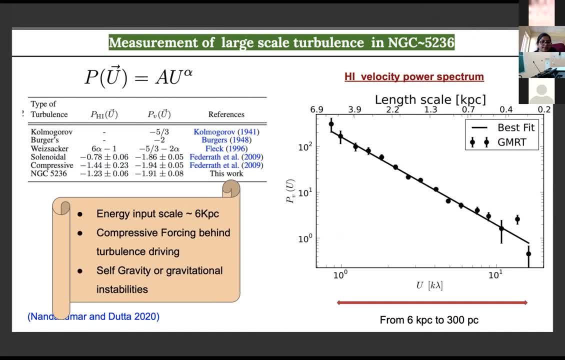 turbulence is either self gravity- We can measure themaddle strength, which is the force points that we measured here- So the possible- or the gravitational instability. so by this we able to successfully measure the larger scale turbulence in galaxy 5236. now the next question is: what is its implications? so first we are: 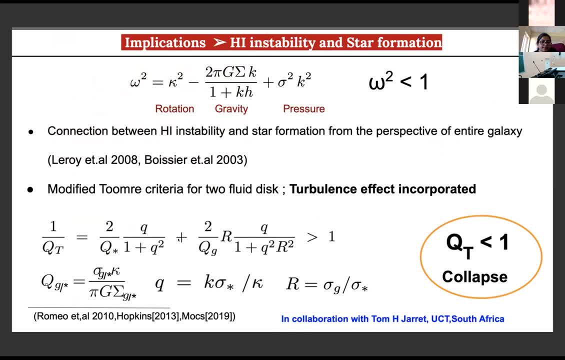 interested in to see its influence in staff formation activity. so here is the basic h1 instability- sorry, instability- equation. so, which is a well-known thing. and so when there is a competition happens between these three terms- rotation, gravity and pressure- and when that gravity wins, that in that competition collapse happens, and that is the condition omega square. 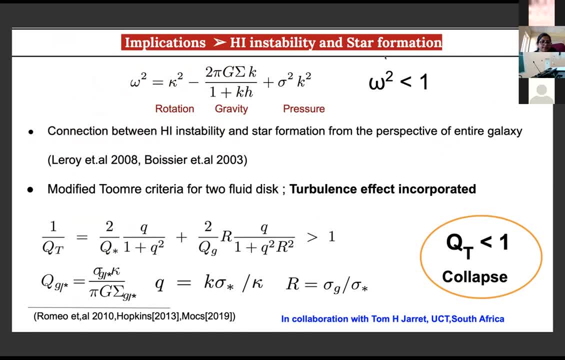 less than one basically tells you. so people have studied the connection between h1 instability and star formations from the perspective of entire galaxy. so here, like daily, take lot of samples of galaxy and do the check, the investigation, investigate the connections. but here we are interested to uh. 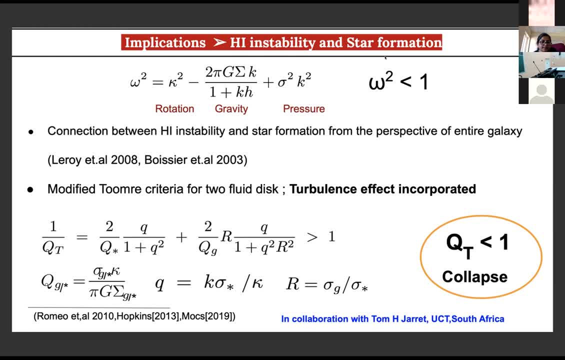 find, uh, how staff formations are connected with other things in the particular galaxy at different length scale. so we use the modified tumbray criteria parameter criteria for the two fluid disk model. so this is the tumbray criteria parameter which is defined in this way. so 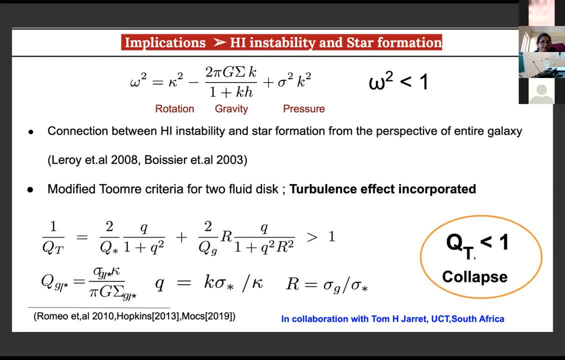 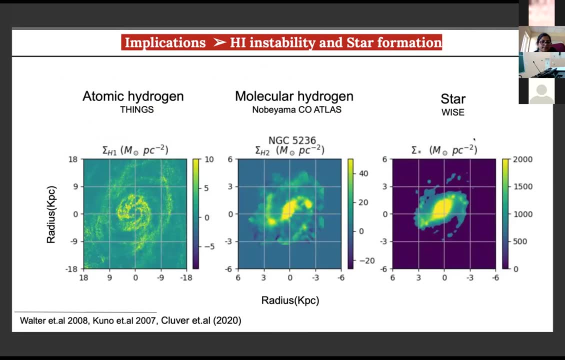 the condition for the collapse is qt less than one. so here we have include the effect of turbulence also, so i am not discussing it, the analysis, in detail, because of the time constraint. yeah so, so we need both gas component and staff component. so the in star mass maps were obtained from y, so 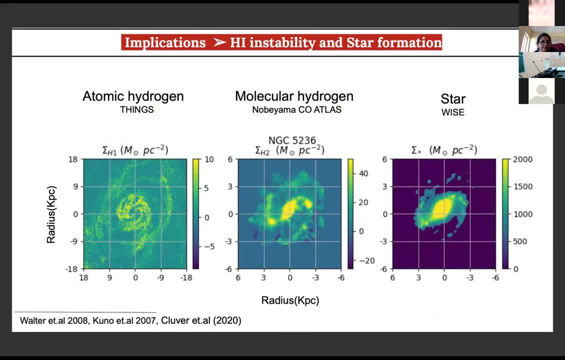 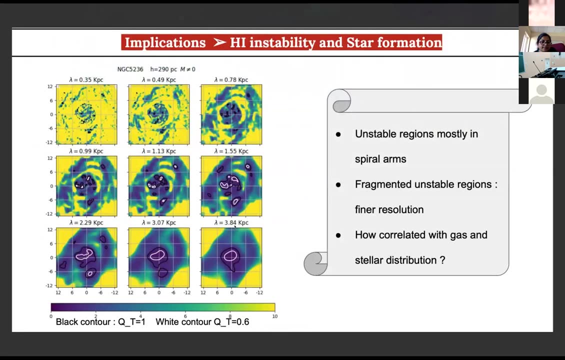 see this- were obtained from our collaborator thomas jared, and the gas part, both atomic hydrogen and molecular hydrogen data were obtained from the archivals. yeah, so using these data, we able to generate the qt maps of the galaxy at different length scale, at different resolution scales. so 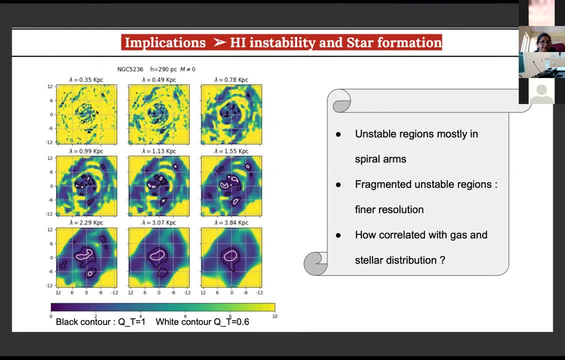 these are the qt maps generated at different length scale ranging from 300 parsec to around 4 kpt. so the black contour line represent qt value equal to one and white contour represent qt value 0.6. so what this means, the whatever the contour regions, what you're seeing is essentially unstable. 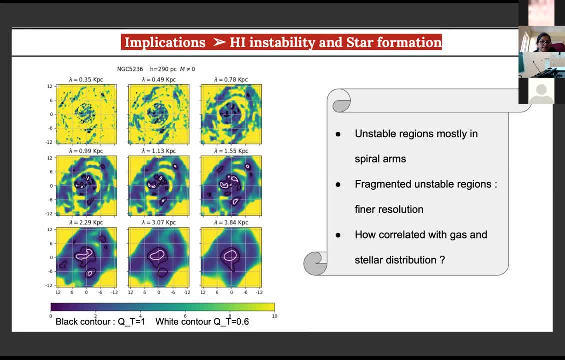 regions. so happily, we could able to detect unstable regions in most of the length scapes, and most of the uh unstable regions are from our cluster and the other cooldown regions, so we're following the spiral structures where the sub formation activities last. now the question is how these unstable regions are correlated with the gas fractions or how it is correlated with 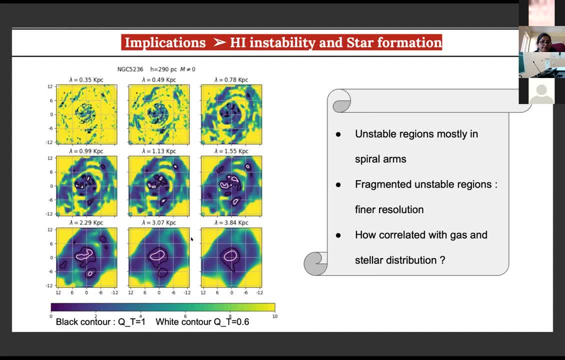 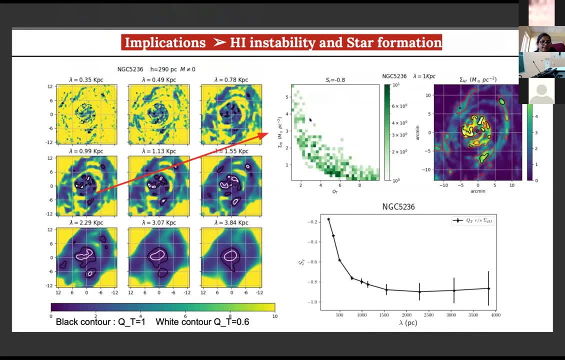 the h1 present there. so to do that, what we does is for a particular length scale, we try to plot the correlation plot between the qt for qt and the h1 surface density. so the in this map, in this density map, what you see in the background is the surface density of the h1 and the contours. 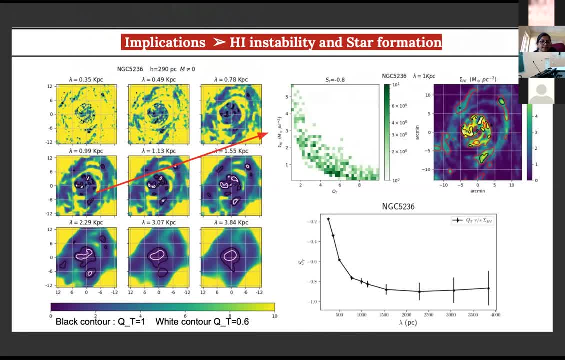 represent the qt values. so we can clearly see that the small values of qt, so this qt values, are small values less than two. the contours represent the qt values less than two. so these values, so the smaller qt values, are highly correlated with the high densities in the h1, which is the. so that strong anti-correlation between the 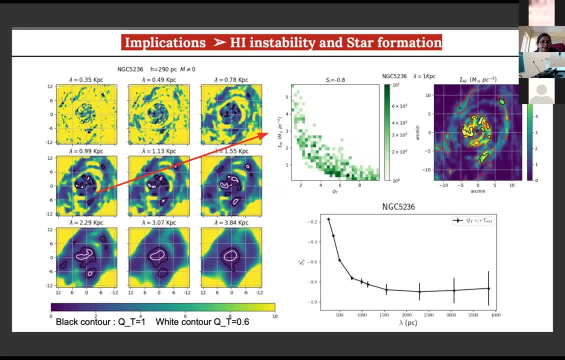 qt and the h1 is nicely seen in this correlation plot. also, the Spearman correlation coefficient is around minus 0.8. so we try to see how this correlation coefficient will be at different length scale. so we did this analysis for all these. so we did this analysis for all these length scale. so we did this analysis for all these. 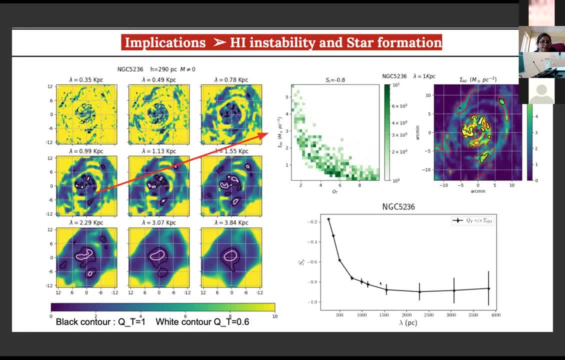 Long scales and that Spearman correlation coefficient plots are given over here as a function of length scale. so we can clearly see that the QT values and the H1 mass are highly strongly, strongly anti correlated, Strongly anti correlated at a larger length scale, which means that the possibility of finding high density H1 re-H1 in unstable regions is large. 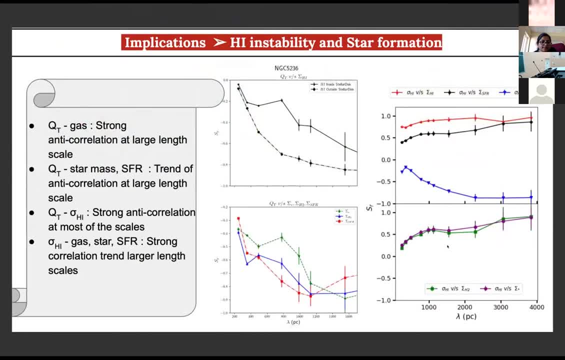 So we did a similar analysis by taking different combinations of spares to see what is happening actually. so we tried to find out the correlation between QT and H1 gas, Then QT and H2 gas- H2, then between QT and star formation rate, star mass, star maps then. 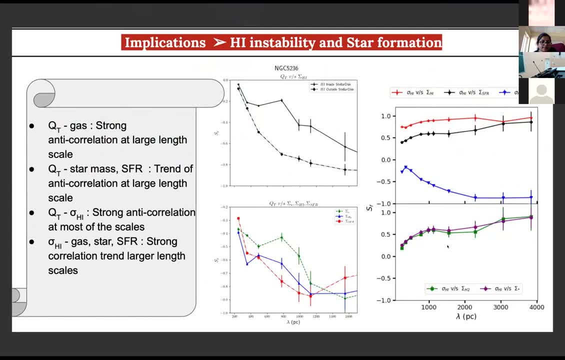 between the we find the correlation between QT and H1 velocity dispersion, which is kind of an indication for turbulence. So these different plots are basically representing the results for the different correlations, so how the correlation coefficients are varying at different scales. So the overall conclusions that we can draw from this graph is this: 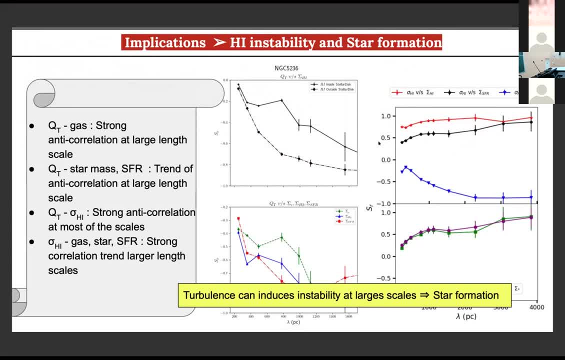 Meera, you have two more minutes. Yeah, So the overall conclusion of this plots are basically in this way that wherever unstable- so the unstable regions are highly correlated with high density, high density of H1.. So the overall conclusion of this plots are basically in this way that wherever unstable, so the unstable regions are highly correlated with high density, high density of H1, H2, and H1 velocity dispersion. 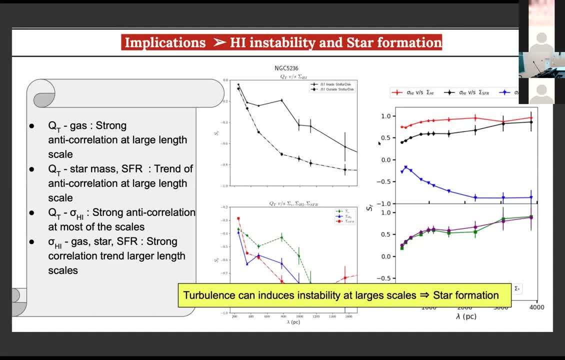 That means it is saying that possibility of finding is seeing H1, high H1 mass regions and high H1 velocity regions in unstable regions are high. So basically this is indicating that turbulence is playing a significant role in inducing instabilities. So this was one of our 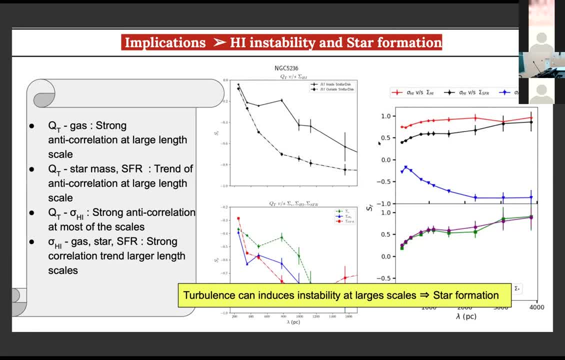 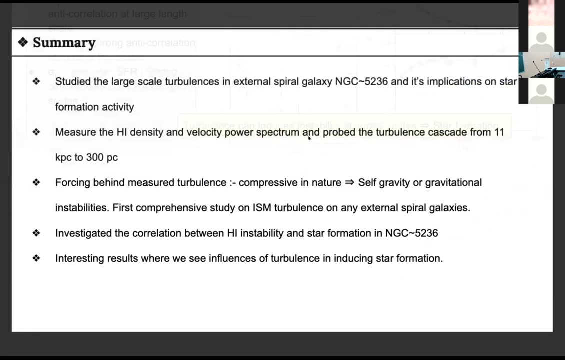 aim to aim in this work. So this work is currently in the process. so this is just the preliminary results of the analysis. So in near future this work will be presented in a coherent manner. So by this I will end my talk, leaving the summary slide to you. Thank you. 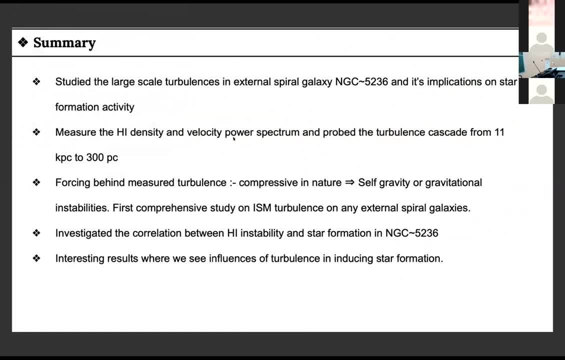 Thank you, Meera. We have time for a few quick questions, If there are any questions in the lecture hall. yes, yes, ma'am, there is a question. yeah, please go ahead. sorry, uh, the kolmogorov spectra that you drew i saw at various places. it was deviating from from the kolmogorov. 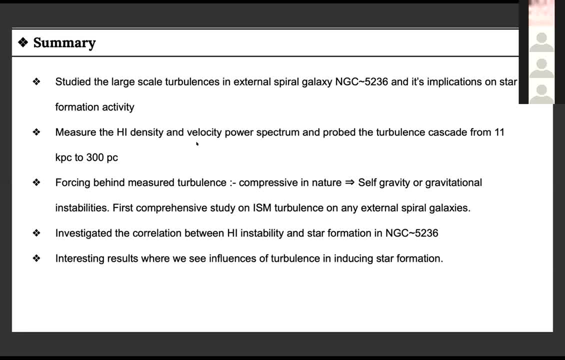 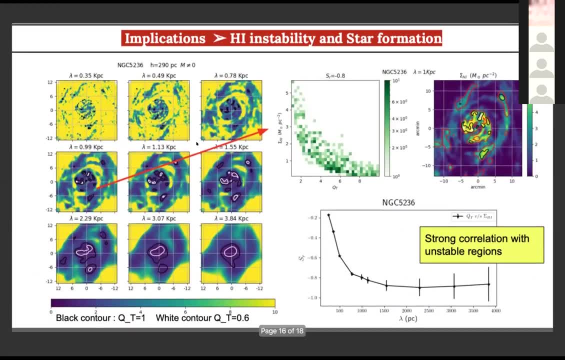 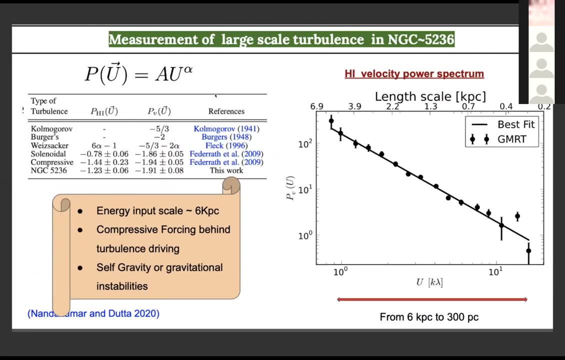 uh, parlor, uh, index, uh, could you just throw a light on why do you, why it's happening and what do you think why it's happening? okay, i didn't understand that. i understand your question completely. uh, did you mean this? no, no, no, no, go back, go back. yeah, yeah, this one, this one, this. 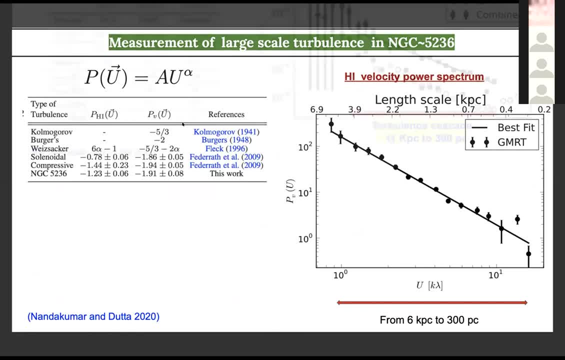 yeah. so i think, yes, oh, this one, no, no, no, it appears that just go back one more. yeah, not back. so yeah, this one. so you see, at uh, at higher, uh, k lambda, you, uh, sort of there is a jump and then it comes down, right, yeah, yeah. so it is deviating, i don't. 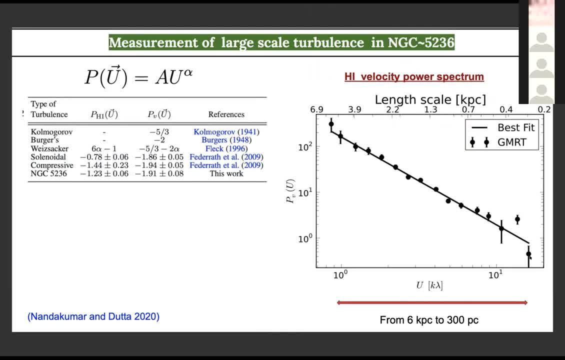 know what is the? what is the power law you got? it is minus five, third. that is what i got is minus 1.91. okay, okay, that's, that is the slope of the slope of the bus spectrum, so this is like compressible turbulence. okay, so it's, it's deviating. 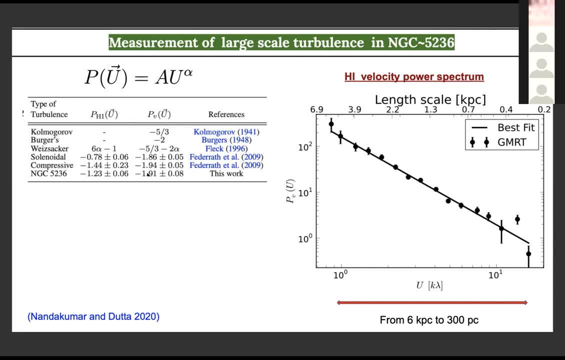 from the kolmogorov minus five third right. why is it that? i mean you have any explanation for that or any speculation for that. so i mean, what i meant is: uh, i think i'm uh in, i think kolmogorov turbulent, kolmogorov is. 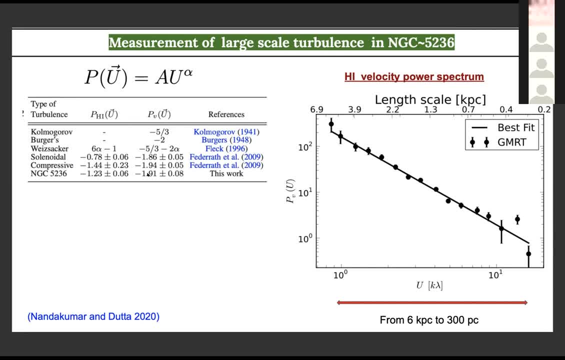 for incompressible turbulence. but what here? what we are looking at is the compressible turbulence. what can be the reason? i'm not sure. hello ma'am, there is no question from offline audience. okay, so are there any questions from the online participants here? you can also type your questions in the chat box. 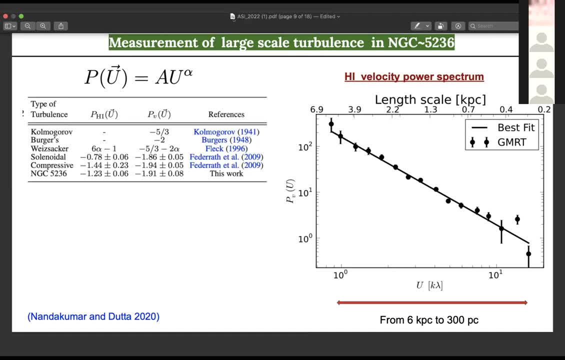 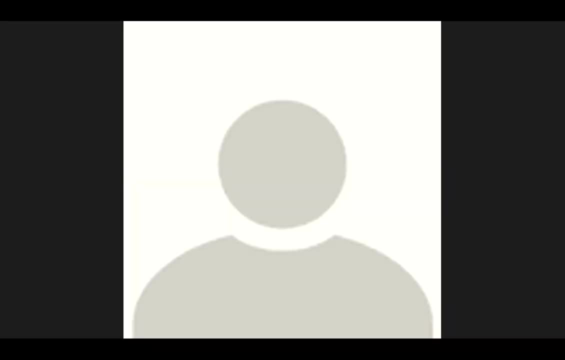 in zoom and also make use of the chat box. if you have any further questions, please email us at swedish chat box or at the uh the facebook page of the facebook channel. so if there are any questions, let us thank mira for this talk. mira, if you can please unshare your slide? uh, the next speaker in this session is uh. 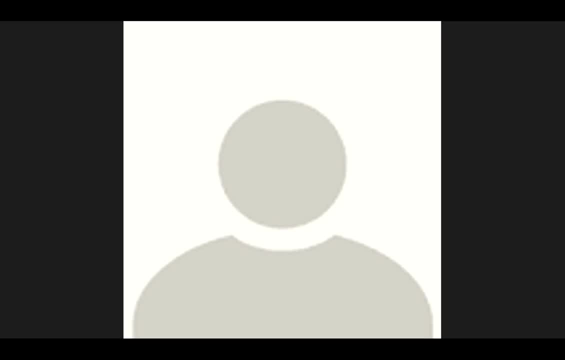 prasoon dhal, and he will be speaking about generation and transport of large scale magnetic fields and accretion flows. so, prasoon, i will give you a warning at 12 minutes, at 10 minutes. okay, sure, ma'am. thank you for your attention and we will start the next session very soon. 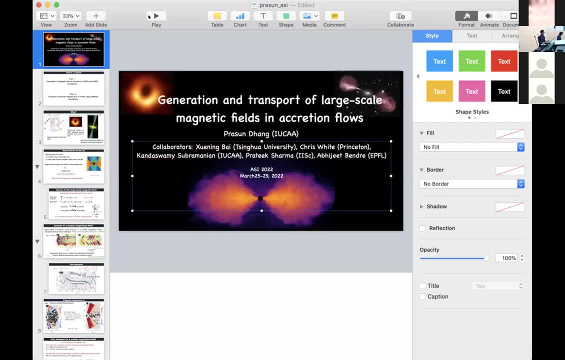 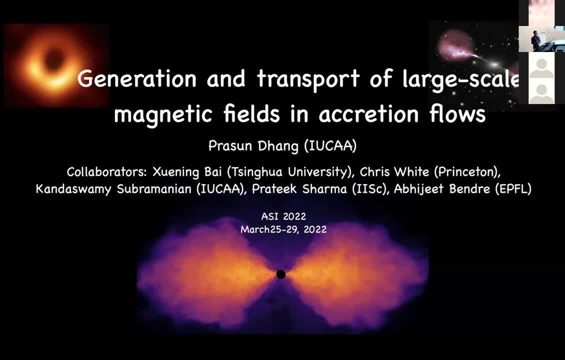 so, so let's start. hello, yeah, please start follow our mic. morning everyone. uh, i'm prashant, i'm a postdoc at ayuka and in this talk actually i will talk about something on origin of large scale magnetic field in accretion flows. so it's a kind of a huge 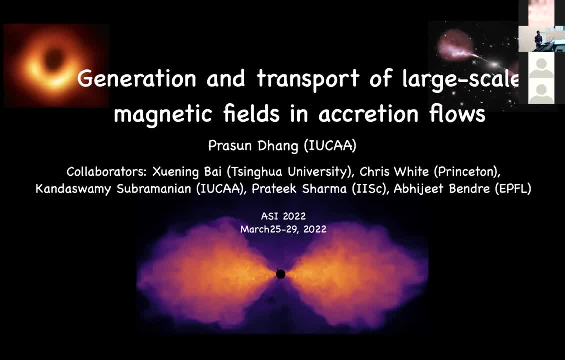 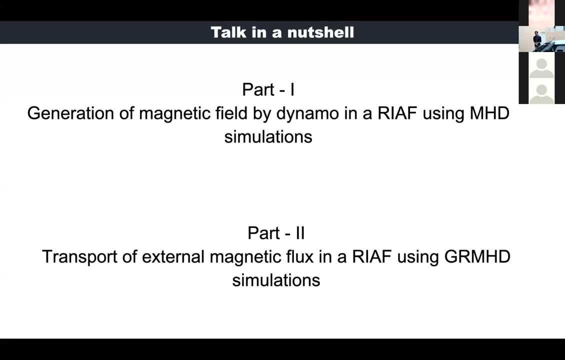 topic, so i'll quickly go through it. so you have. if you have any question, please feel free to interact in chat slack. so why are we basically studying it? um, that i'll talk later. so there will be two parts of my talk. in the first part i will talk about the generation of large scale. 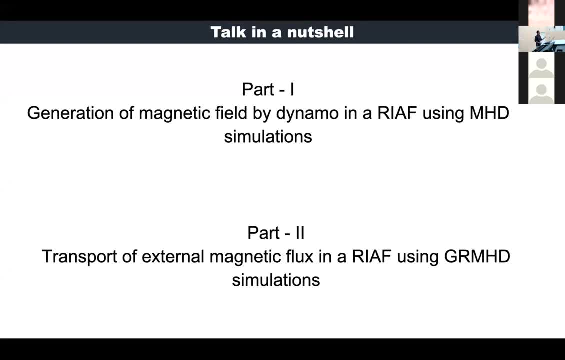 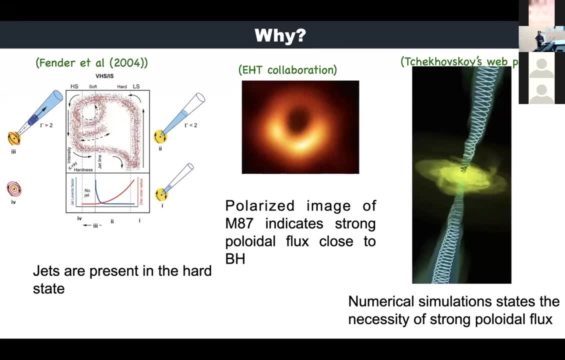 magnetic field, and in the second part i will talk about the transport of external magnetic flux in the accretion flows. so, basically, why are we studying it? the reason is some observations and and theories. let's first look at the first picture, um, which is, uh, a famous scheme diagram for black hole binaries. so jets are actually present in the hard state of 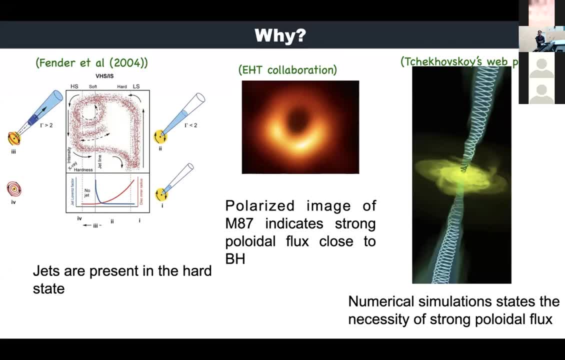 this uh sources, this transient source, like this thought that uh, there's a hot accretion flow, exists close to the central equator, in this hard state. also, if you, if you are uh, probably have seen this second image, which is a polarized image of a medicine black hole, which is also a checkered asian. 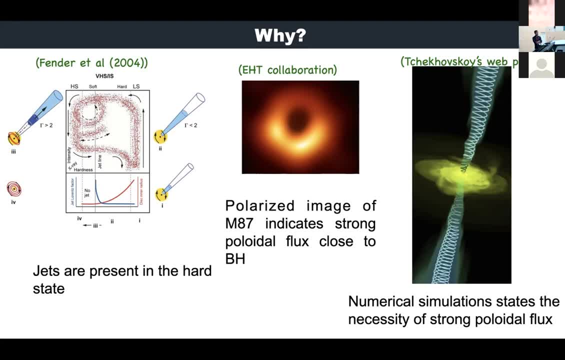 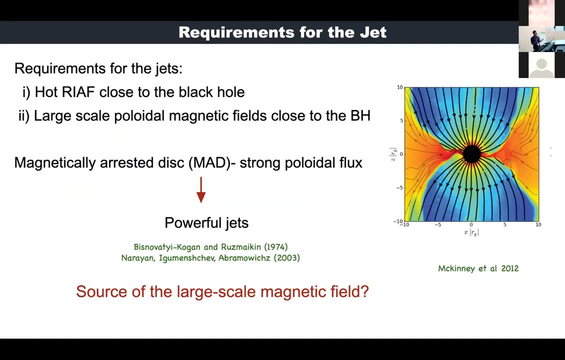 and the recent observation shows that there's a presence of a large magnetic field close to the black hole, and different theories- also numerical simulations- informs that we need a large scale magnetic field in order to produce jets. so if i summarize all this observation and theories, the crux is that we need a hot accretion flow close to the black hole and it should be saturated with. 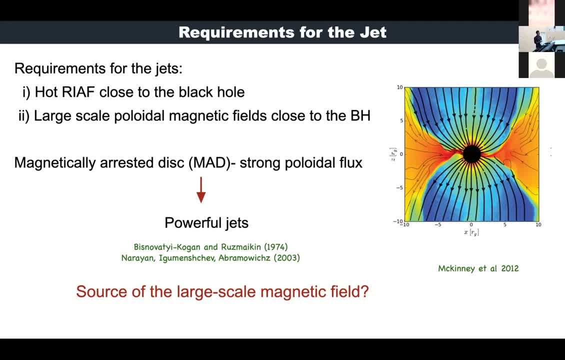 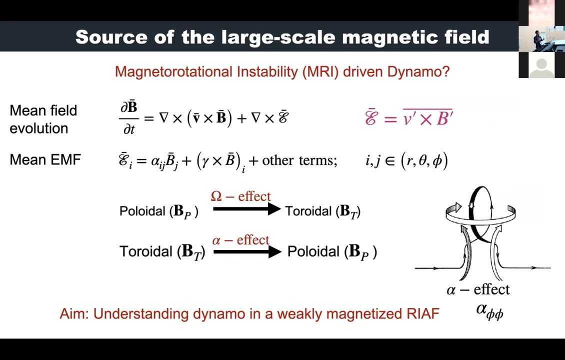 large scale magnetic flux. this is the requirement for jets and this has been realized in numerical simulations and the model is called magnetically. understood this, uh, but the question would be: what is the source of large magnetic field? now, the first case is that, okay, the large magnetic field is generated in the disk itself. 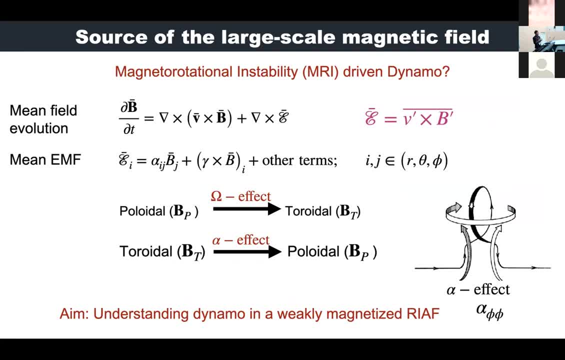 or in the ray of itself, by a emerald driven dynamo which is responsible for the environment and transport. now, before going into the results, let's uh look at this equation called mean field evolution equation. the first term in the first equation is basically: uh is responsible for the 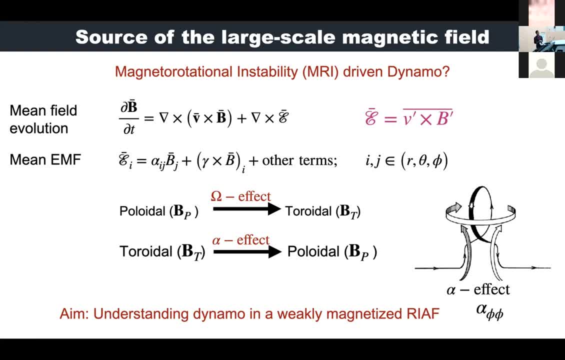 generation of colloidal field from the colloidal grid, and this is something called famous omega effect. second term, which involves a term called mini mf, uh, which is which arises because of the correlation between the fluctuating velocity and magnetic field, is responsible for the generation of all the field. 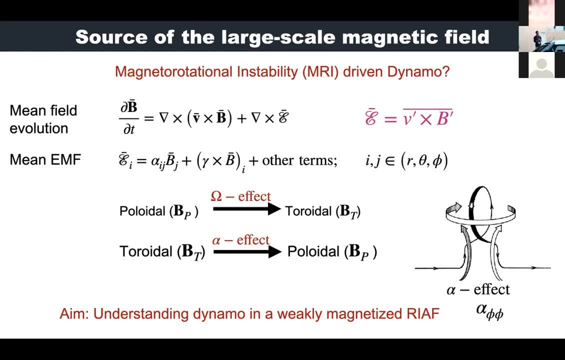 out of the corridor and this is something known as the alpha effect. and if i want to understand what is alpha effect, think about the total field embedded in a stratified medium and, due to buoyancy, when, when it is rising up and if there is some kind of twisting motion, let's say some kind of 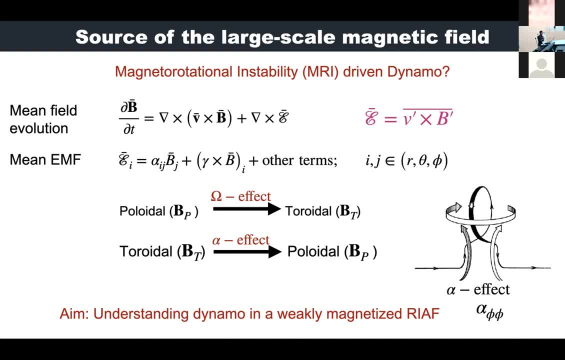 collision motion, then it can generate polarity loops out of the total fields. so this is kind of the picture what uh people think about alpha, omega dynamo, and we want to understand whether this kind of dynamo uh can generate sufficient amount of large magnetic field and right off 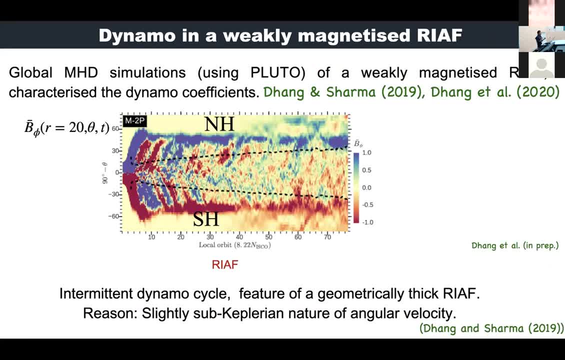 so the first thing people do to uh look at the dynamo is to look at the butterfly diagram and this is nothing but the special temporal variation of the mean territorial field. y-axis is the latitude. so if you are looking at the mid plane is basically a testament and xx is. 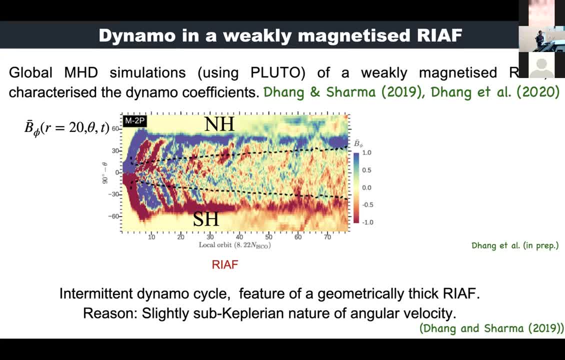 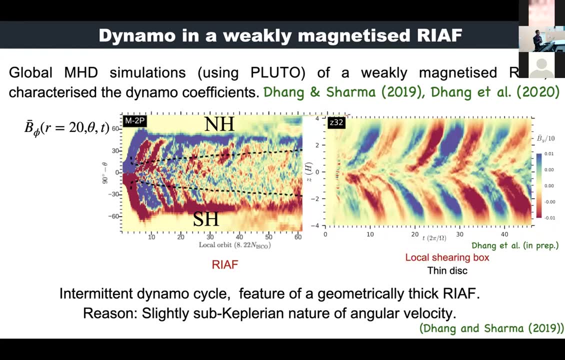 the time and we are looking at a particular radius here. we have chosen as the radius of the 20 short radius, so the computation radius. now you can see the here the mean territorial flips, intermittently or irregularly. if you compare it with the same thing, same butterfly diagram of a. 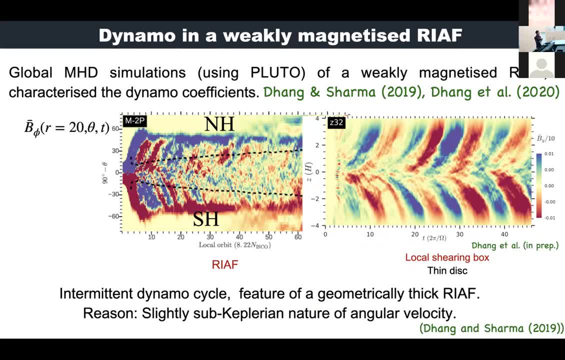 thin disc is pretty regular. so the reason behind this intermittency is the slightly subcapillary of the angular velocity in the ray of, and this is a generic feature of the thick disk. next we look at the helical distribution as a function of latitude. so, as you can see in the mid, 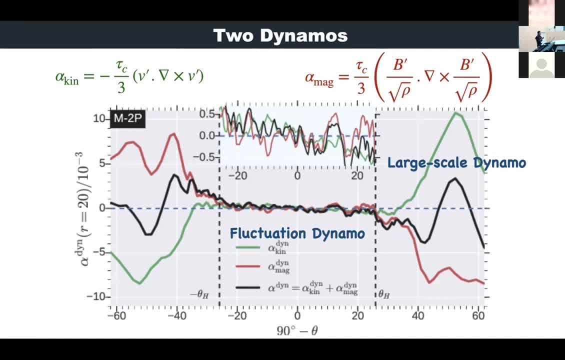 plane and that means at smaller latitudes the helicities are vanishing, while as you go up or down that means you are going at higher latitudes, the helicities become non-vanishing and indicates that that in the mid plane basically, magnetic fields are grown by the 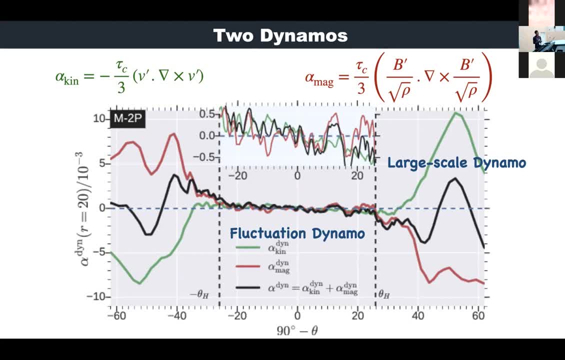 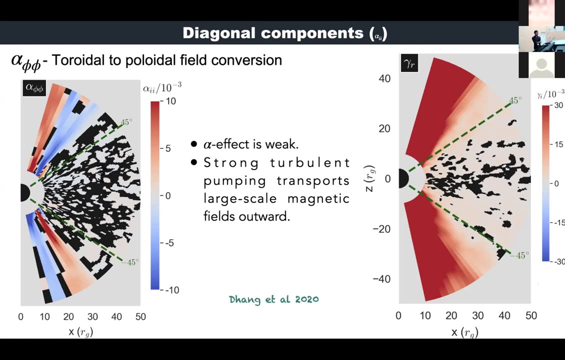 stretch of the magnetic field lines. and this is the reflactation dynamo bus or sponsored dynamo. while we have larger scale heights for larger latitude, a helicity driven large scale dynamo operates and dominates the process. now we also basically quantified, uh, the different dynamo. 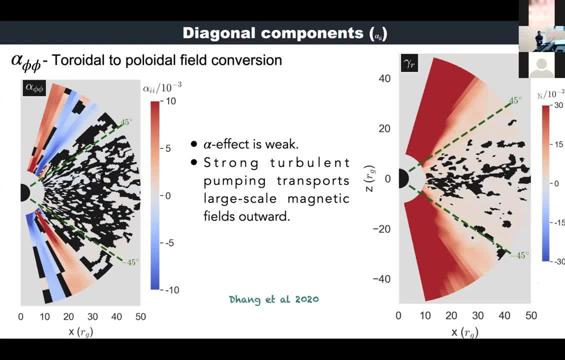 coefficients, as i have shown in the first equations, and out of the many coefficients, i will only talk about the two which are of particular importance. the first one is alpha phi, phi or alpha effect, which is responsible for the generalization of the randomness of the dynamic field lines. this is a 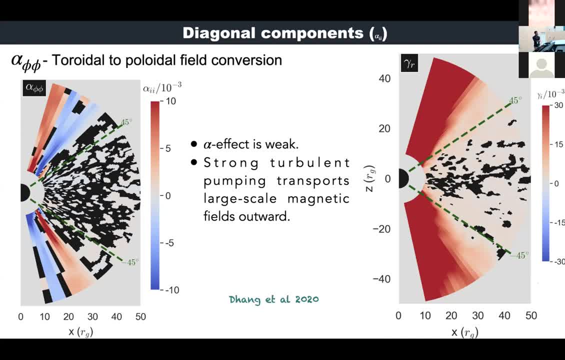 of colloidal field out of the colloidal field, and here I have shown you the colloidal distribution of the alpha-phi-phi in the left panel and, as you can see that at larger latitudes those are actually showing a sign change, while in the mid plane there is a black mask. 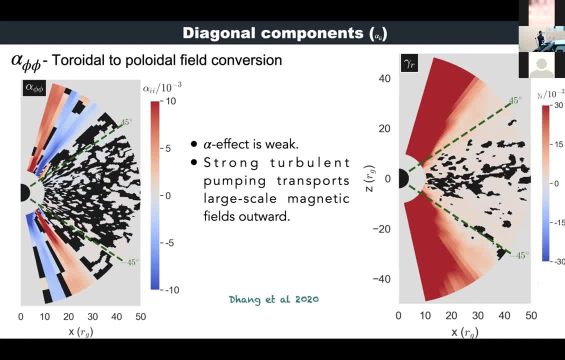 The reason is that in the mid plane small scale dynamo dominates and results are not reliable. So this is kind of fine, but also we found that alpha effect is weak. Next one is the turbulent- something called turbulent pumping gamma r, which is responsible for the generation of sorry transport. 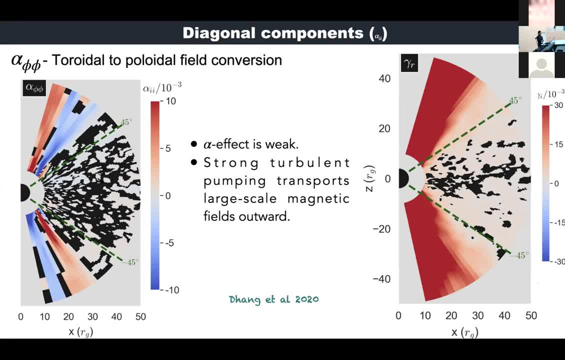 of large magnetic field from the laminar region to the turbulent region and here gamma r is positive. that means basically it is prohibiting to gather the magnetic field close to the mantle. So if I combine both weak alpha effect and strong turbulent pumping then it says that basically in ray of 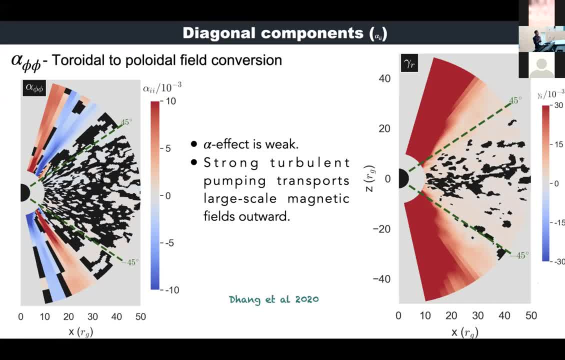 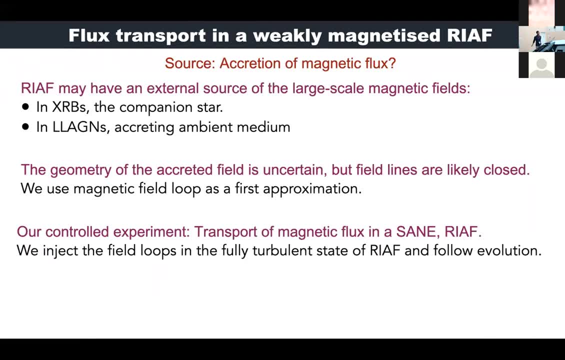 it is difficult for dynamo to produce sufficiently large magnetic field close to the black hole which can produce jets. But there can be another source, something called advection, advection of external magnetic flux from some external sources. Now, for example, in extra minus it can be the. 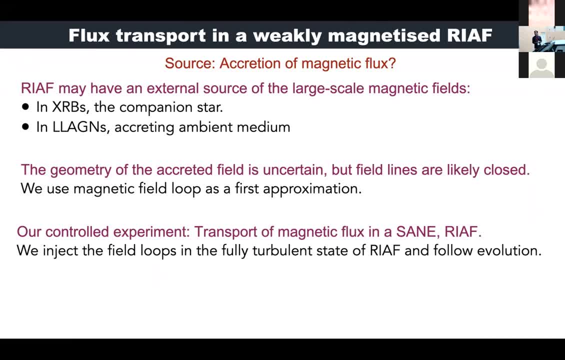 companion star in low luminous agents. it can be the creating magnetic ambient medium which also harbour the magnetic fields. Now actual configuration of the magnetic field could be quite complex, But as a first step we did the controlled experiment of advection of magnetic field loops. 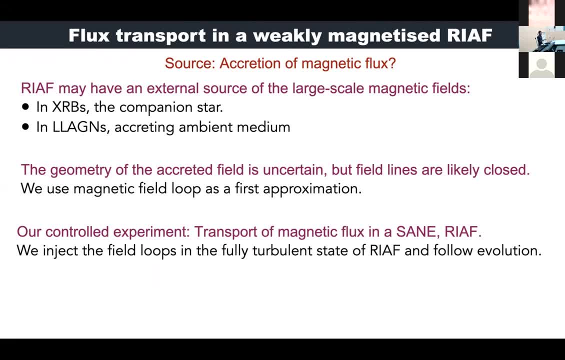 in a fully turbulent raya. So this is a very different from the earlier studies where people have injected the magnetic field in the laminar stage and they have considered it So to my, the best of my knowledge, is this the first study which injected the loops in a fully turbulent. 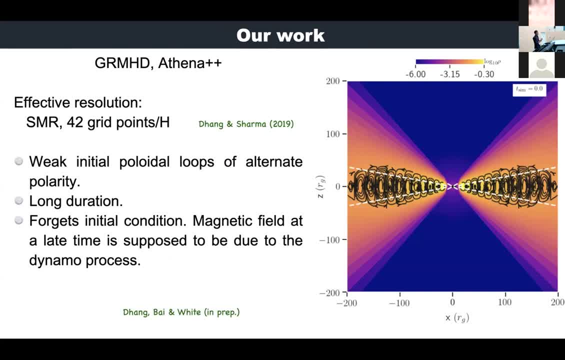 raya. So first attempt would be: we have to construct a fully turbulent raya and row which will forget the initial condition. So what we have done, we have considered the initial polarity field loss and we run it for long enough so that it forgets the initial condition. 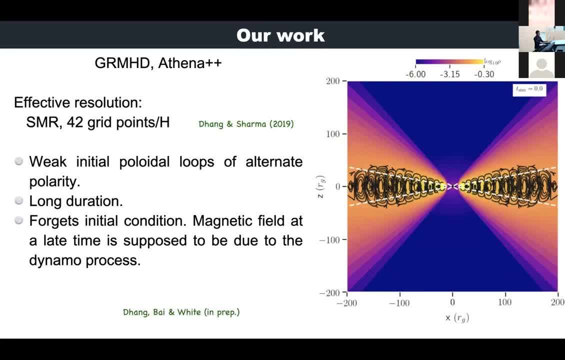 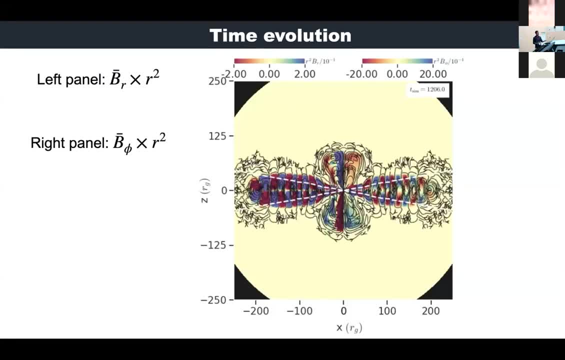 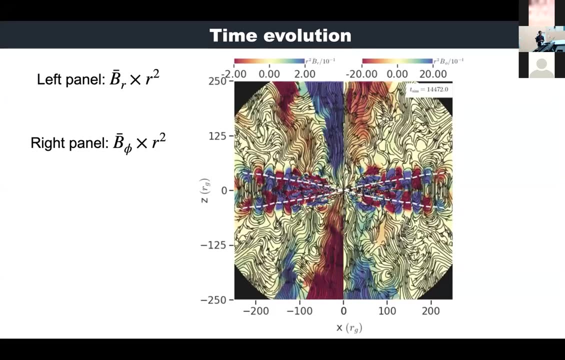 So, by the way, this is a GRMU dissimulation using ether++ code, So let's see how it rolls. So right hand panel shows here the mean B5 and left hand shows the mean BR, and streamlines are basically the polarity field lines. 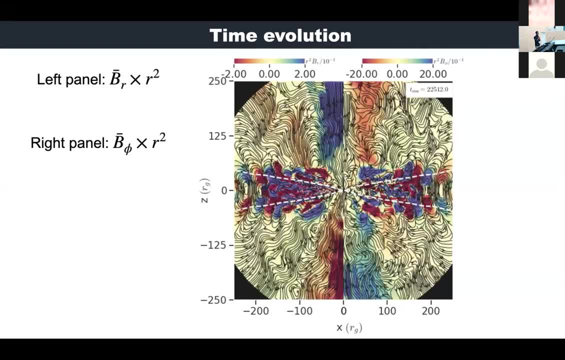 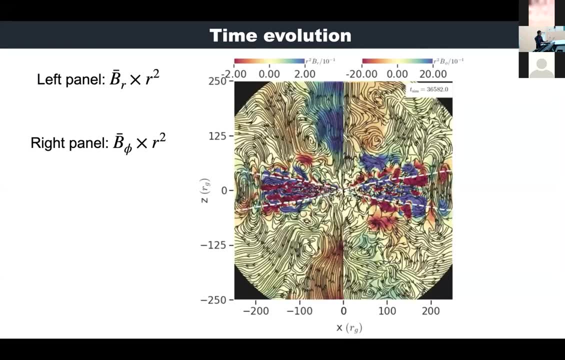 So, as you can see, that MRI basically dominates at the last stages and everything becomes turbulent. So there is no signature of the initial field geometry. So the movie is quite long but due to the time constraint probably I'll skip it. So we want to inject the field lines. 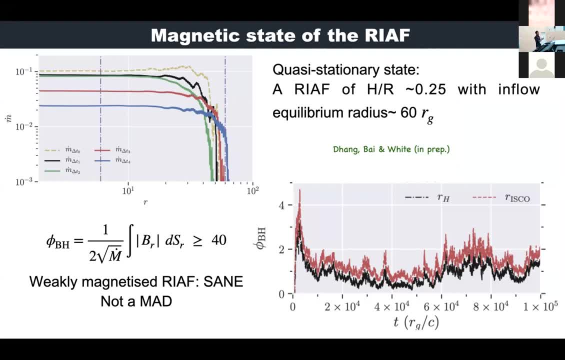 or magnetic field loops in a quasi-station state. So we have to calculate during the runtime how much of the region is in a quasi-station state. This has been defined by something called inflow equilibrium radius, So two diagonal lines to do the diagnosis. 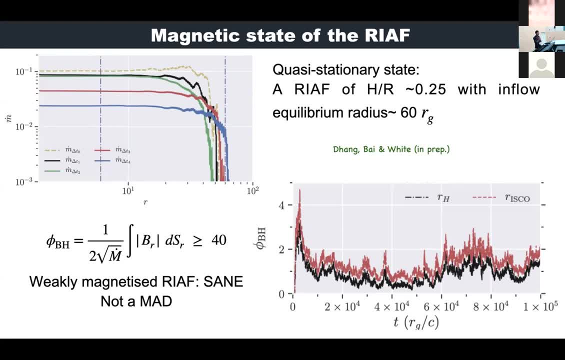 but in two we looked at the radial profiles of mass accretion rate at different times. So blue line is the latest type of the simulation and wherever the region is flat, we call it an inflow equilibrium radius. So for the blue line, 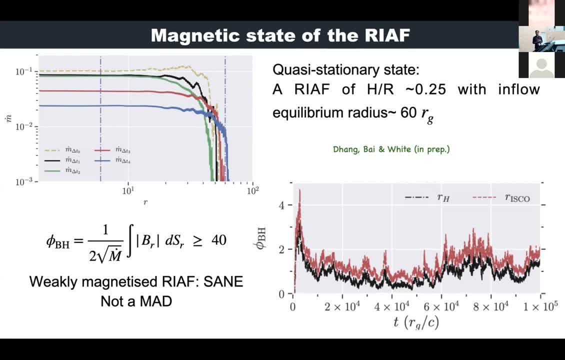 you can see the roughly the inflow equilibrium radius could be around 60.. Next, I also, as I have told, I want to inject the field lines in the weakly magnetized dry off. So I want to see something, whether it has reached MAD or not. 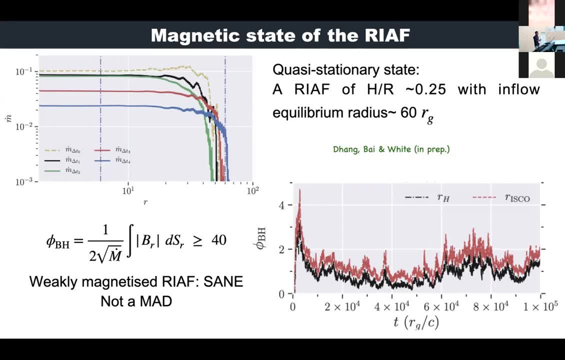 And to quantify it, you can look at something called MAD, MAD parameter or 5H, which is basically the radial flux threading the event horizon of the black hole and normalized with the square root of mass accretion rate And if it is of a critical value, 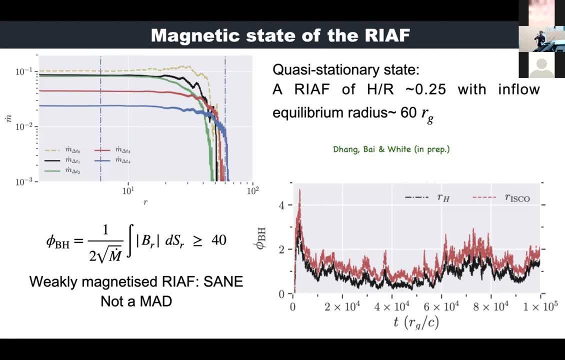 let's say 4T, then we call it a MAD. Now in our simulation you can see in the bottom right that throughout the simulation it is always driven below two, So which is a kind of supersend regime. There is no MAD at all at any time of the simulation. 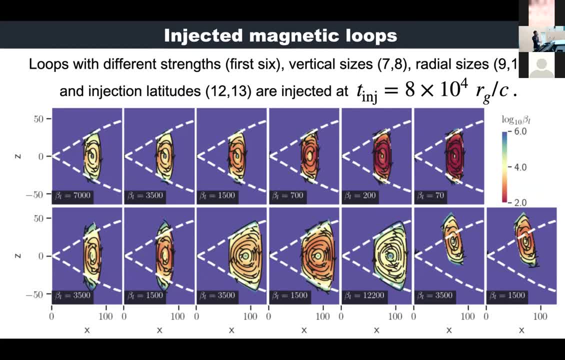 Now, in this stage, we want to inject the field lines, inject the different magnetic field loops of different strength, as shown by the top six panels, different vertical size and different radial size. Also, we look at the effect of injection location, as shown by the last two panels. 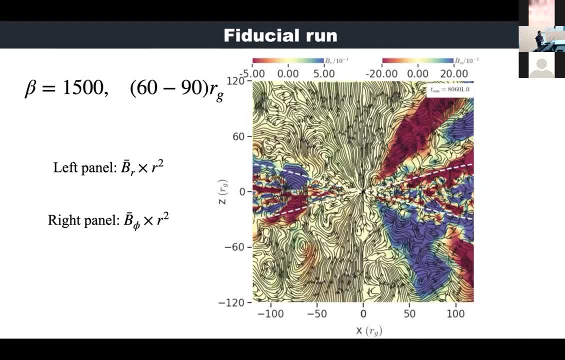 Now let's see how it happens if I inject the external magnetic field loops in the turbulent dry off. So you can probably see in the left-hand panel the loops were pretty clear. I think it's clear, let's see, And we have injected the loop. 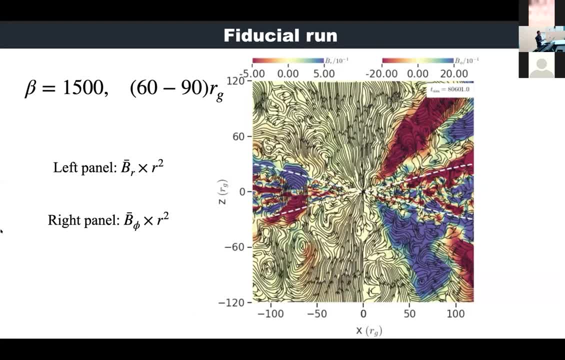 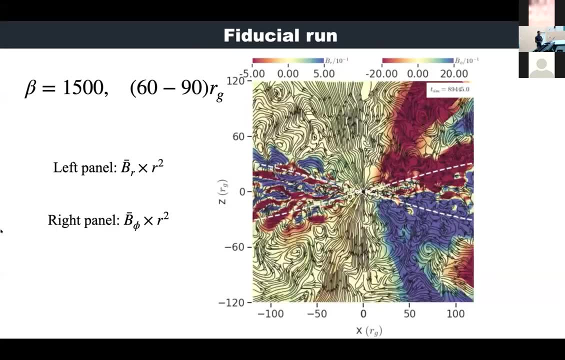 in between 60 and 90 gravitational radius of plasma, beta 1500, which is kind of moderate And let's see how the loop does. So it is slowly drifting towards the backbone And, as you can see that it is enhancing the magnitude of the magnetic flux. 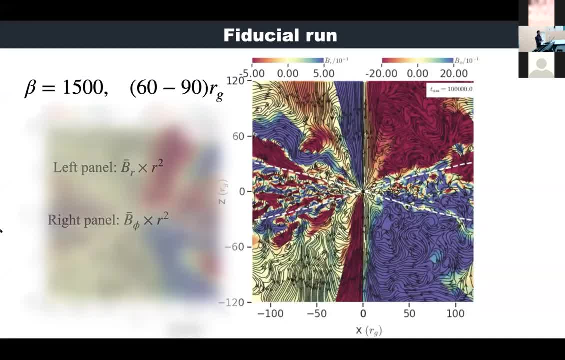 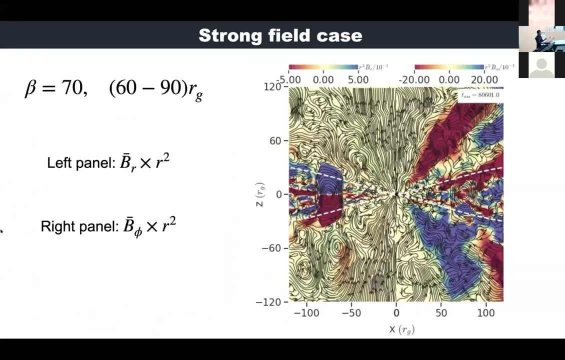 close to the poles And if I compare it with the original dry off run without injecting the flux, you can see the difference. So some of the flux is really reaching the backbone, but slowly. Now let's consider a very strong flux. So beta small means strong flux. 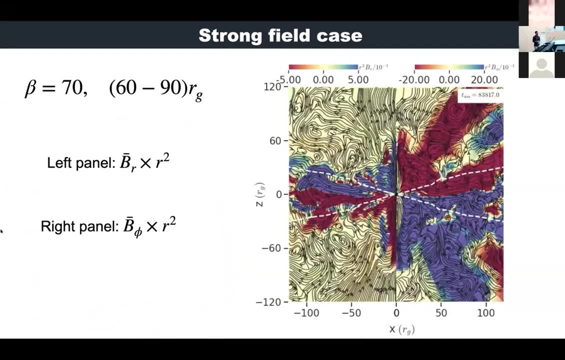 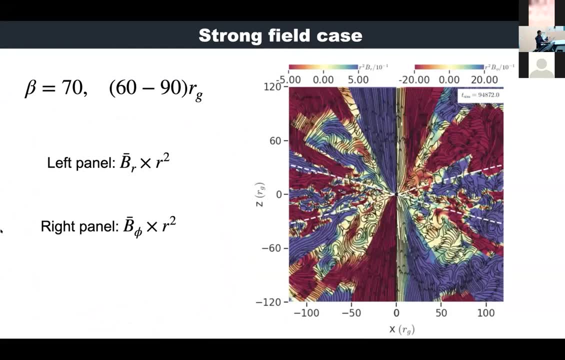 So here you can see, this just quickly plunges through the backbone, And this is probably expected, because it generates the large-scale stresses which transports the material, as well as the magnetic field, very quickly. Now, different magnetic fields loops will harbor different amount of magnetic flux. 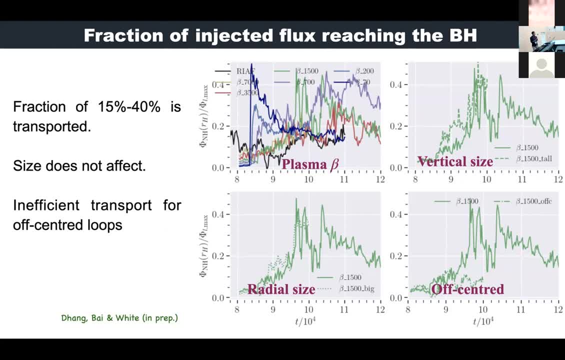 but we are particularly interested in the efficiency. That means we want to look at how efficient the transport process is. So we look at different things like plasma-beta, which will define the magnetic field strength, vertical size, radial size and also injection location. 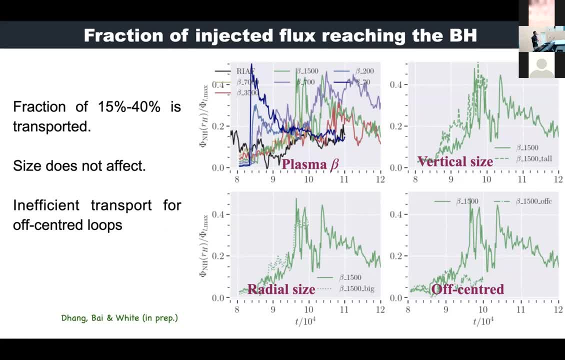 will be considered off-center loops. We found that around 15% to 14% of the magnetic field loops are being transported to the black hole. The rest of them will be diffused or reconnected, And we also find that size doesn't really matter in this case. 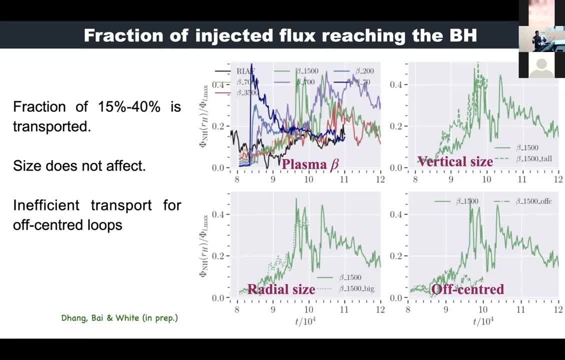 At least the parameter space we have scanned for Either vertical size or radial size Interesting. So this is a good example. Interesting thing: we found that off-center loops are poor show poor efficiency of The reason behind that for the off-center loops. 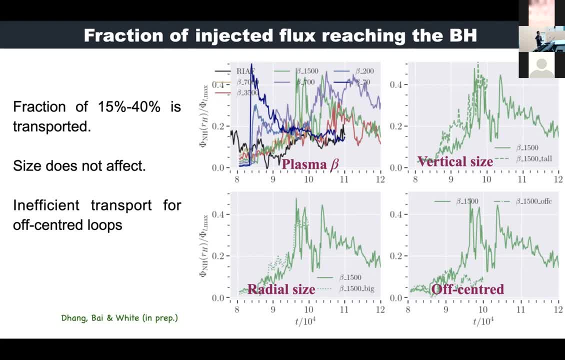 due to the shear. both the torridal field will be converted quickly to the torridal field in a dynamic time, And it will-. You have two more minutes left. Yes, this is my last slide, So it will create the torridal fields. 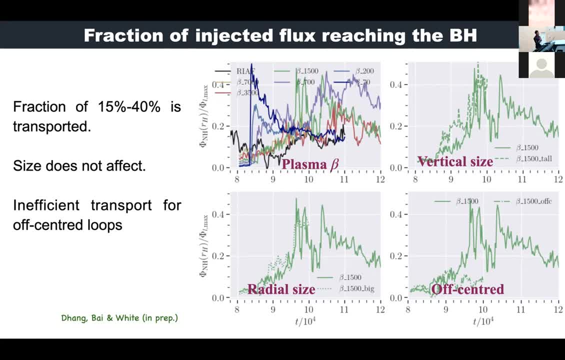 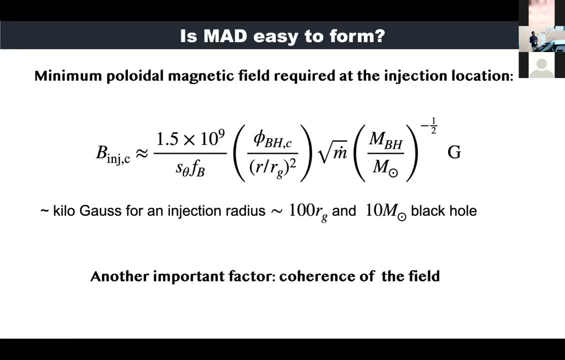 of alternate polarity in the same hemisphere And it will quickly reconnect and diffuse, So they cannot really reach the black hole. So we have also looked at some handling calculation to look at the minimum polarity field required at the injection location in order to reach the map. 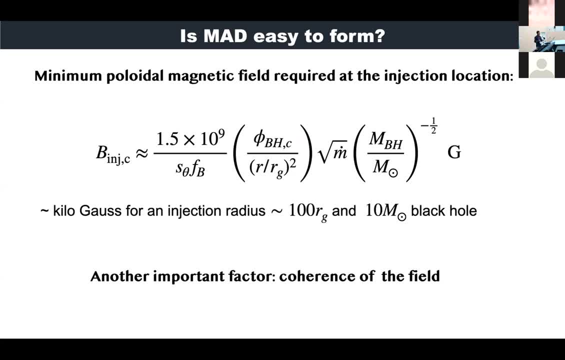 So this is the formula we come up with And we found that if we inject the magnetic field loops around 100 solar channel radius- sorry, gravitational radius- for a 10 solar mass black hole, which is typical mass for the XK binaries, then kilohertz field is fine. 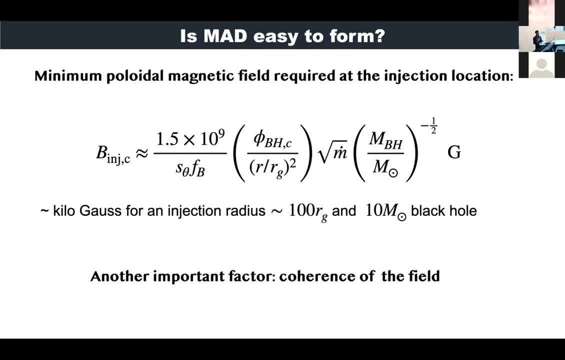 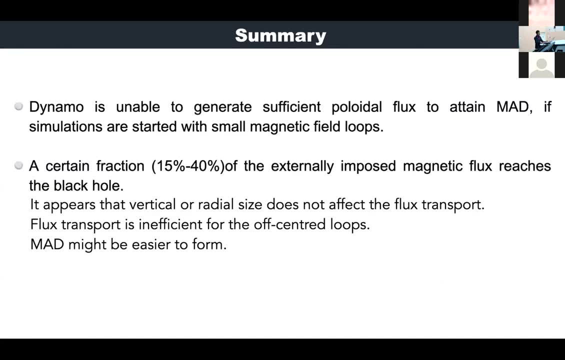 That will reach- That will eventually create the map, Although we are silent about our own feature. this is the- This is the coherence of the field That is also required. So here is the summary of my talk. So we found that dynamo is probably not efficient enough. 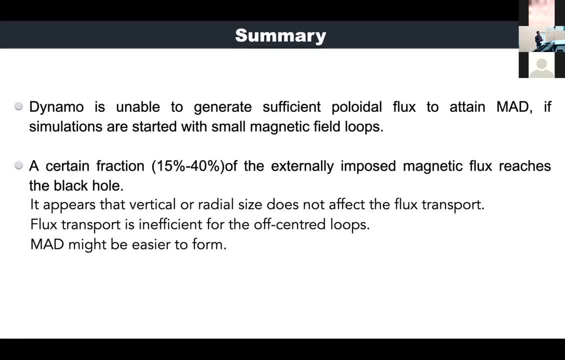 in the dry-up itself to generate the strong enough torridal flux in order to produce jets. If we talk about the external magnetic flux, a certain fraction of the external magnetic flux is reaching the black hole, which is, I would say, a moderate amount. 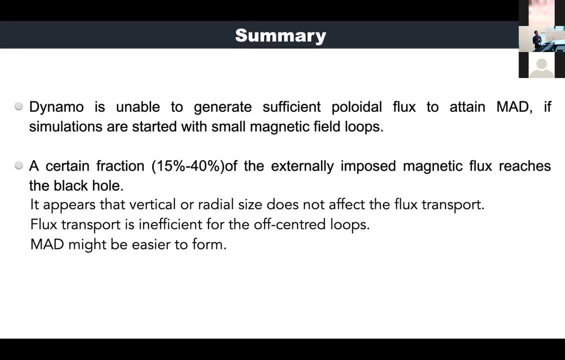 And we found that in the parameter space we have scanned for the vertical- the flux doesn't really matter. And we've also found that off-centered loops are basically show very poor efficiency in transporting the magnetic field And the final conclusion would be probably: 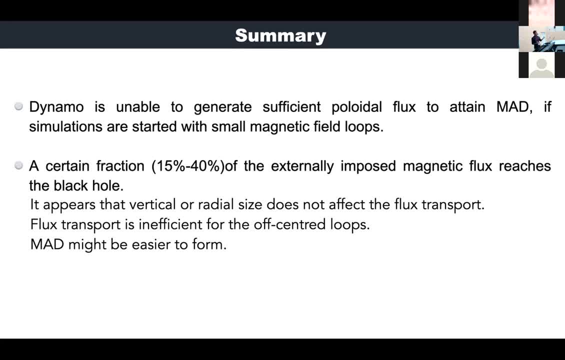 that it would be easier to form, provided there is something that our experiment we have done in the parameter space we have scanned is maintained in the nature. Yeah, that's all I wanted to say. Thank you, Prasoon. Questions from the audience. 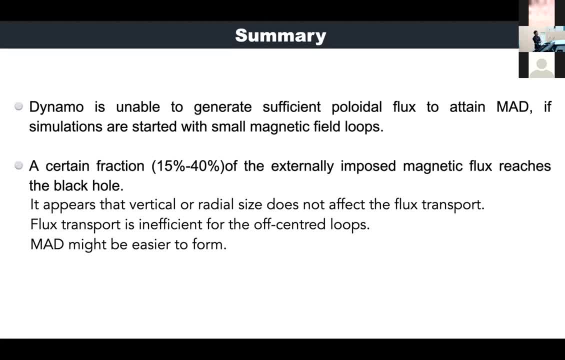 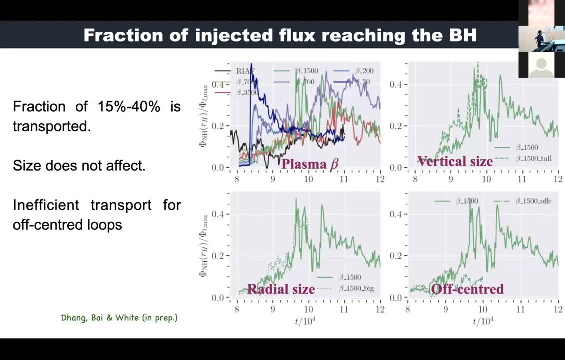 From the people present in the lecture room: Prasoon: good talk. Did you check- I mean sort of estimated- the resistivity, although I know it's an ideal image because you see, physically speaking, the magnetic field cannot enter the black hole. 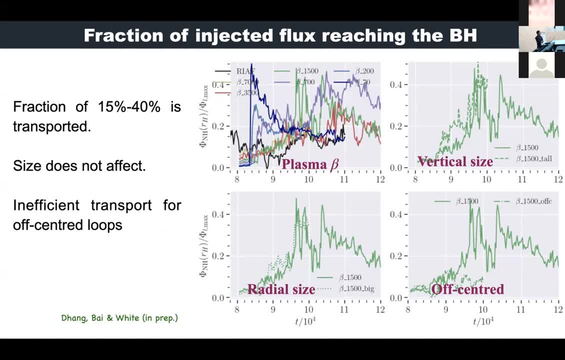 Yes, So therefore, what can it do physically? It can generate, because the region is very compact near the black hole, it should generate a lot of resistivity. Yes, OK. So if you can, you sort of measure, I mean? 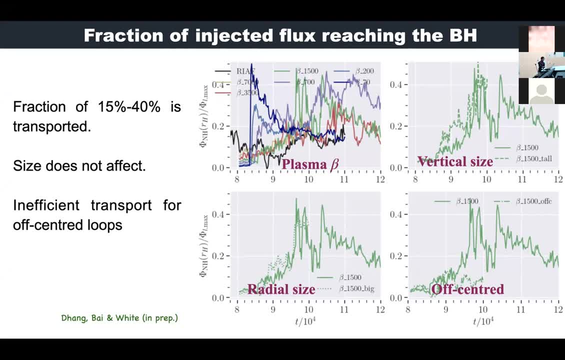 post-theory, after the simulation is done, instead of plotting the plasma meters and all. it is better if you can measure the resistivity, Then there will be indication that that magnetic field is actually decaying near the horizon. Yeah, so that's a good question. 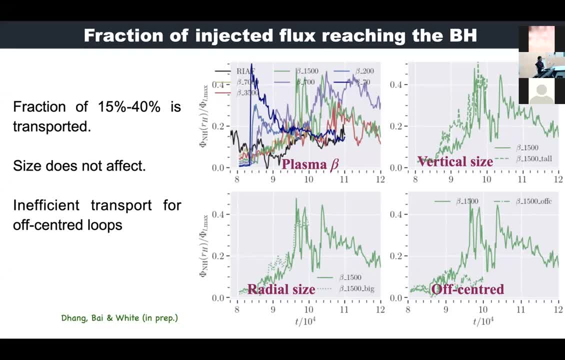 The reason is that we have not done it for GM-MHD, but we have done it for our earlier case in MHD simulations. Yeah, OK, So the problem is that we have to do control volume analysis of the whole domain, which is kind of very expensive. 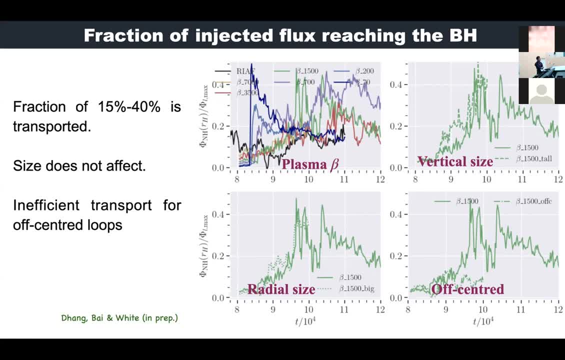 even in post-resisting, And people have found that the resolution we have used, the effective Reynolds number would be around 5,000, which is probably one of the highest achieved in global simulations of emission flows. And here all the resistivities comes from the grids. 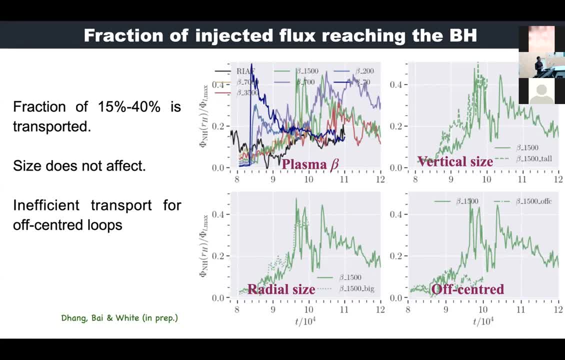 as we are not putting any explicit resistivity, But there is another term, something called turbulent resistivity as well, which is much more, much more dominant over the explicit resistivity. So we have computed it in Shearing-Box simulations and we found order of magnitude larger. 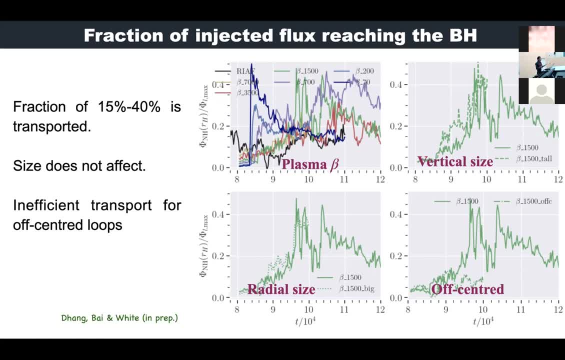 than the grid resistivity. So I think we are fine, or we think as a community we are fine, But again, as we increase the resolution, ideally we should reach around 10 to the power, 18 to the power, 17 Reynolds number which is, I think, kind of infeasible. 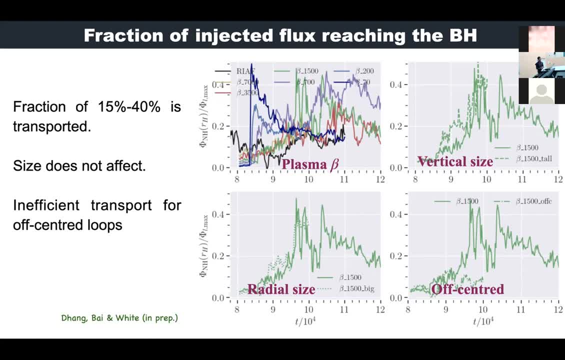 unless something big comes up. Any other questions from the auditorium? No, there is no question from, So has a question from the Zoom? Hi, Hi, Thank you, Prasoon, can you hear me well? Yeah, yeah, I can hear you well. 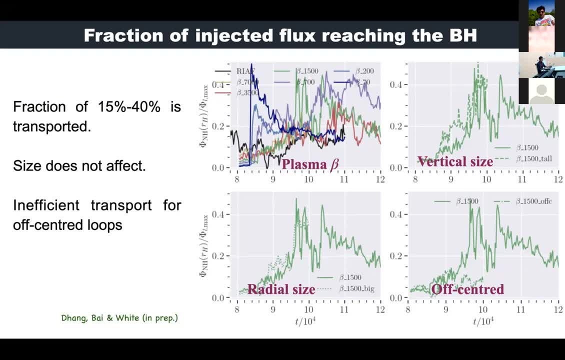 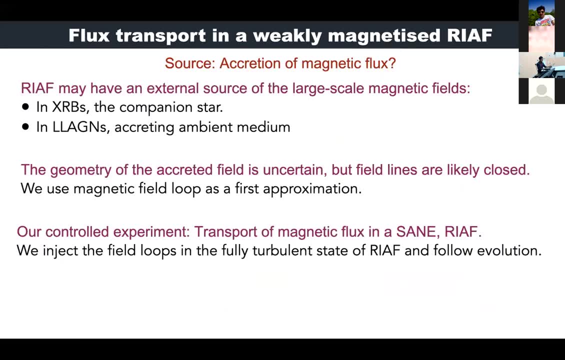 Yeah, Prasoon, you mentioned about the thing of MRI, in order to transport the matter in your re-ops, So usually in GRMAG simulations, people. actually, you know they have a lot of time. Yeah, So we compute something called as a quality factor. 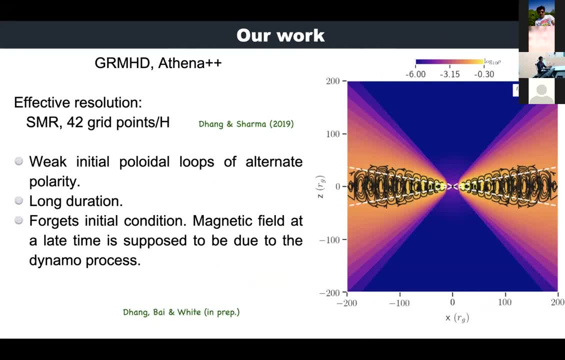 Yes, yes. So have you estimated that and whether that estimate remains MRI unstable throughout the simulation? Yes, So generally it is told that empirically if the two quality factors the multiplication of Q3 and Q5, if their multiplication is above 200,, 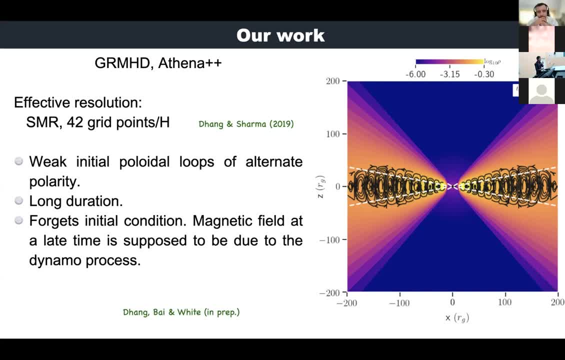 we say that, OK, it is resolved. So for our simulation it is around 250 throughout the runtime. And also I think the better quality factor would be the magnetic tilt angle, And people have found that it is above 10 degree. 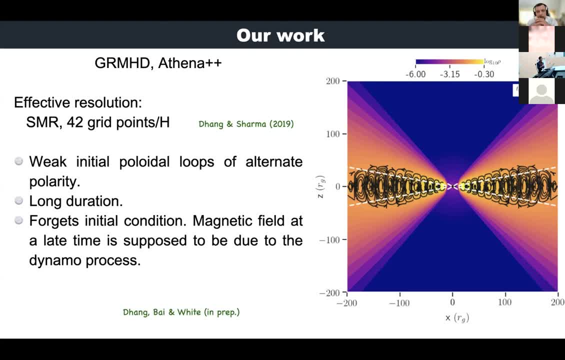 then simulation is well-converged And for our GRMAG simulation we found it to be around 30 degree, And for our MEG simulation it was much more better, around 40 degree. OK, And this was also true when you included the magnetic flux. 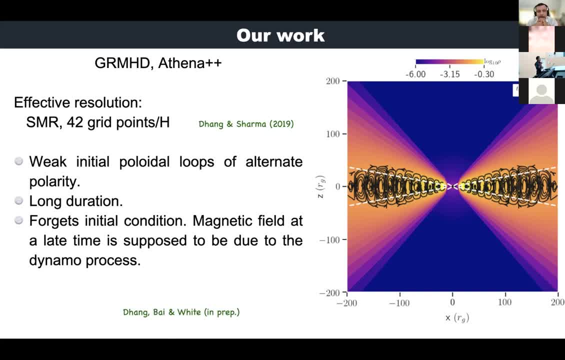 When you injected the magnetic flux, the quality factor, It will increase because we are adding the magnetic flux on top of the existing field, So it will enhance the quality factor. OK, Thank you. Any other questions from the online participants? I have one. 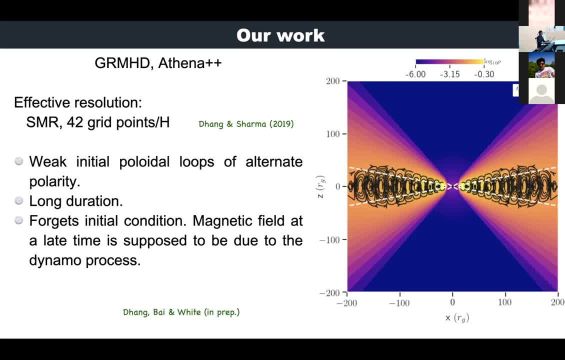 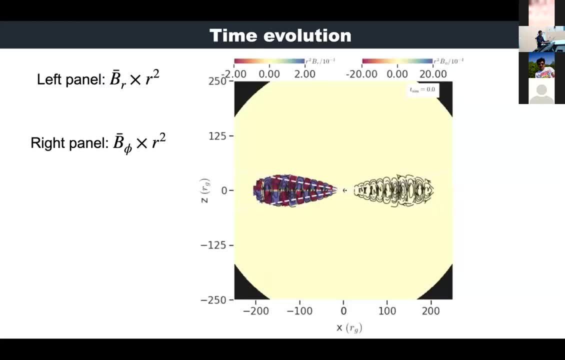 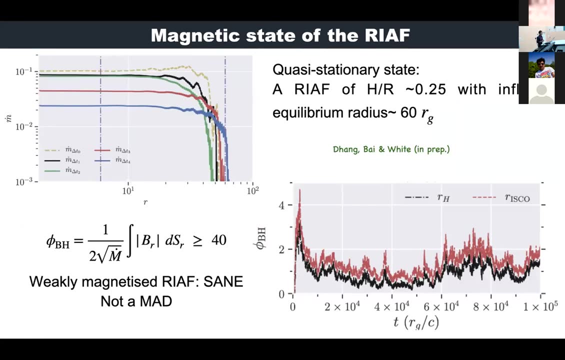 OK, Go ahead. So when you say that there is a need of high magnetic flux, so how are you going to call it high? Because there's the? Yes sir, This is the people looked at. Yeah, So the observation are being more refined. 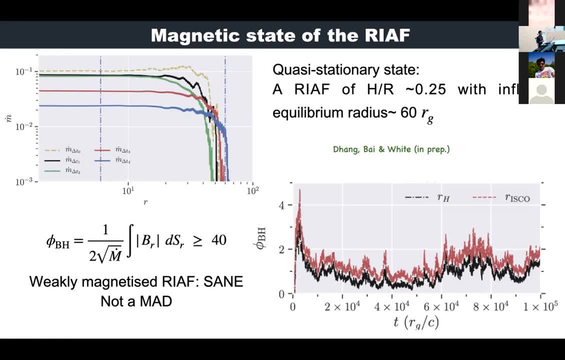 So initially, like for MIT-7, it was supposed to be somewhere around 160, 180.. And then the number keeps on coming down. based on this Like, we sent this polarization image to suggest that it should be somewhere around 30 or 40.. 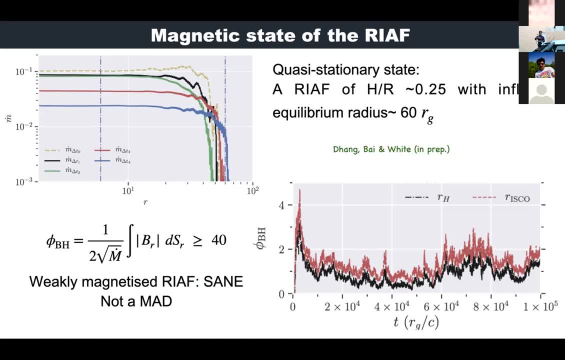 Some 30 Gauss, 30 Gauss, 30 Gauss, Yeah, 30 Gauss. See, this is a dimensionless number, So it is normalized with the mass efficient rate. So it should not change. OK, OK, So that. 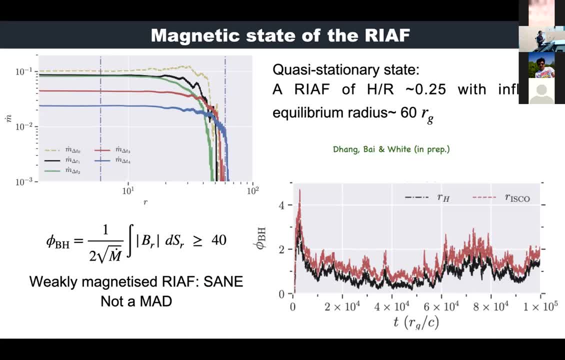 OK, So that is the. It is irrespective of the mass of the black hole, Because essentially, for AGS the mass efficient rate will be low, But for x-ray binaries it will be higher. Oh sorry, Hold up. 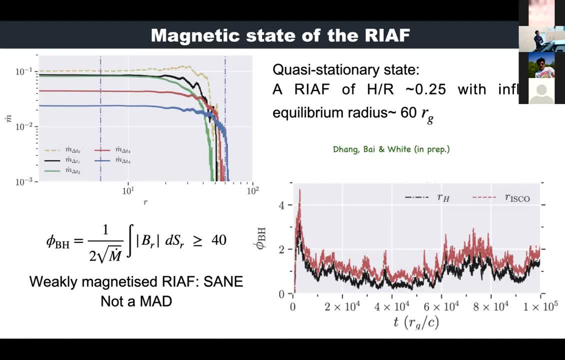 Hold up, Hold up. But shouldn't there be an interplay between this magnetic energy density and the thermal energy density, so which dominates? Like, let's say, the matter is too hot, then it doesn't care about the magnetic, It depends on the process you are looking at. 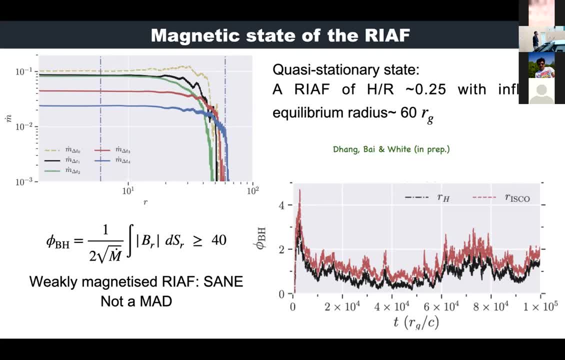 If you are looking at probably 0.8, flux will dominate over the radiation, But so far I think more consensus is from numerical experiment. is that probably dominates over all other processes? At least we have one. But again, Christian is working on something. 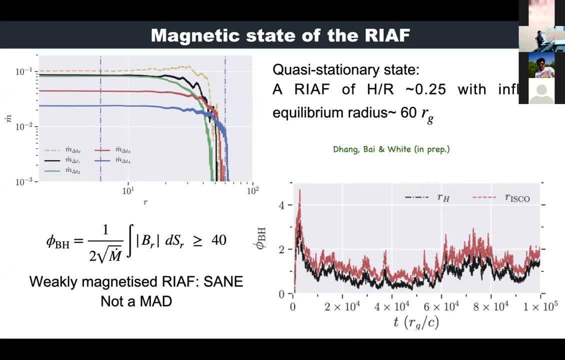 where they found also works. Yeah, So like the from the initial that it is too low. Like not, No, no, It's not. Yeah, Yeah, The electric is embedded in the disk itself, But the mass equation rate is low initially. 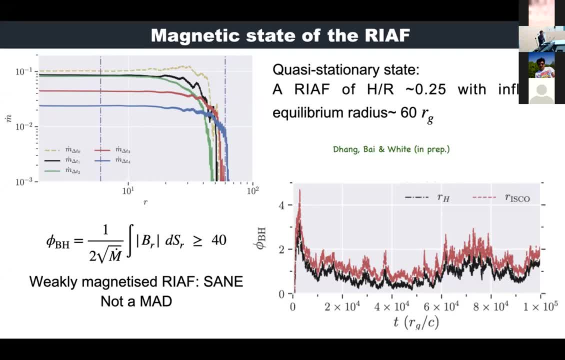 In. That's what I'm asking again, Like you don't have like very high equation rate. See, as I have heard from people who are doing jet simulations, as long as you have a strong magnetic corridor flux, nothing can kill the jet. 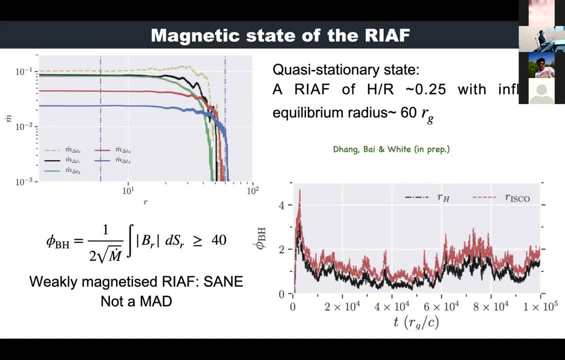 No, a lot of matters will kill. OK, If you can generate a lot of electricity, That's our end- use paper. They are saying that it will kill. You will generate electricity anyway. So that apart, if you have a lot of matter. 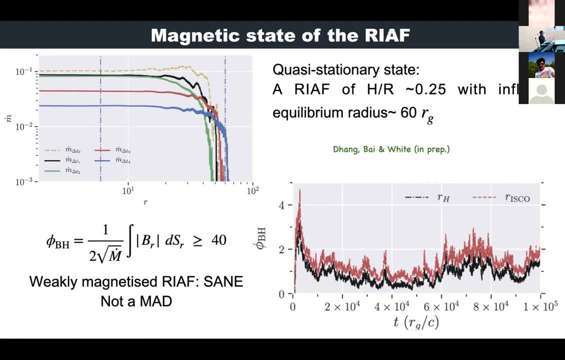 is not supposed to, Because if you look at original paper, it is basically vacuum. Yes, exactly. And then you give a little bit of particles, the spheres, just to kickstart the thing. Oh, by the way, when I'm saying the matter, 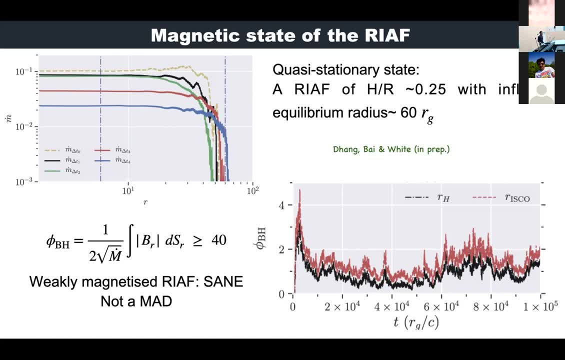 I'm talking about the disk, not the funnels. Funnels are generally almost vacuum. Like you can compare the density of the disk and funnel, it is order of magnitude less. For example, here if it is 10 to the power 6,. 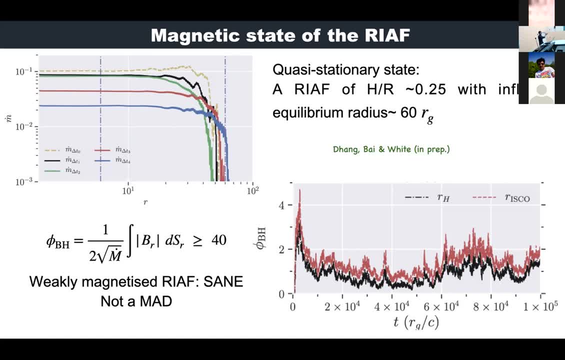 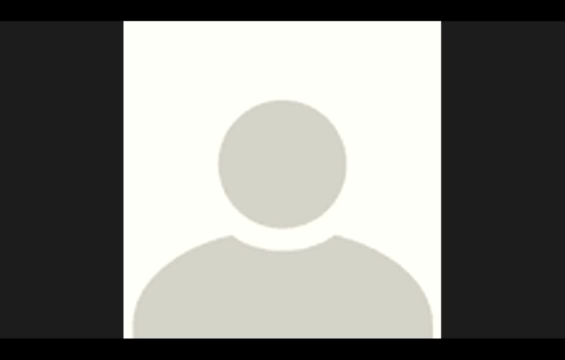 let's say it will be 1 here, So we always find a along the poles. So that is the reason. OK, thank you, Prasoon. Yeah, Thank you. We'll move on to the next talk now. The next talk is by Rajdeep Agrawal, who. 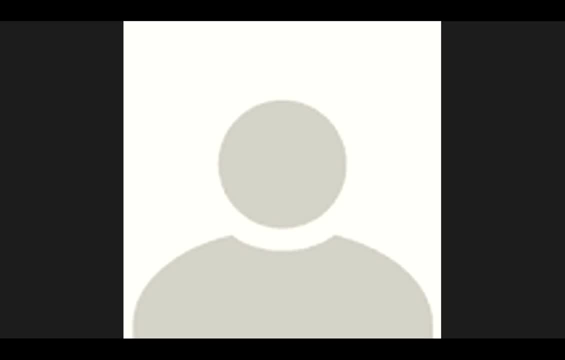 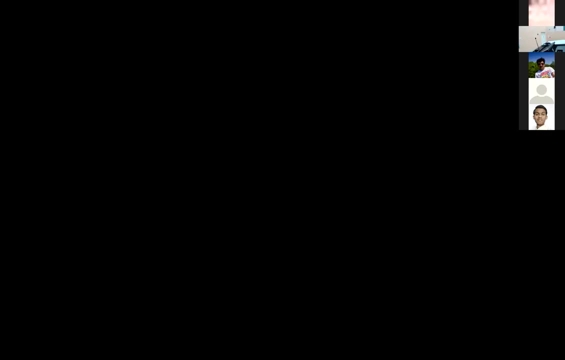 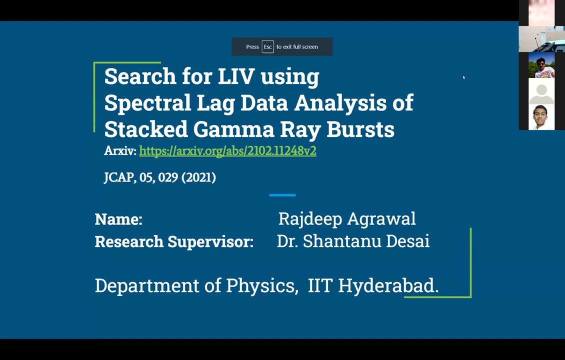 will be speaking about search for Lorentz invariance violation from stacked gamma-ray burst spectrolabs. So, Rajdeep, I guess you are giving the talk online, So please share your screen. Yeah, yeah, thank you. Yeah, so can I start? 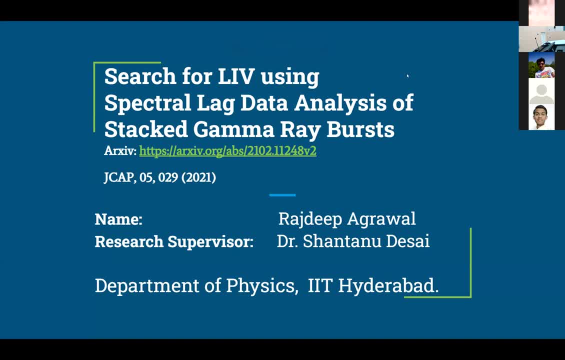 Yeah, please start. So good afternoon everyone. My name is Rajdeep Agrawal and I'm a student. I'm a final year undergraduate student at IIT Hyderabad, OK, And I'm a professor at the Department of Physics. 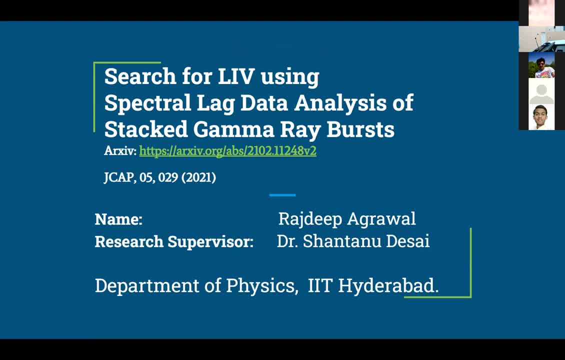 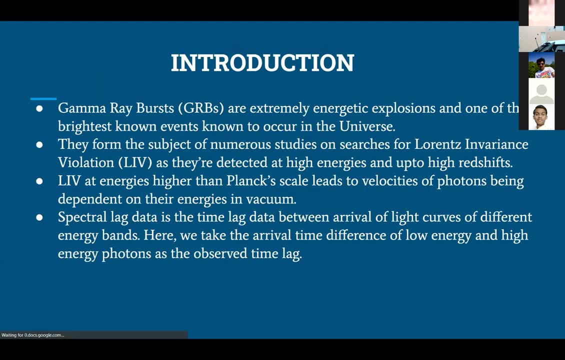 So the topic of our research and presentation today is the search for Lorentz invariance variation using the stacked spectrolab data of gamma-ray bursts. So brief introduction. as most of us might know, gamma-ray bursts are extremely energetic and some 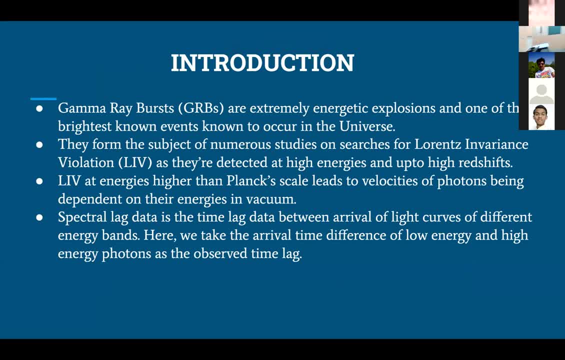 of the brightest and most luminous known events to occur in the universe And in recent times, gamma-ray bursts have proved to be a very useful probe for Lorentz invariance variation due to the energies and redshifts that are detected. 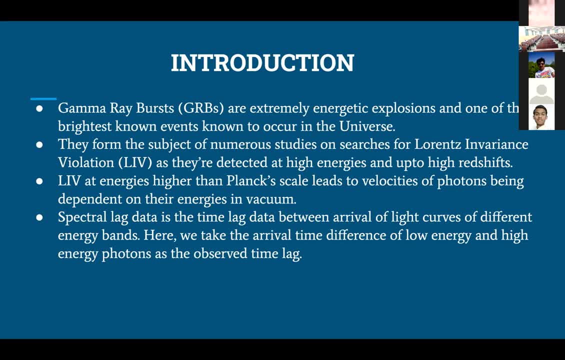 So typically, the quantum gravity energy scale at which these gamma-ray bursts are detected are almost close to the Planck energy scale at which LIV is supposed to set in, And the spectrolab data that we have used for analyzing these gamma-ray bursts is essentially the time-lapse data. 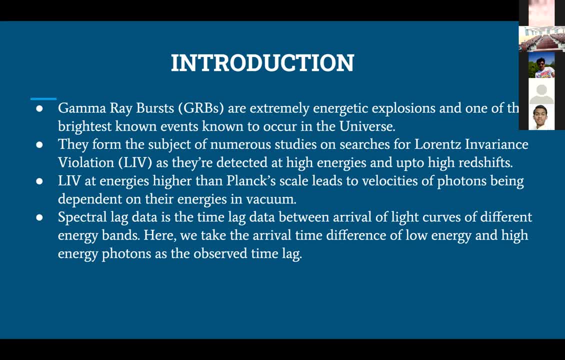 between the arrival of the low-energy and high-energy photons of these gamma-ray bursts, since one of the major consequences of LIV is that the velocities of photons will now be a function of their energies in vacuum And no longer constant as the speed of light. 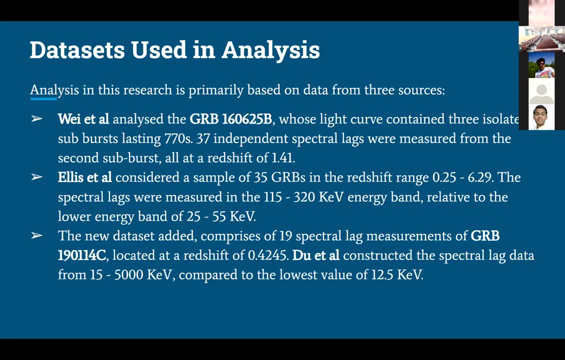 So a small summary of the data sets that we have used for our analysis. First we had the Wey et al data of GRB160625b, which comprised of three isolated subbursts, And from the second subburst they were able to extract 37 independent spectrolab. 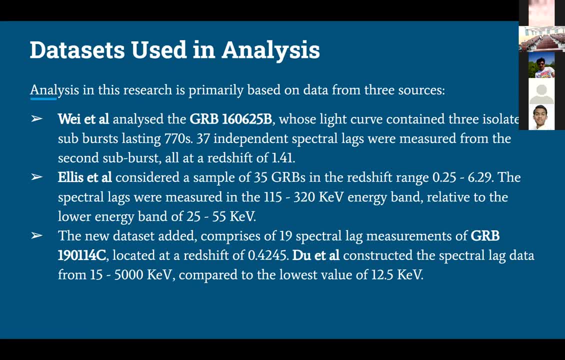 measurements all at a common redshift of 1.41.. And this was one early research where they had claimed that sufficient evidence for spectrolab overturning, that is, LIV observation, was present. But that was later almost refuted in further statistical analysis in another 2017 paper. 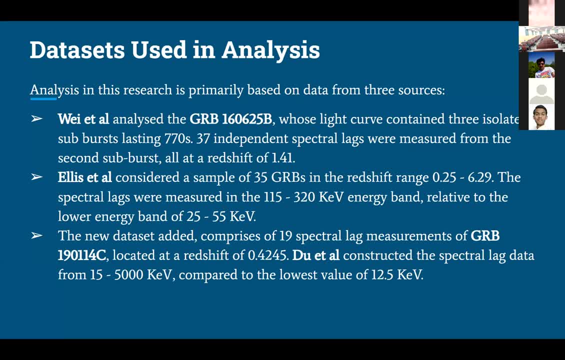 The second data set is Ellis et al, who took a slightly more diverse number of GRBs in a redshift range as specified here, And the upper energy band of these GRBs was around 115 to 320 keV and a lower energy band of 25 to 55. 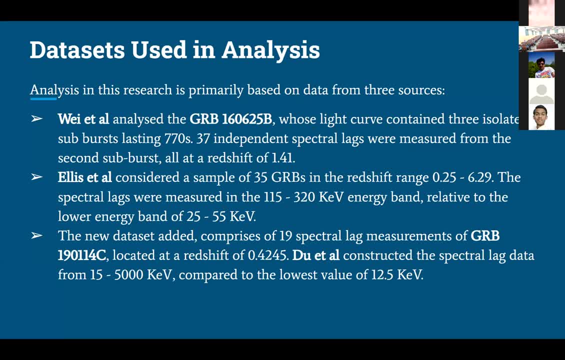 keV And the final data set, A slightly peculiar one. This one was from the Du et al paper, Again comprising of a single gamma burst of a constant redshift of 0.4 to 45. And in that paper they used opposite sign. 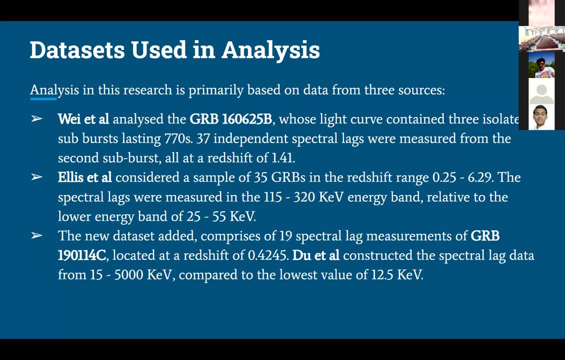 for the intrinsic parameters, intrinsic black parameters, which we will incorporate in our research as well, And the higher energy band, if you see, has a very higher upper limit, which is around 5,000 keV, which is quite high as compared. 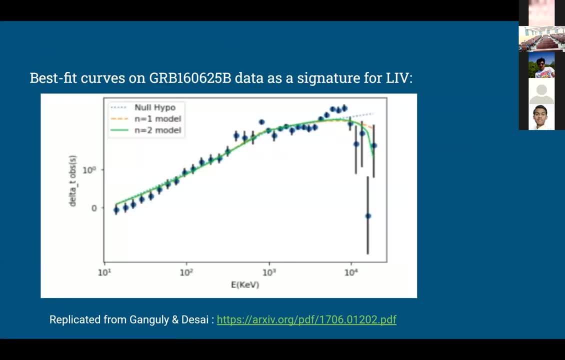 to the other data sets that we have used. This was the result of a preliminary analysis on only the Wei et al data set, where we fit the three model hypothesis functions, which is the null hypothesis, which includes only the intrinsic time lag, And the n equal to 1 and 2, which is the linear and quadratic. 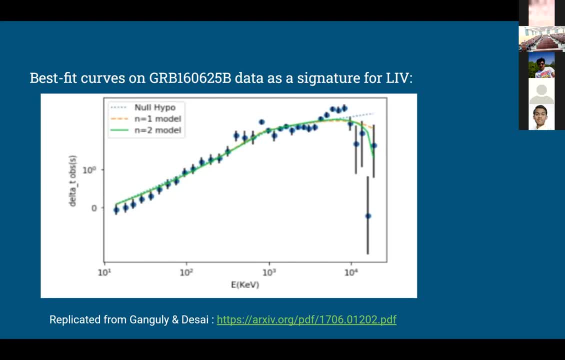 LIV models were fit on the spectral lag data provided in that paper And, as we can see, for higher energies of observation of these gamma rebursts. we observed that again, the data in the LIV-based models show that tail towards the end, which 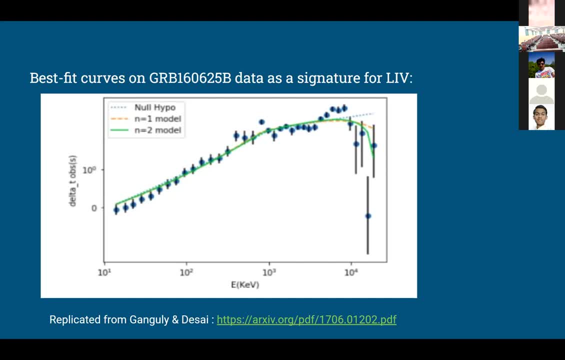 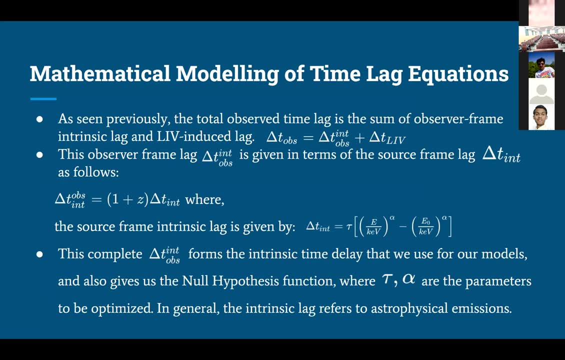 proves to be a better fit on these higher energy scales, whereas the null hypothesis almost diverges from those points. So a brief thing about the mathematical modeling of these time lag equations. So the total observed lag between the low energy and high energy photons of gamma reburst. 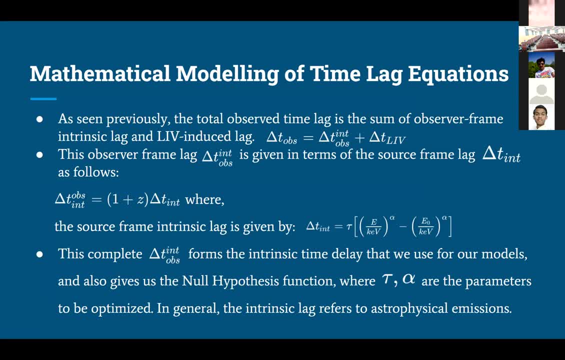 is taken to be a combination of the intrinsic astrophysical emission lag and the LIV-induced lag. So the intrinsic lag is calculated in the observer frame by multiplying with the cosmological redshift to the original source frame time lag. And this intrinsic lag itself has two unknown parameters. 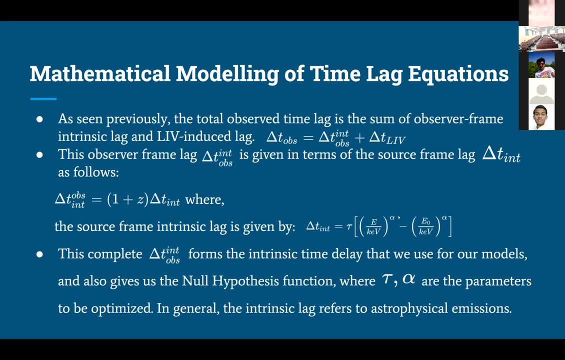 which have to be optimized, tau and alpha, along with E0, which we assume to be the medium of the lower energy bit of the gamma reburst, And E is the observed energy at which the emission was observed, And so the second term which we have. 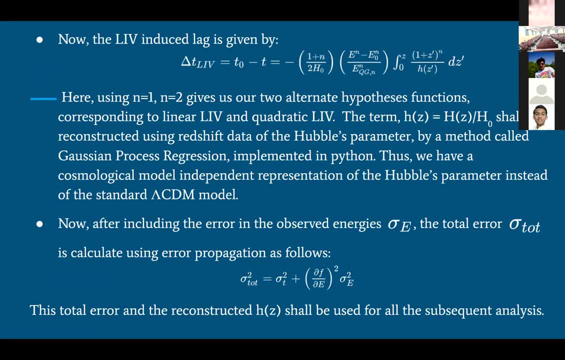 is the LIV-induced time lag, which is part of the n, equal to 1 and 2 models. So this comprises of: so that is what the n represents here, And we have H0, which is the Hubble's parameter. 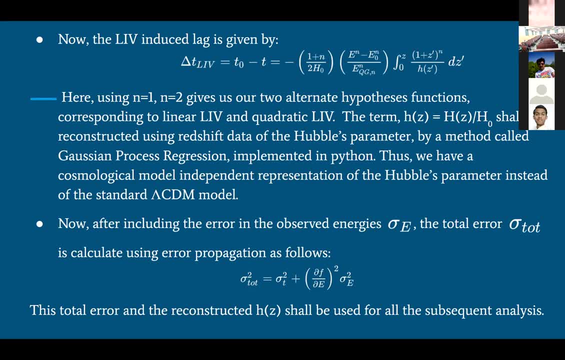 And in the integral, if you see, we have a term H of z prime, which is the redshift-dependent Hubble's parameter, the reduced quantity, And that in a cosmological model-dependent sense it would depend upon the redshift. in a basic formula, 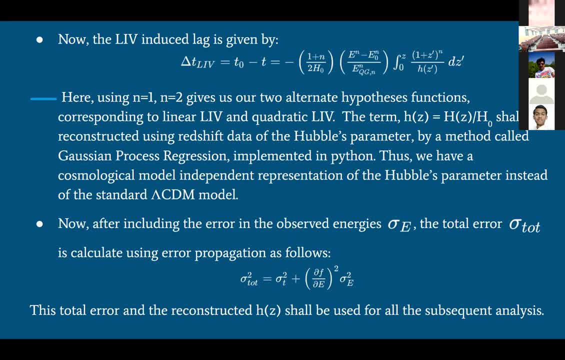 that we are aware of, But since we're dealing with energies close to the Planck scale, where the cosmological model may not be applicable anymore. so we have tried to reconsider And we have constructed this Hubble's constant as a non-parametric function of the redshift. 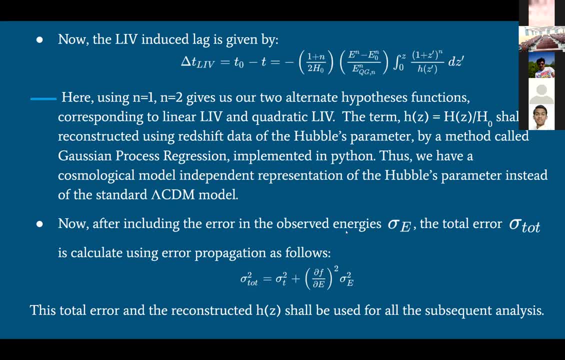 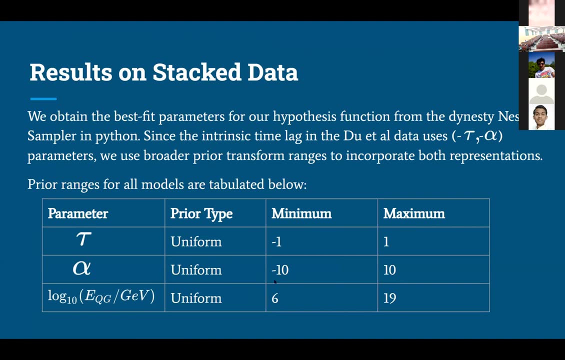 using Gaussian process in Python, thereby eliminating the dependency on the standard lambda CDM model, And we also had the errors observed in the observed energy, as well as the time lag which was present in the spectral lag data. So these are the results. 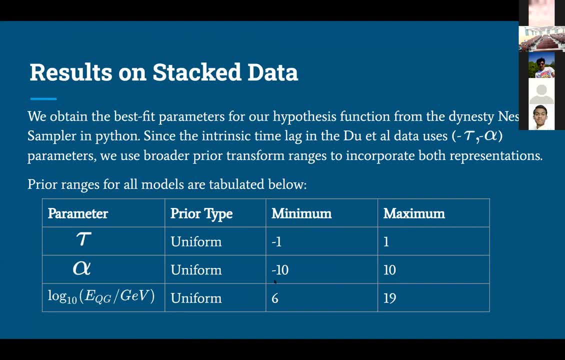 This is the prior transform ranges that we had used for our nested sampler in Python to compute the best fit parameters and the Bayesian evidence for the different models. So since the last data set do et al, they had negative signs on the opposite signs on the intrinsic lag parameters. we 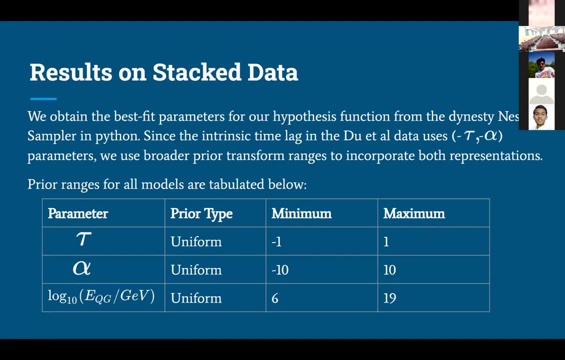 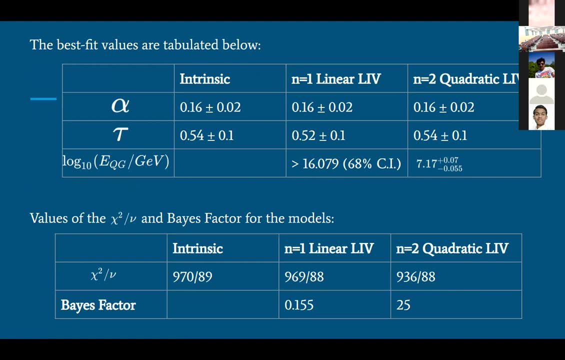 had to expand the scope of the prior transform ranges for the tau and alpha, which are the intrinsic parameters, in order to incorporate that, And the best fit values obtained from the sampler are listed here. So in cases where we see an empty cell, 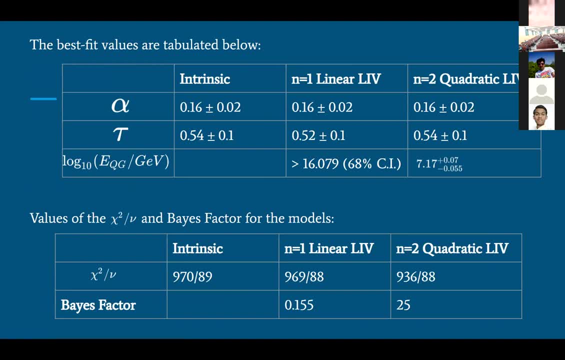 it's because the close bounds on those values were not obtained from the sampler. And if we observe again for the LIV energy values, the EQG, we see that it's close to 10 par 16 or 10 par 7 in this case. 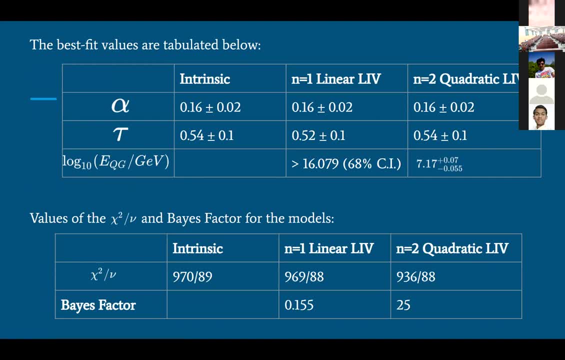 which is which kind of approaches for high energy gamma-ribbers that actually approaches the Planck's energy scale of 10 par, 19 GV in some cases, And in the table below we see the parameters to estimate the goodness of fit and a model comparison. 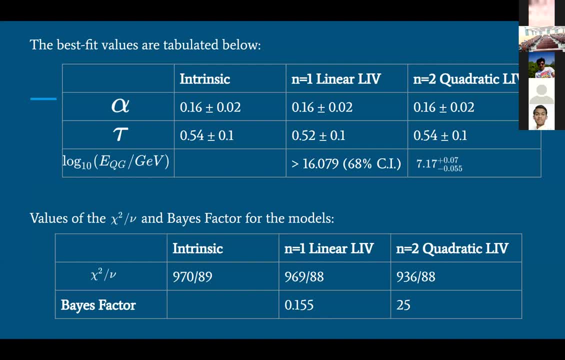 So the reduced chi-square is empirically supposed to be close to 1 to indicate good fit of the model. So in this case it's close to 10 or 11 in almost all the cases, which does not signify a very good fit. 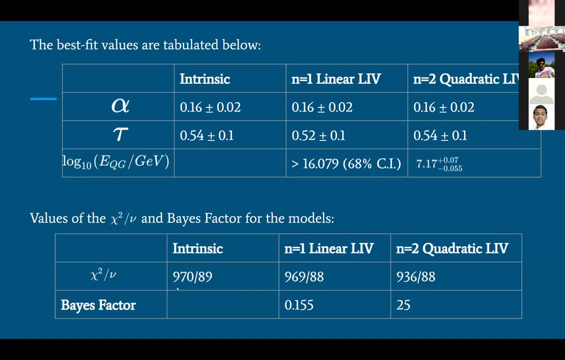 And the base factor for the LIV models, if we see, is almost very negligible for the linear model, which almost gives no evidence in its favor, whereas a quadratic model with LIV of 25 still has a strong evidence in its favor. 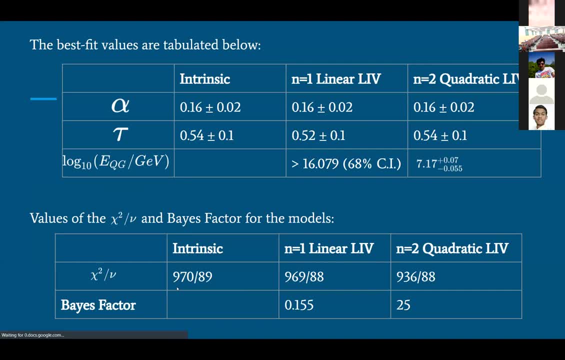 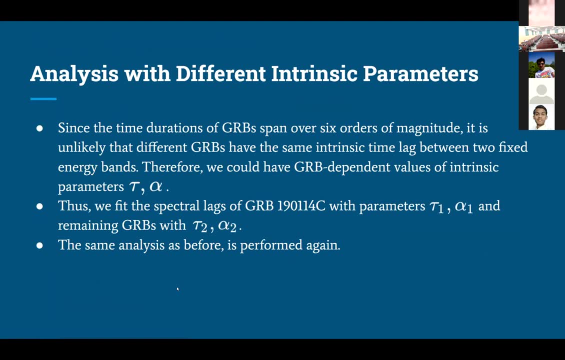 though it is not decisive enough to overturn the null hypothesis Now because they are. So this was the analysis done with common intrinsic lag parameters tau and alpha, throughout the entire set of gamma-ribbers that we had. But because the final data set in our analysis uses basically: 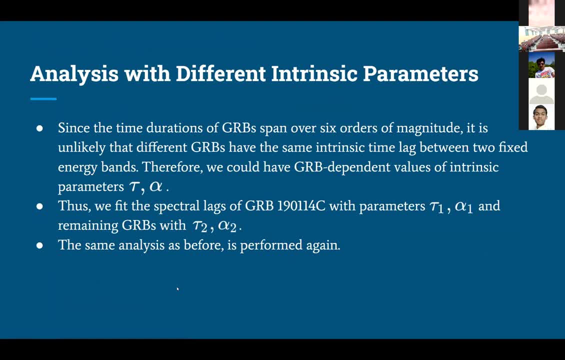 has gamma-ribbers spanning over larger orders of magnitude, as well as detected over a much higher upper energy band, along with opposite signs for the intrinsic parameters. it was considered prudent to try and analyze that data set with separate intrinsic parameters, tau and alpha. 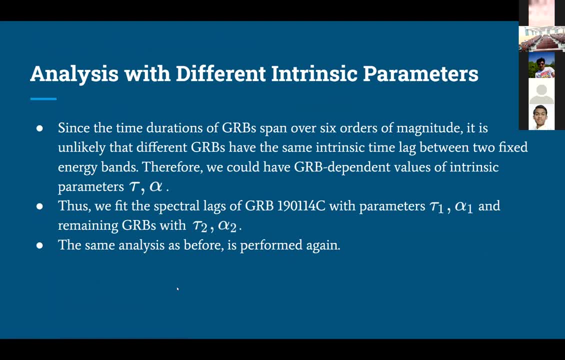 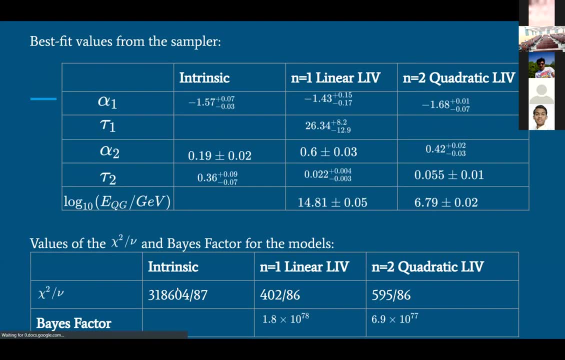 So to that end we have. We have chosen distinct- what do you say? GRB-dependent- intrinsic parameters for the analysis and performed the same operations again. So again from the sampler we obtain the best fit values for the different parameters. 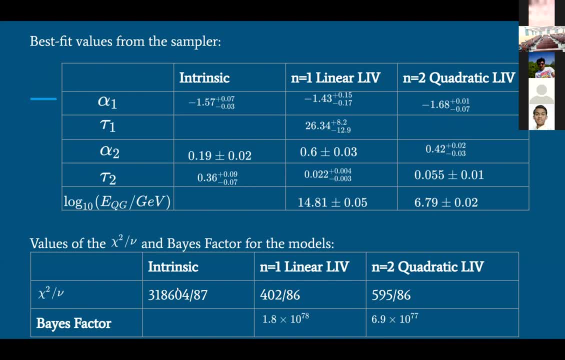 Again, places where it is empty is because we could not get a close bound on those parameters from the sampler. And again, if you observe the LIV-based energies for the linear and quadratic models again approach like 10 power 14 or 10 power 6.. 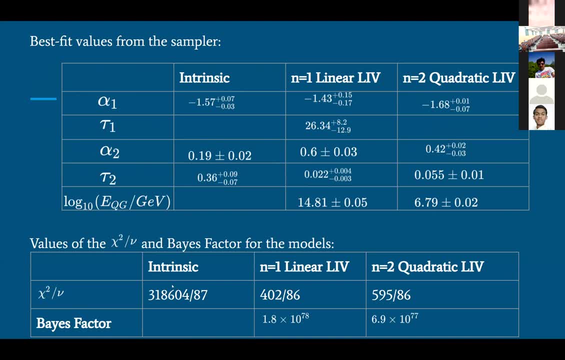 So again, kind of moving towards the Planck scale of 10 power 19 GV. And for the goodness of fit of the models, we see that the reduced chi-square value is much higher for the intrinsic model as compared to the LIV models, indicating that the LIV models are 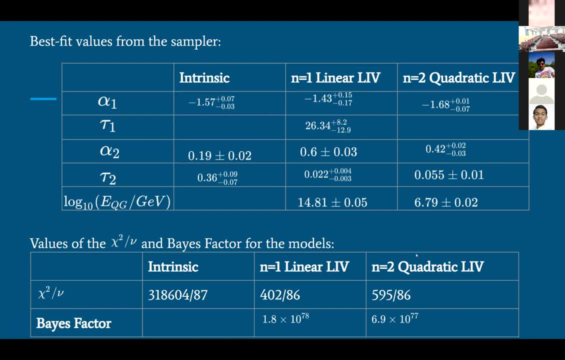 a slightly better fit And even comparing with the previous analysis, the reduced chi-square for the LIV models is between 4 to 7, which is lower than the previous values of 10 to 11 almost. And the major difference here is in the base factor, which was 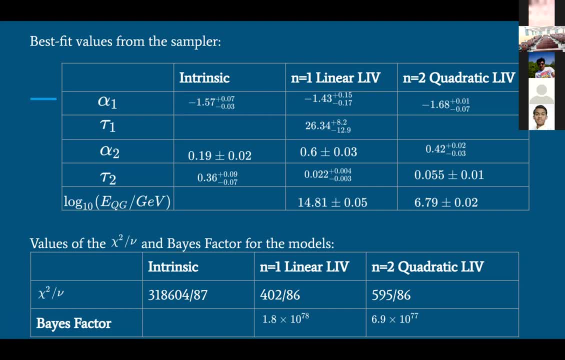 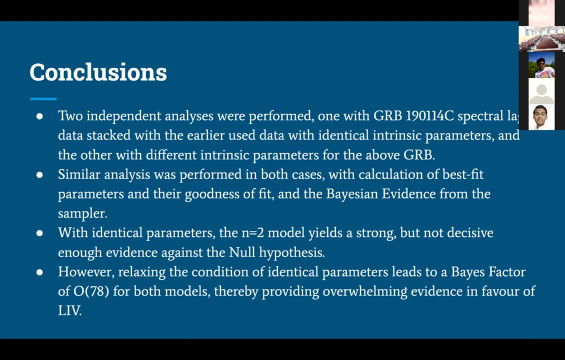 again quite insignificant previously. It is now almost overwhelmingly large in this case, thereby presenting substantial evidence in favor of LIV with this analysis of more GRB-dependent intrinsic parameters. So the final conclusions of this research is by performing two independent analysis on stacked gamma. 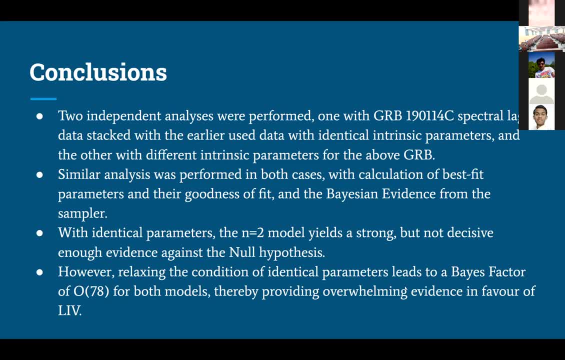 ray burst data from three sources. we have first modeled them with common intrinsic parameters, in which the quadratic LIV model gave us some strong evidence for LIV, but it wasn't substantial enough. And then, when we used the GRB-dependent intrinsic parameters to single out the last set of GRBs, 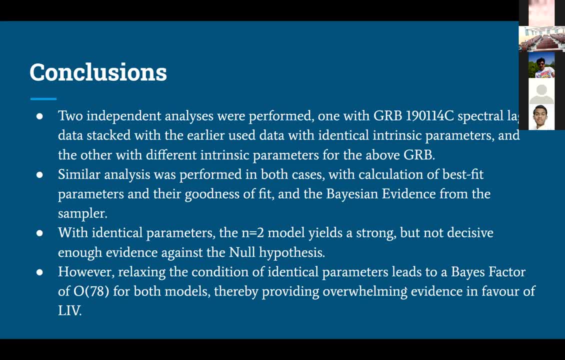 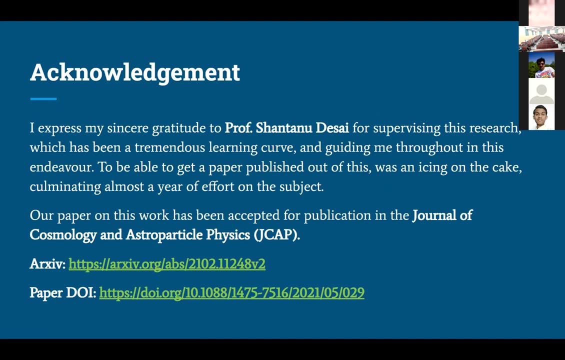 then we got substantial evidence in favor of both the LIV models that we had used And the analysis performed was absolutely identical in both the cases. So that's it about the presentation And, just a note of thanks, My supervisor, who is also part of this conference. 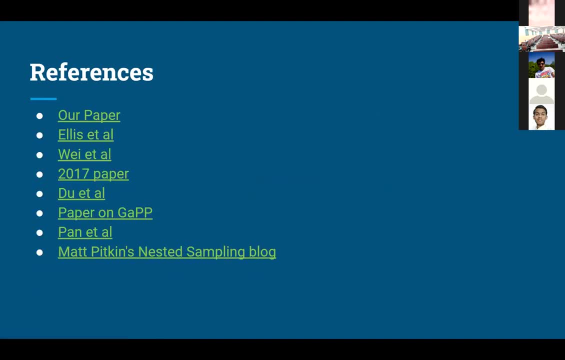 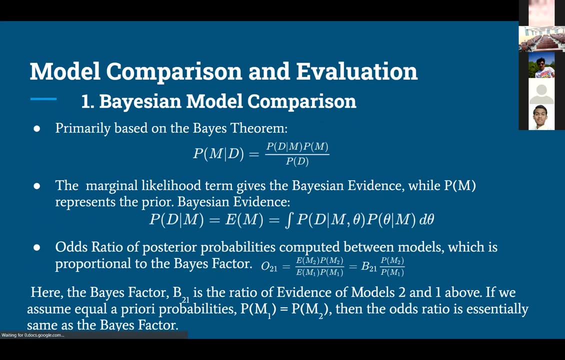 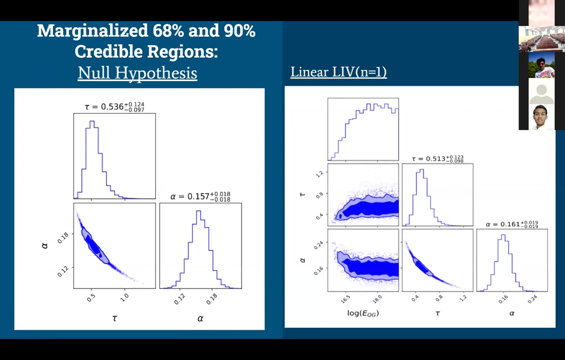 And this research was done in collaboration with him. And these are the references, And this is just the appendix, about various model comparison techniques: the Bayesian model comparison and estimation of chi-square from the log likelihood. These are the Bayesian credible regions, again obtained from the sampler. 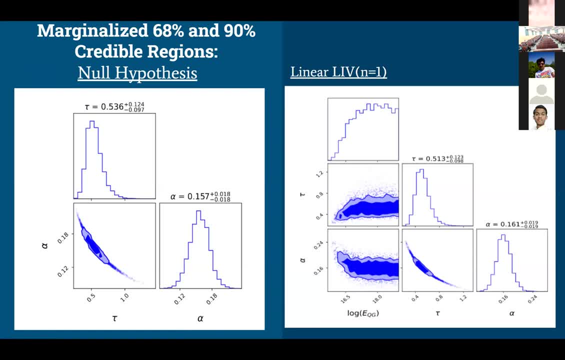 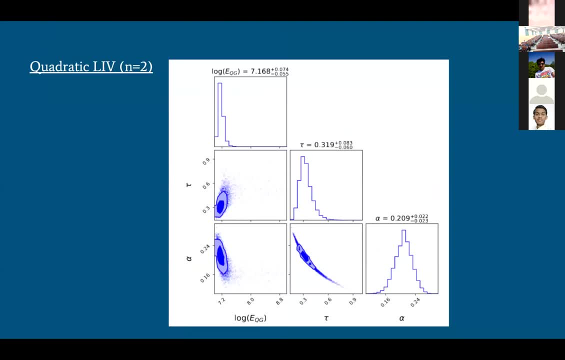 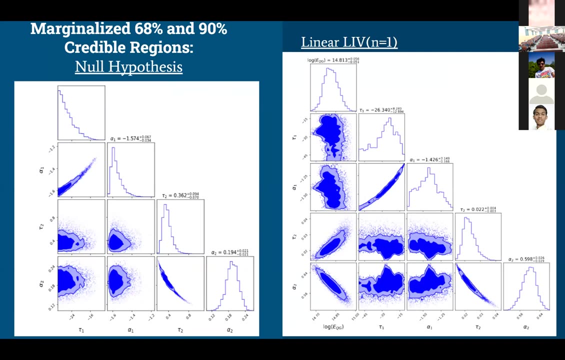 These are for the common intrinsic parameter case for the three different models: The LIV-independent model, the linear LIV model and the quadratic model, And these are the same reasons for the case with GRB-dependent intrinsic parameters. As you can see, we have different intrinsic parameters. 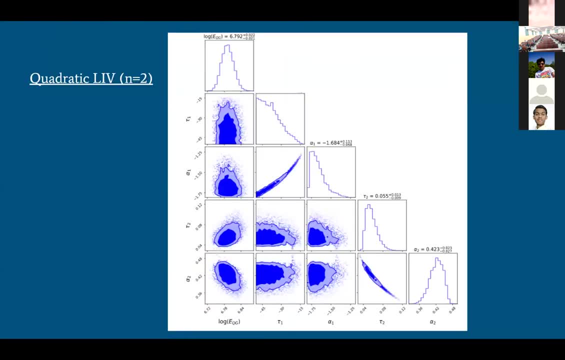 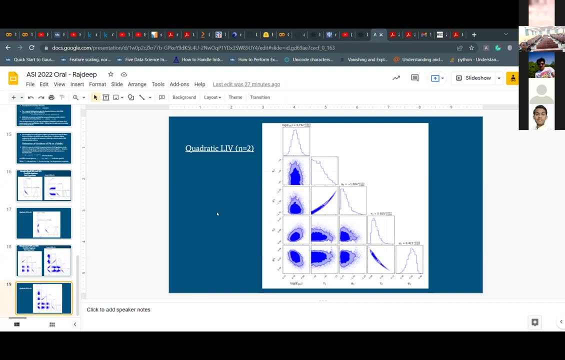 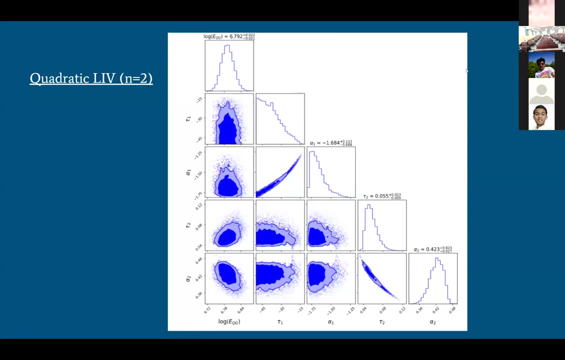 here. So again for the three different models. So yeah, that's the end, Thank you. Thank you, Rajithi. Any questions from the audience? No, ma'am, There is no question from offline audience. OK, From online participants. is there any question? 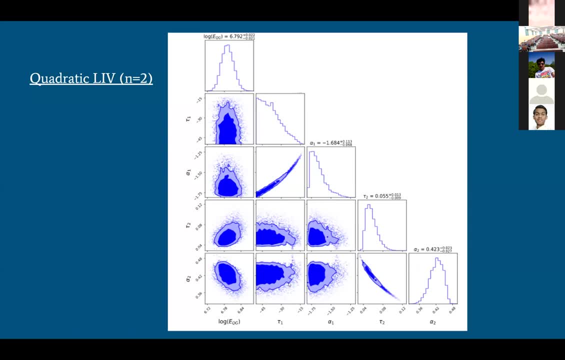 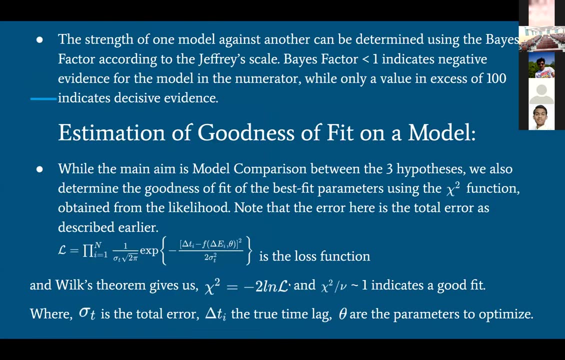 OK, Rajithi, I have one question. So here you showed the case of 1901-14C. I may have missed this point in your talk, But did you also? how many other GRBs did you try this with? 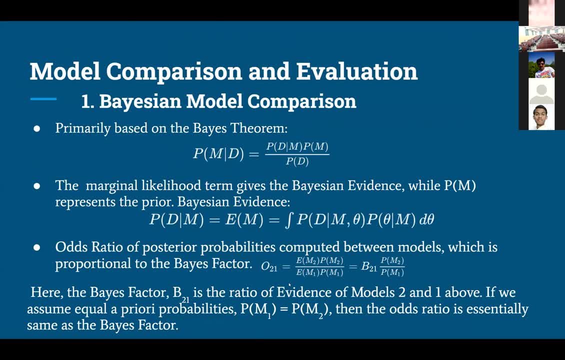 See, we have three independent papers from where we collated The GRB sources. So in the second paper we had a whole lot of GRBs. The 1901-14C was one of the GRBs taken from the third paper. 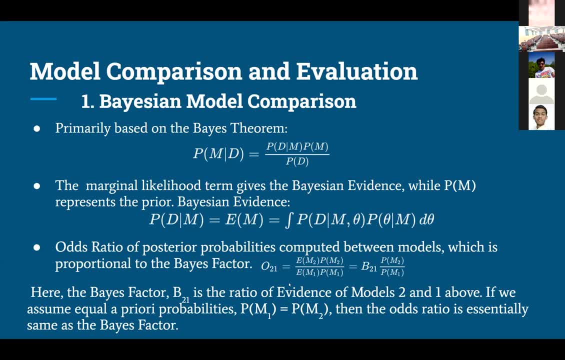 So we have a whole lot of different GRBs, OK, and what was the selection criteria for choosing only those GRBs on which you run this analysis? That was primarily based on the recent research which was done on similar kind of GRBs, So whatever was suitable to what we wanted to do. 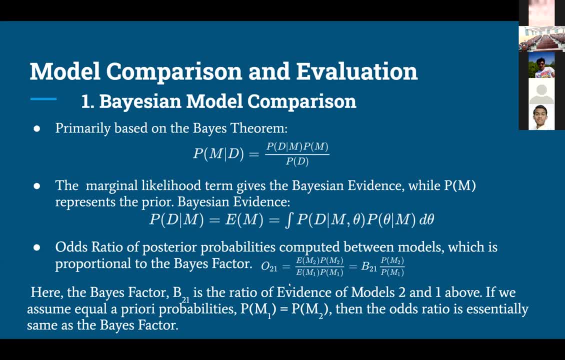 Our aim was to basically develop some sort of unified model where we can stack these GRBs and check if there is some evidence of LIV. So, whatever individual works were done in this regard, that is what we stacked eventually, And this comprises of both long and short bursts. 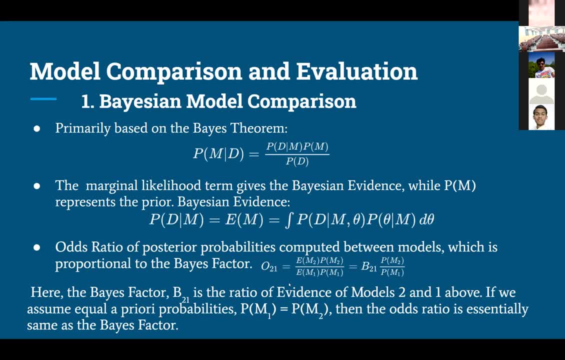 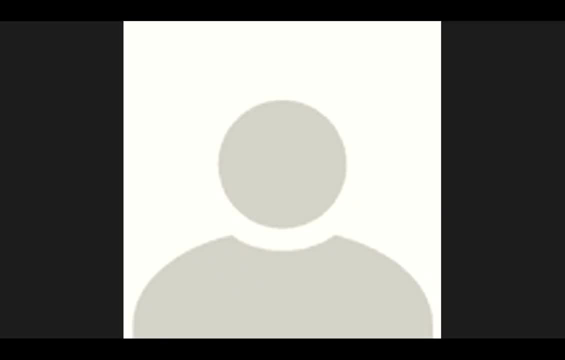 Yes, You have not made any distinction between them. Yeah, we have not stated that explicitly. OK, thank you. OK, if there are no other questions, let us thank Rajdeep for this nice talk, Thank you. Thank you, It's been a nice talk. 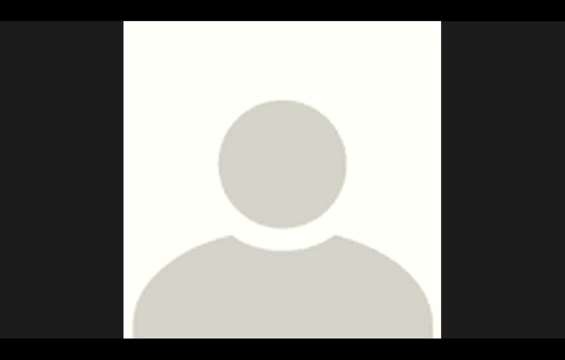 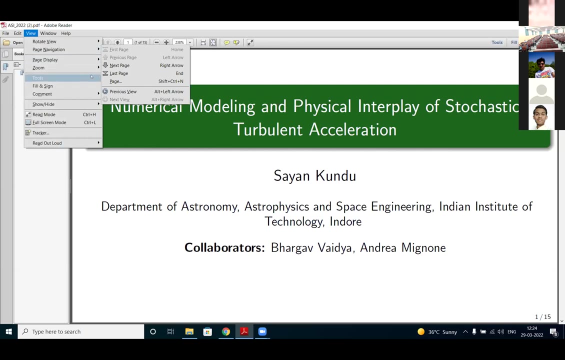 The next talk is by Shayan Kundu, And he'll be speaking about numerical modeling and physical interplay of stochastic turbulent acceleration. So, Shayan, you may please go ahead and share your screen. Hello, Am I audible? Yes, you're audible. 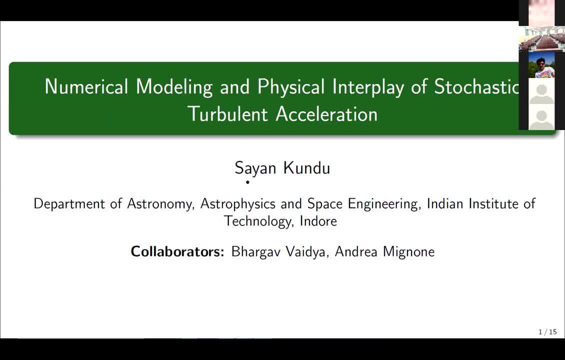 I'll give you a warning at around 10 minutes So you can start your presentation now. Hello everyone, I'm Shayan and the subject of my presentation today is numerical modeling and physical interplay of stochastic turbulent acceleration. I'll be focusing on a single astrophysical object, namely the radiolob of FR2J. 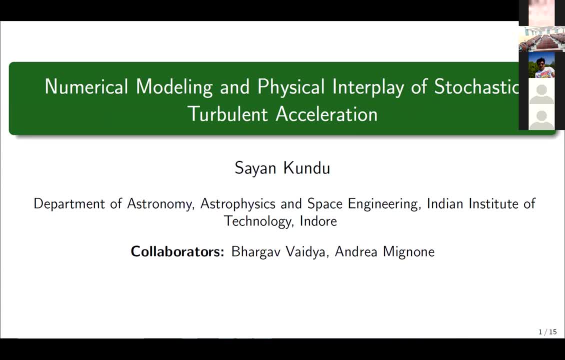 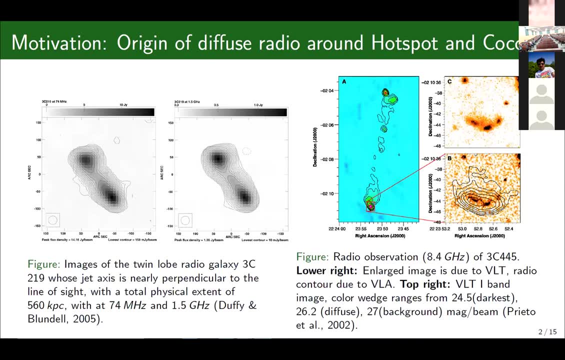 And this work has been done in collaboration with Dr Bhargav Vidya, who is my PhD supervisor, and Dr Andrea Mignone. So first let me tell you why stochastic acceleration is important. There are observations which indicate turbulent acceleration. as a candidate to explain certain observational features, 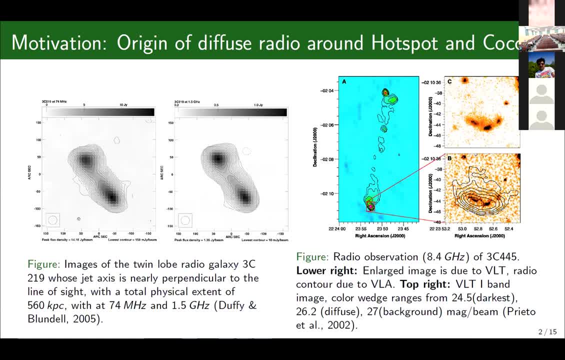 Likewise, in the left panel we can see a radio galaxy in two different frequencies. An interesting observation is that the size of the radio galaxy does not shrink with increase in frequency, as it should be, because of various radiative losses. That implies the presence of some distributed acceleration in energies to energize this particle. 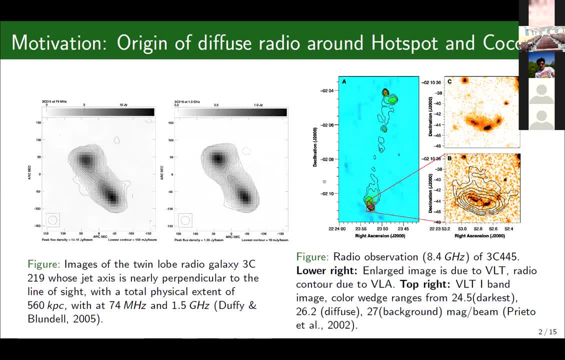 So that they can radiate even in higher frequency. Another plot here in the right hand side shows a diffuse emission around the hotspot region of the radio galaxy, which also requires a distributed mechanism present around the shock region to induce a diffusion in the emission. 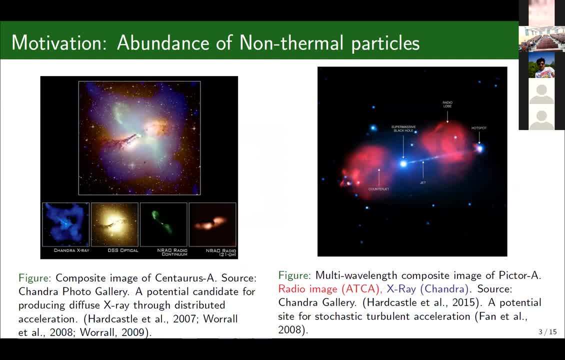 Also, there are certain observations which say that the Aegean jets are found to be found to have a Aegean jets are found to be found to have a X-ray kind of halo around it. Here in the left panel we show a plot of Centaurus A, which is a FR1 radio galaxy. 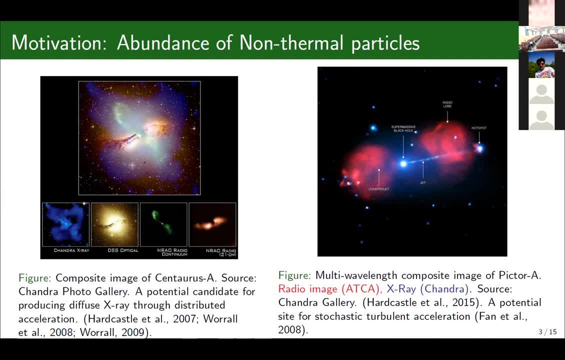 where you can see the blue line, depicts a radio emission. This radio emission, some sort of distributed emission, some sort of distributed acceleration process, has been attributed to indicate this radio emission in a FR1 galaxy. Similarly, in a FR2 galaxy, as I have shown here in the right hand side. 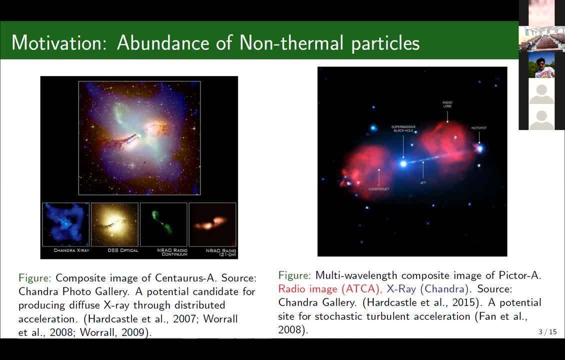 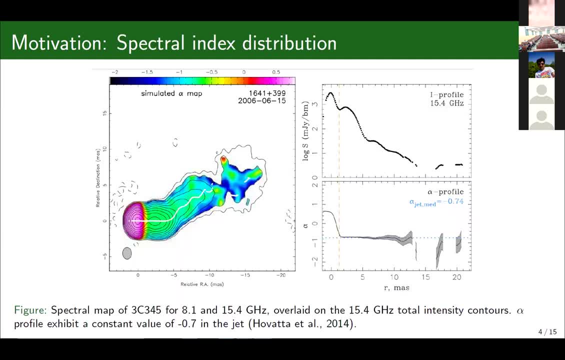 we can show. we can see a FR2 galaxy which is submerged in radio kind of halo, shown in blue. Moreover, observation suggests that in radio lobes spectral index maintains a constant kind of value. Here we show such radio lobe where one can observe a constant spectral index kind of structure. 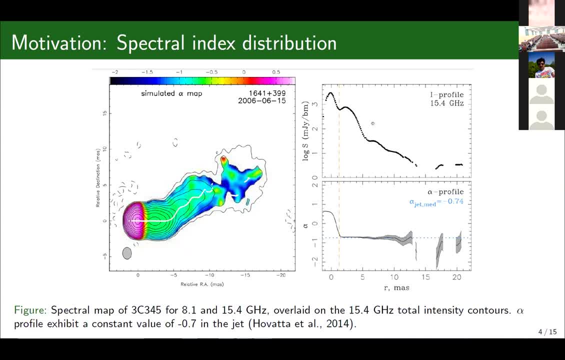 As we, as we move along this white line In the in the top panel, we show- or it's, it's been shown- the, the, the flux with this, with this distance, when, when one travels to this white line, 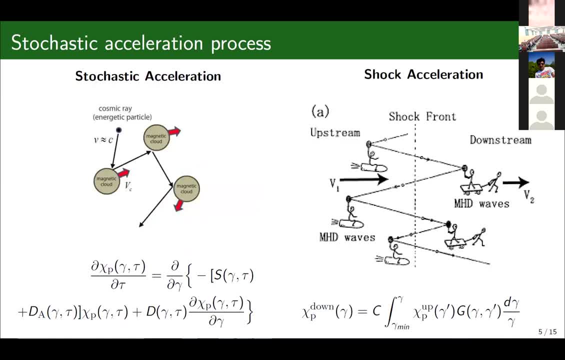 Being said that, let me tell you how this stochastic acceleration works. Stochastic acceleration is a process where non-thermal particles get energized by random interaction with MHC waves and magnetic inhomogeneities. Particles can both energizes and de-energizes. 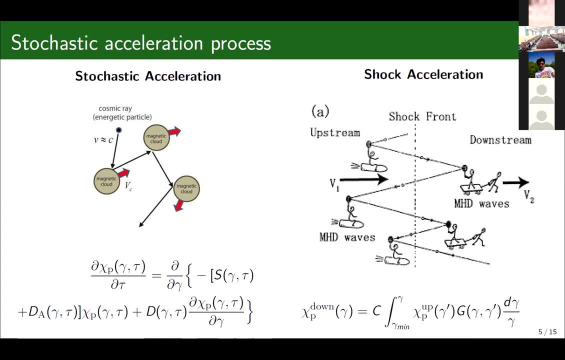 in this process And that is the origin of stochasticity in the stochastic acceleration process. This process is usually numerically modeled with, with a, with a Fokker-Planck equation, where this diffusion coefficient takes care of the random energization. 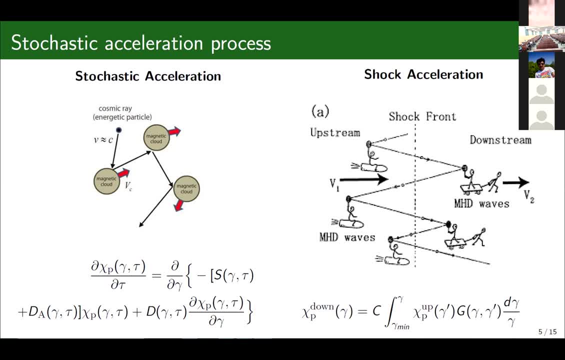 There is another acceleration process, which is known as shock acceleration, where the particle gets energized by crisscrossing the shock. The numerical implementation of the numerical modeling can be done of this acceleration process by this way, where one confers the upstream spectra with a suitable kernel to the downstream spectrum. 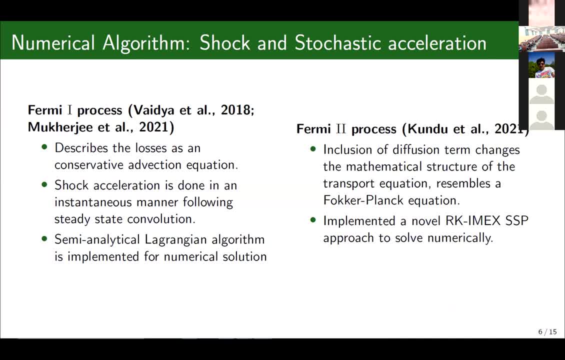 The shock acceleration has already been implemented in the code, in the code Pluto, which we use for our simulation, and with various radiative losses We extend the already implemented module by incorporating the stochastic acceleration. We have used a second-order accurate RK-IMAX SSP algorithm. 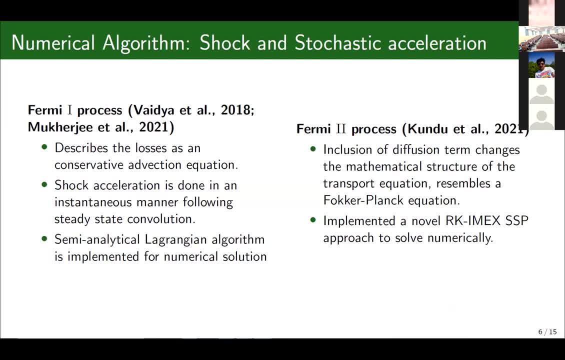 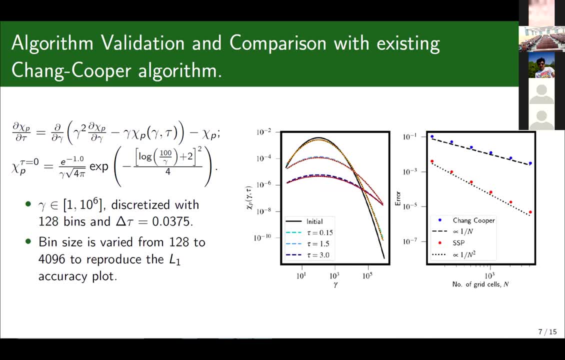 which gives a second-order accuracy even in non-uniform logarithmic grid. Here we compare the numeric, we compare our numerical scheme and with the analytical result to validate the scheme. We also show a comparison with the Chang-Cooper algorithm. We consider this Fokker-Planck equation with this initial condition. 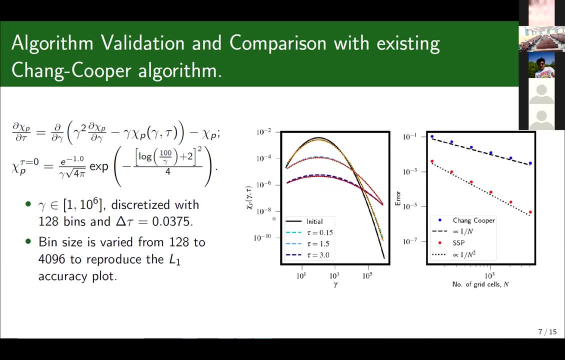 and the following computational geometries And, as you can see from the from this plot, our result, which has been shown with a dotted line, matches very closely with the analytical result which is shown in the solid line in compared to the Chang-Cooper result. 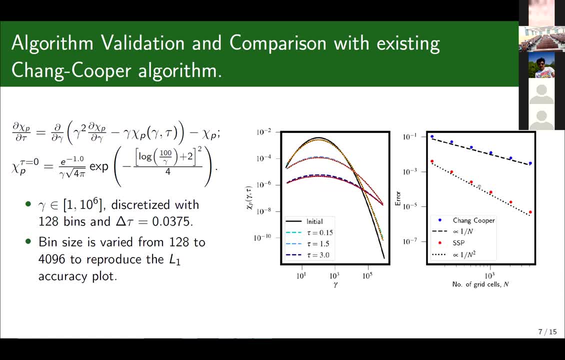 which is shown by the dashed line. Also in the right-hand side plot, you can see the accuracy of our code, which is SSP, is of second order, whereas the Chang-Cooper gives a first-order accuracy only With this numerical code of energy. evolution of non-thermal particles. 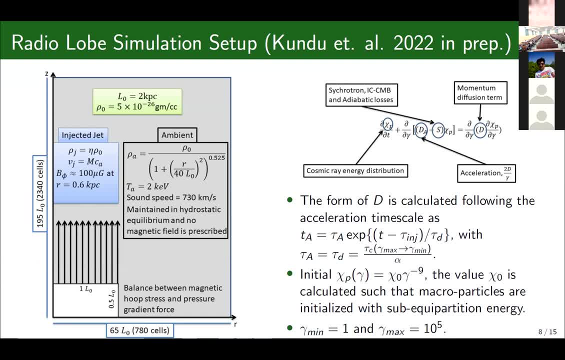 we proceed to simulate the radial lobe of FR2Z. We consider a non-relativistic axisymmetric simulation to create these lobes. For dynamical simulation we consider a non-magnetized ambient medium with a King's-like density profile and temperature of 2 keV. 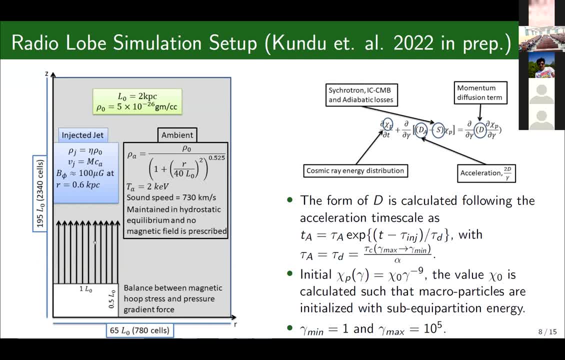 We then inject a light jet through the cylindrical nozzle with the jet parameter shown in this cartoon For the emission modeling. we inject enough macroparticle to uniformly fill the entire jet cocoon To evolve the energy distribution. we solve this equation with various radiative 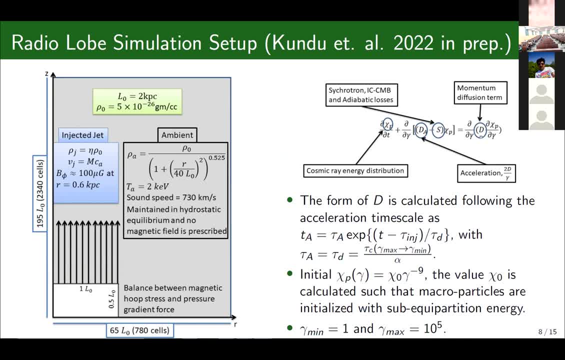 with various losses, and a phenomenologically motivated term for acceleration timescale to simulate this momentum diffusion and acceleration. This is the timescale that we have chosen. This timescale has the ability to mimic the turbulence decay process usually observed in various astrophysical scenarios. 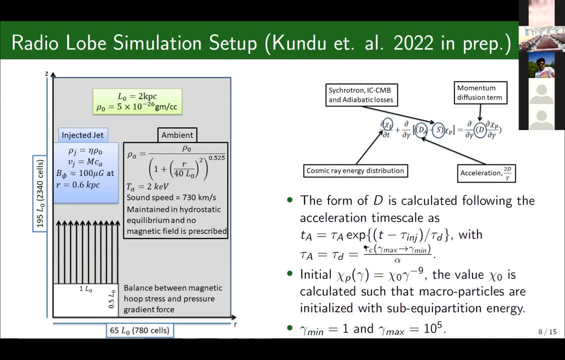 This tau c is the cooling timescale for each and every macroparticle, from gamma x10 to the power of 1,, gamma x10 to the power of 5, to gamma min 1.. And alpha is a parameter that we tune to get various acceleration scenarios. 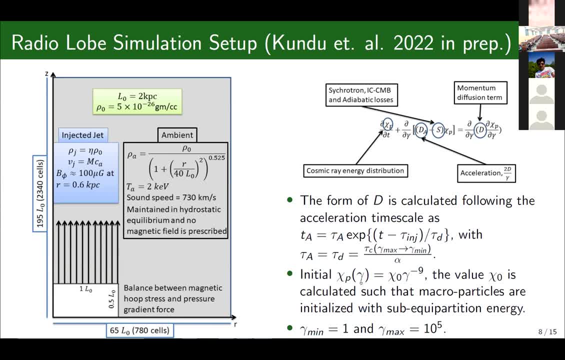 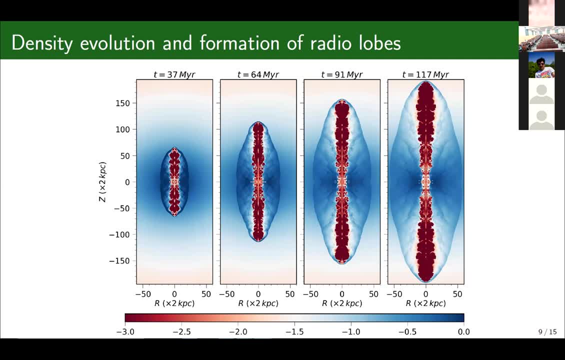 We solve this equation with an initial condition of a very steep power law given by this. Here we show the density evolution of our simulated jet And one can see a thin lobe kind of structure being formed at very early time which through time expands transversely. 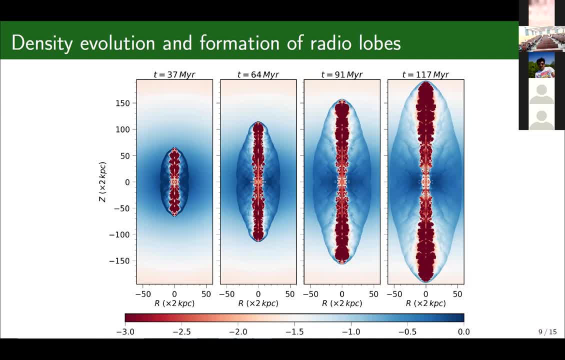 to give a radial effect. This is the radial effect of a radial lobe kind of structure. at later time Further, all our simulation or all our results would be partying to this last timescale where the radial lobe could be seen to form. 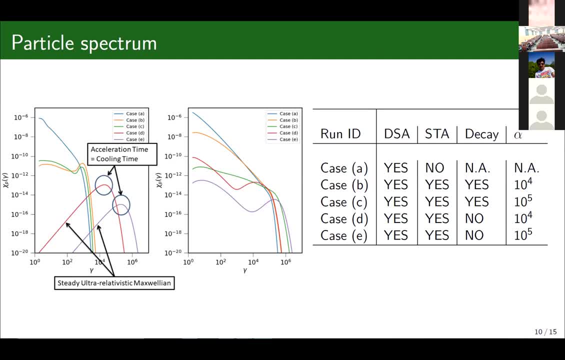 Here we show the effect of stochastic acceleration on single particle spectrum for various case scenarios as shown in this table. We have considered five case scenarios And these two plots depict particle spectrum for two different macro particles which got shock at different times. For case A one can see as shown in this blue line. 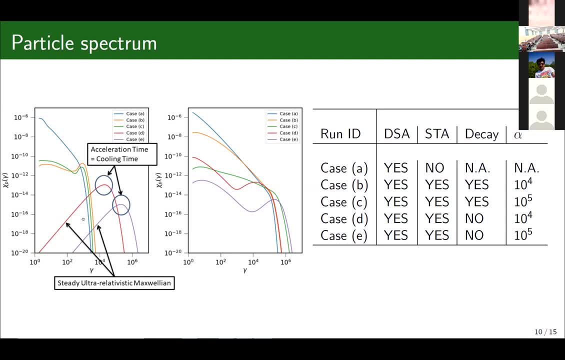 one can see a power law kind of spectrum with an exponential cutoff which is typical for this kind of behavior or for shock acceleration kind of behavior. For case D and E, where turbulence decay process has been turned off. one can see an ultra relativistic Maxwellian. 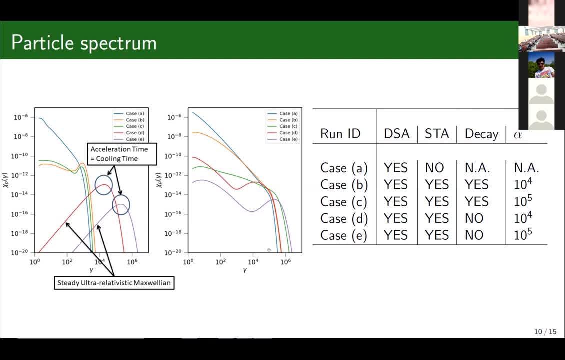 kind of structure being formed for this macro particle where some transient feature for this macro particle which indicates that the particle spectrum is in process of getting into an ultra relativistic Maxwellian. Interestingly for case B and C, where the turbulent decay process has been taken into account. 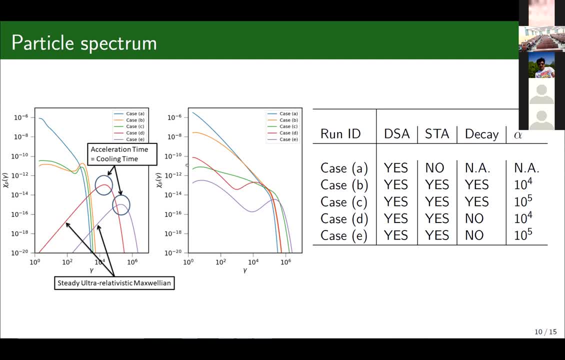 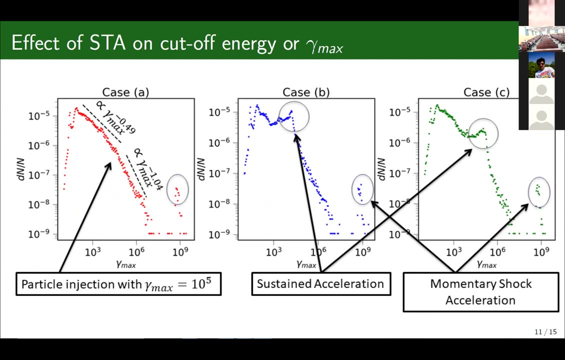 one cannot see a steady state kind of spectra for the particle spectrum, but one sees a cutoff which moves towards a lower energy. Now, after showing the effect of single particles, we show the effect of stochastic acceleration on collection of particles. Here we show the histogram of cutoff energy. 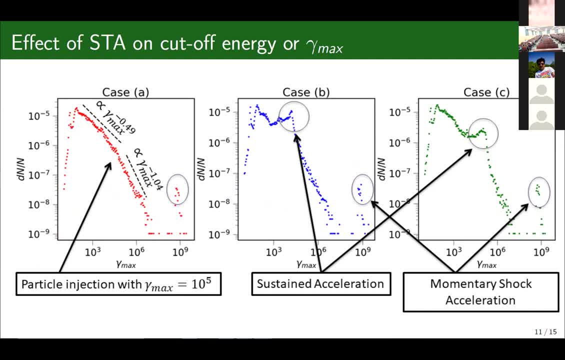 due to various cases, as described in the previous slide. For case A, we can see a broken power law kind of structure for the cutoff energy histogram and the break corresponds to the particle injection. as I have shown above, The break kind of depicts the particle injection. 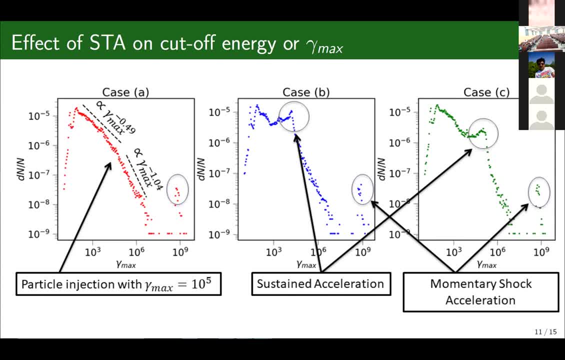 with gamma max 10 to the power 5. It is a continuous process. That's why a break occurs here, Whereas for case B and C, where turbulence decay process has been taken into account along with STA, one can see some additional peaks. 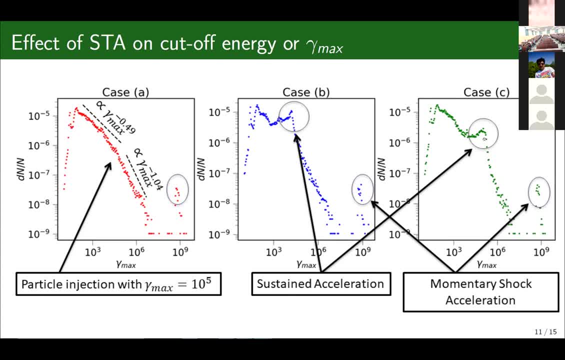 is getting formed due to the sustained acceleration that the STA provides to the non-thermal particles. One can also see some transient kind of peak, which are due to the macro particles are momentarily getting shock accelerated in the system. Here we show the synthetic spectral energy distribution. 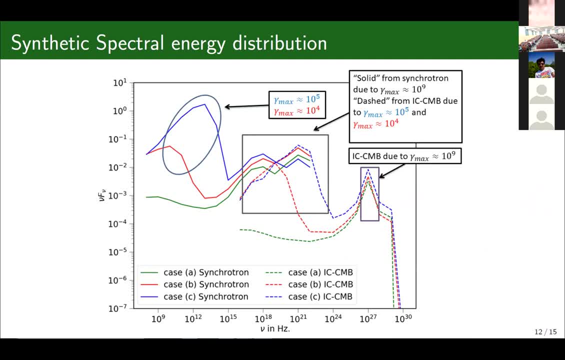 of our simulated radio loop where one can see for stochastic acceleration. when stochastic acceleration is taken into account, some low frequency peaks can be seen to occur here. Some peaks can be seen in the X-ray kind of regime as well because of the transient feature that I have shown. 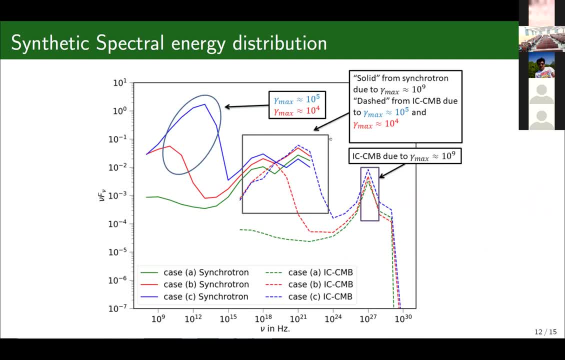 in the earlier slide. Interesting thing is to note that with stochastic acceleration one can get a significant amount of X-ray emission due to ICCMB, which were not present in the case of only shock acceleration. These peaks are also a manifestation of the transient peak that I have shown above. 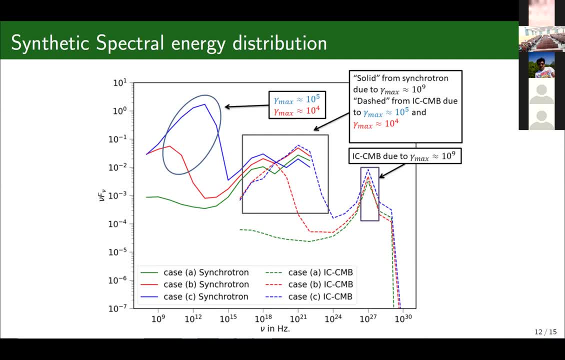 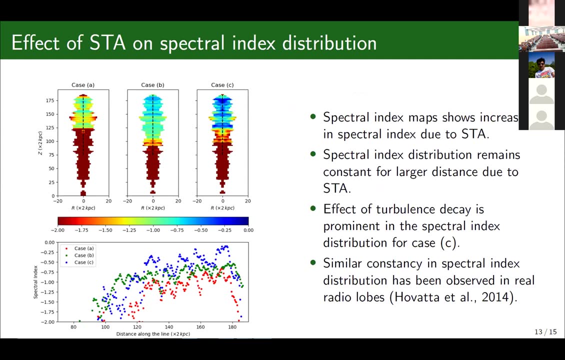 So one thing is that all the peaks shown here have a direct correspondence to the peaks that I have shown in this slide. Further we show the spectral index map of radio loop for different cases. The spectral index distribution following the black line can be seen here, where one can see. 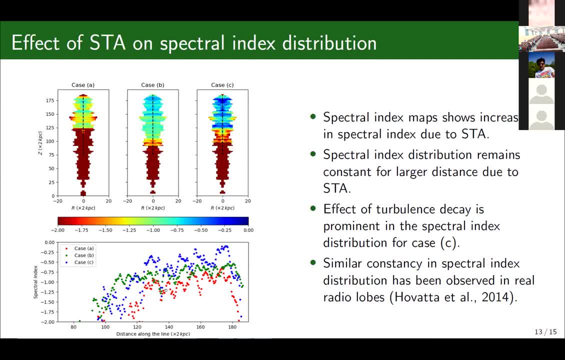 the spectral index gets a very minimal kind of value for the case of only shock acceleration, where the value gets increased when stochastic acceleration is induced And the span of the constancy can be seen to get decreased with higher stochastic acceleration because of the turbulence decay process. 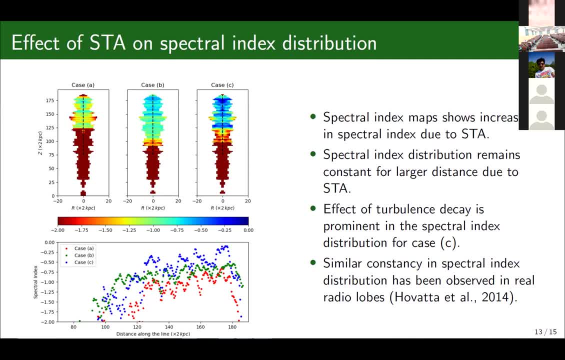 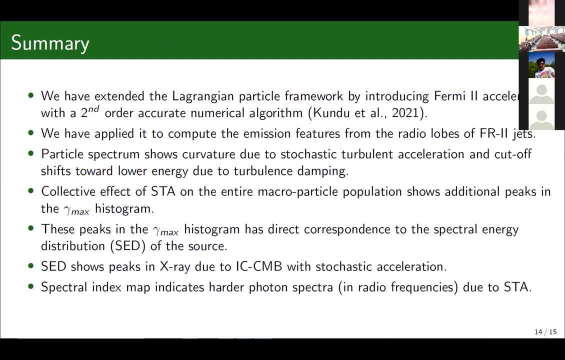 And as I have shown in the motivation slide, this has been observed in various observations as well- that radio loop kind of give a constant spectral index distribution which can get modulated If we tune the stochastic acceleration. So by this we come to the summary of our work. 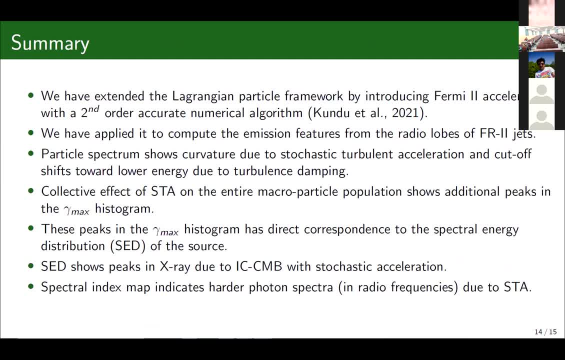 So we have extended the Lagrangian particle module by incorporating Fermi second-order acceleration process with a second-order accurate numerical algorithm. We then applied the numerical algorithm in order to compute the emission features from radio loops of FR2 jets Particle spectrum. as we have seen, 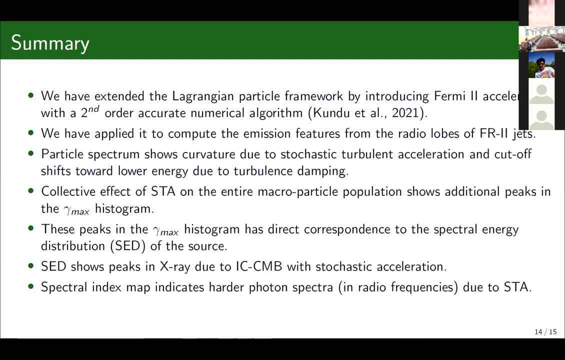 shows various curvature due to the stochastic acceleration process and the cutoff shifts towards the lower end due to turbulence damping, where, without turbulence damping scenario, we got to see a particle spectrum which was steady in nature. Also, in the collective effect of STA, we can see various additional peaks. 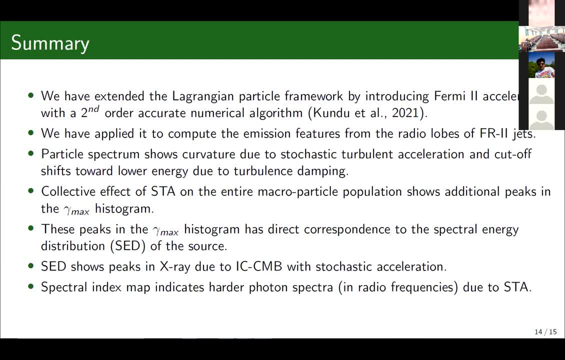 in the cutoff energy distribution which has a direct correspondent to the peaks observed in ACD. The ACD shows peaks in X-ray due to ICCMV, which we can only get due to stochastic acceleration. Also we have shown the spectral index map. 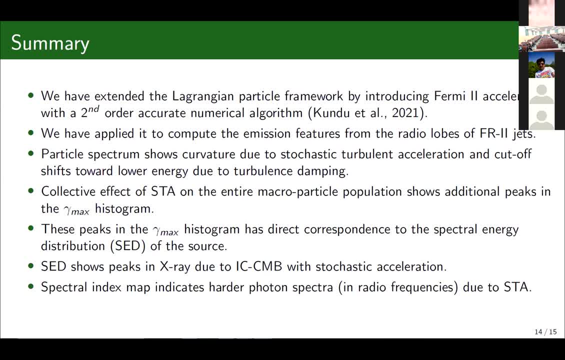 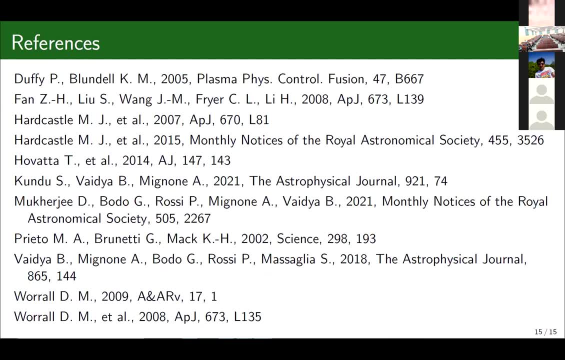 which indicates a higher photon spectra or harder photon spectra in radio frequencies due to STM. That concludes my talk, Thank you. These are the references. Thank you, Shyamal. Questions from the Let you roll, Shyam. very good work. 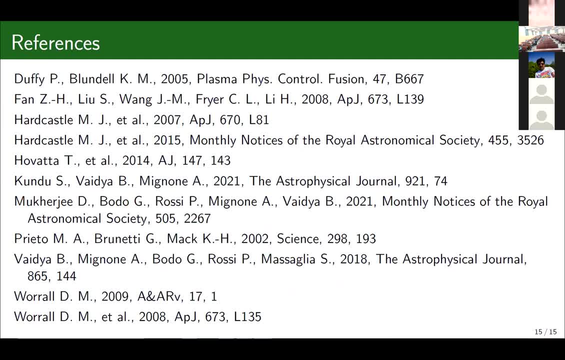 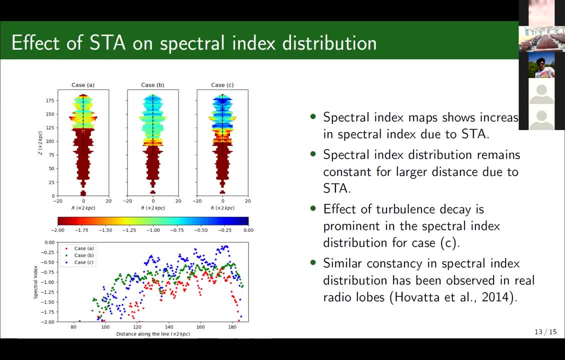 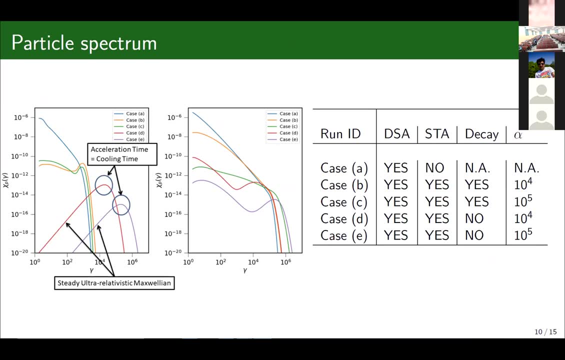 Extremely good work, Thank you. The particle injection that you are I found this particle evolution of acceleration and all So this particle injection that you are giving, probably at the base of the jet or somewhere, Yes, But what is your? 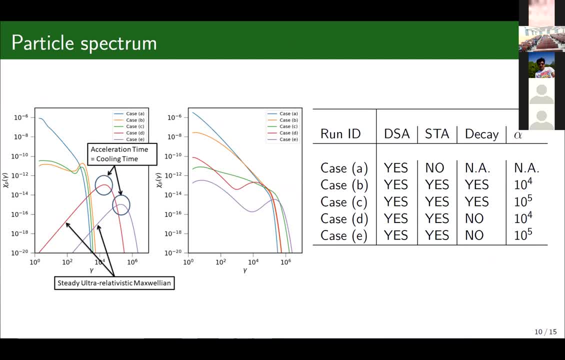 How you are guessing that number. Okay, okay, So Is there any physical argument in which you are fixing the normalization parameter as well as the power law? Okay, So the thing is, the particles that we are injecting at the jet base does not have anything to do. 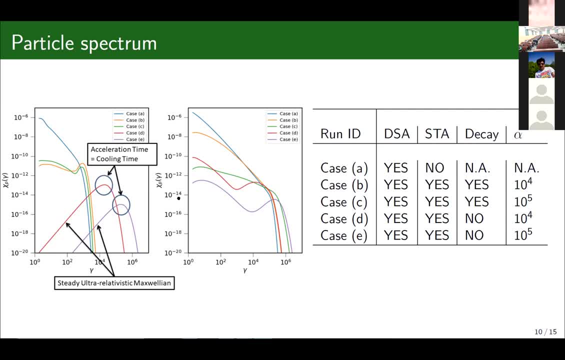 with the particle spectra that I have shown here. Those particles are the Lagrangian particles. that will going to flow, that will going to flow along the fluid, But here we have taken the initial spectrum to be like this, as I have shown. 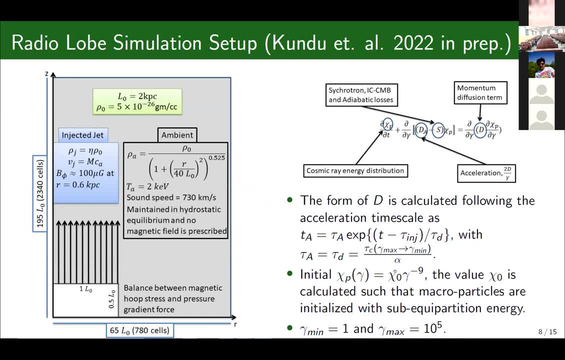 And the Chi naught part, which is the normalization part, has been taken such that the particle stays in a sub-equipartition regime. So we calculated the magnetic field at the jet base And considering that magnetic field we have injected the macro particles. 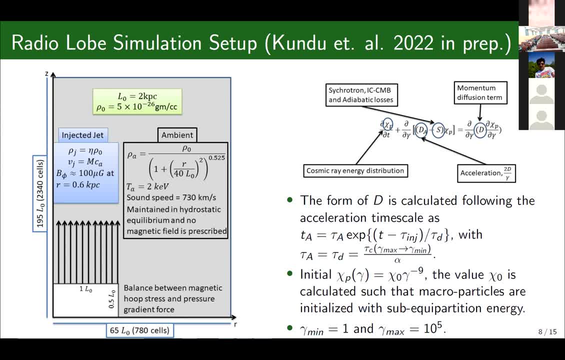 with an energy distribution which has a normalization due to the fact that particles are staying in the sub-equipartition regime, And then we let those macro particles to flow with the fluid And we see how the particles distribution gets changed due to this stochastic acceleration. 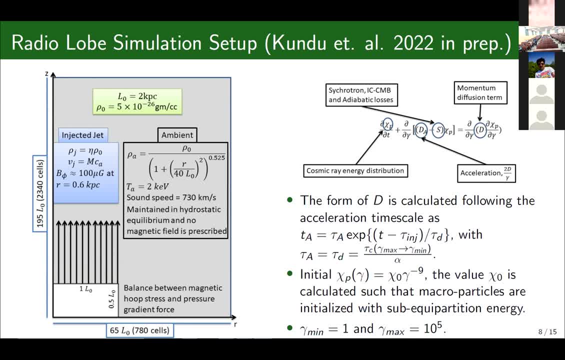 So the injection of the macro particles has nothing to do with this particle spectrum that I have shown here. The particle spectrum only gets governed by the normalization factor that we have shown here And which tells you that the particle starts with a sub-equipartition energy. 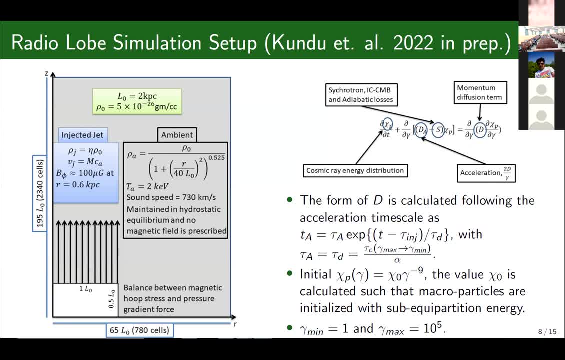 That's it. No, it will not. I mean, whatever you inject will not have any effect there, because after all solving a diffusion type equation, right, So that is understood Anyway. okay, So the macro particle injection is done by: 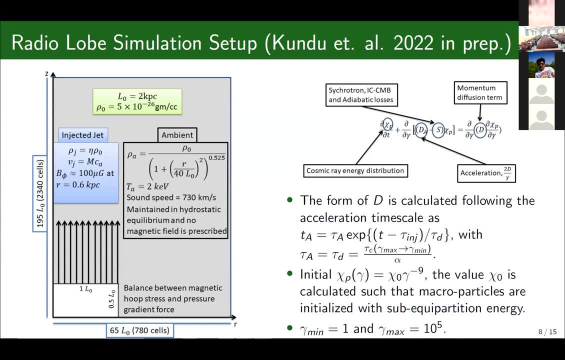 means two uniform we feel- the cocoon area or jet cocoon area, so that we can sample the whole jet cocoon area And we can sample all the energy spectrals and all the differences in the energy spectra that the jet cocoon induces. 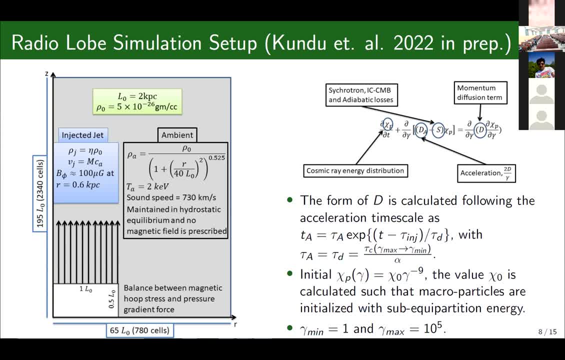 in the macro particles. Oh great, Any other questions, both from online and people present in the lecture hall? No, ma'am, There is no question. Okay, If there are no more questions, let us thank Shayan for his talk. 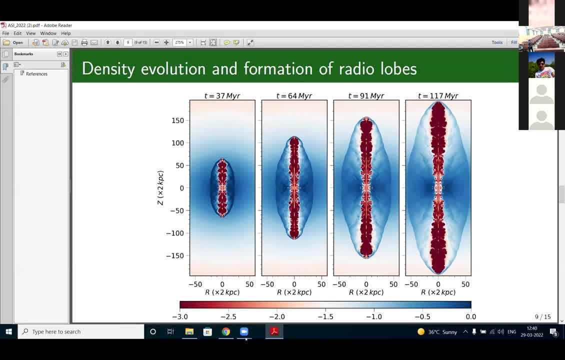 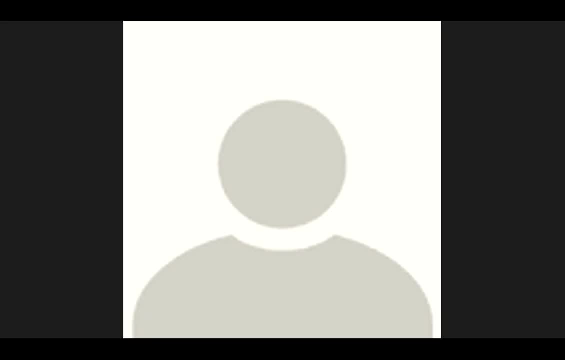 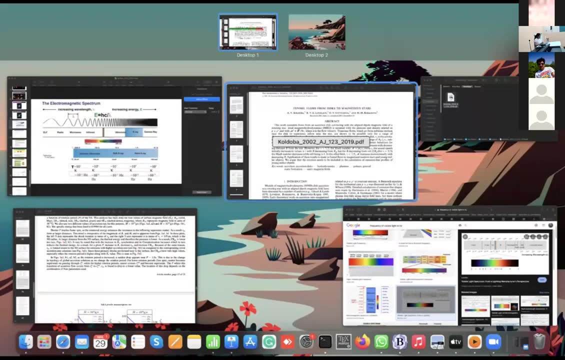 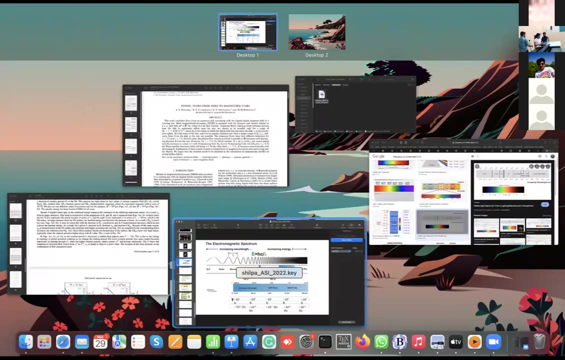 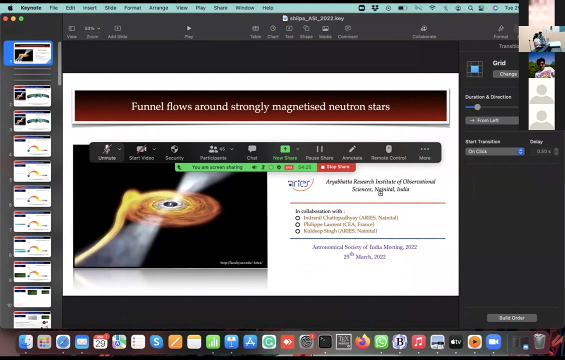 Thank you, We will continue our stream now. The next talk in this session is by Shilpa Sarkar, and she will be speaking about funnel flows around strongly magnetized neutron stars. I think one mic will have to be muted. There is a noise. 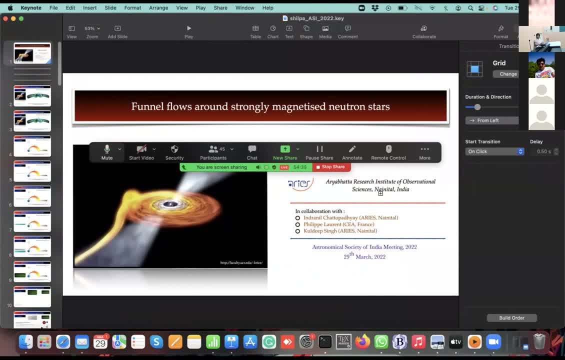 Shilpa, can you speak? Hello? Are you using your laptop? Then just mute this LHC one, I think. Try speaking now, Shilpa, try to speak something. Hello, Okay, Try. 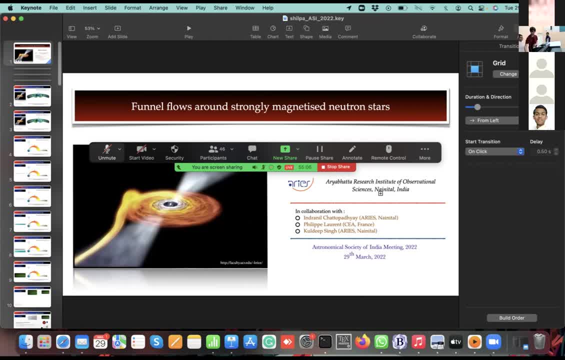 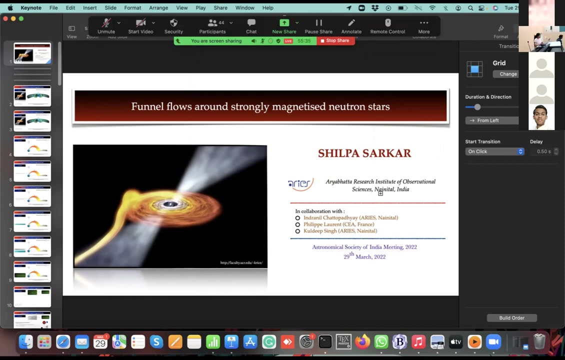 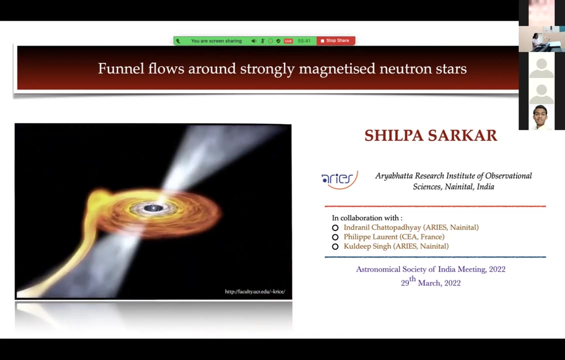 hello, can you hear me? yeah, yeah, it's better now, okay. so, shilpa, i'll give you a warning at around 10 minutes. so, hello everyone, i am shilpa and today i'm going to talk about. 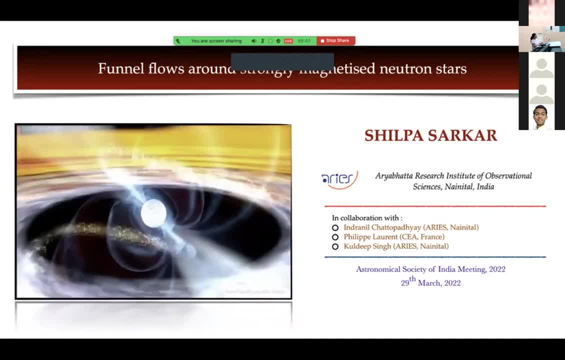 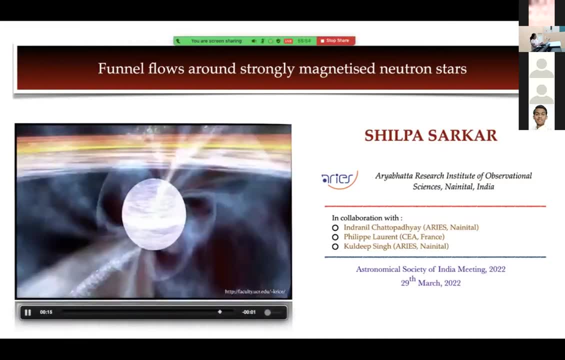 the accretion flows, which are also known as funnel flows, around strongly magnetized neutron stars. so here you can see a neutron star which is accreted matter from its binary counterpart. so the accreted matter has some angular momentum, because of which it first 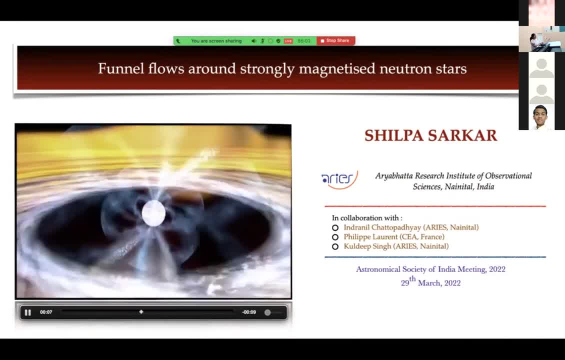 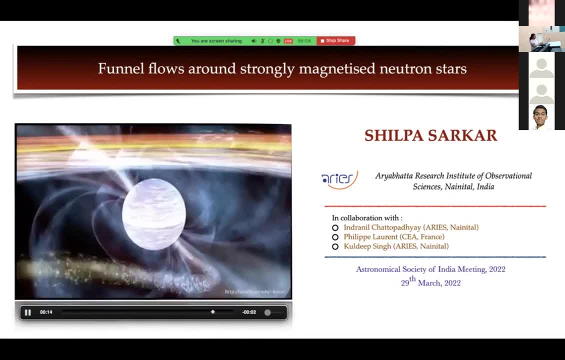 forms an accretion disk around the neutron star, after which, when the magnetic pressure of these field lines exceeds the ram pressure of the matter, this matter is strictly channeled onto the magnetic field lines until it reaches the poles of the star. so, basically, we are going to 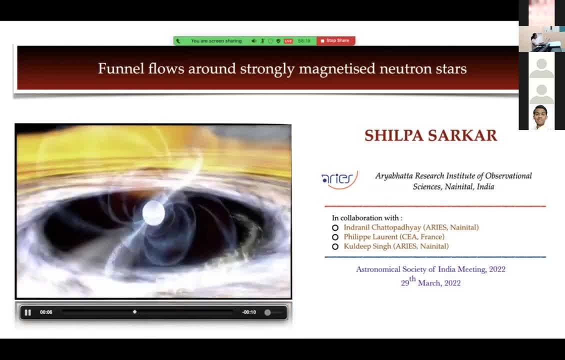 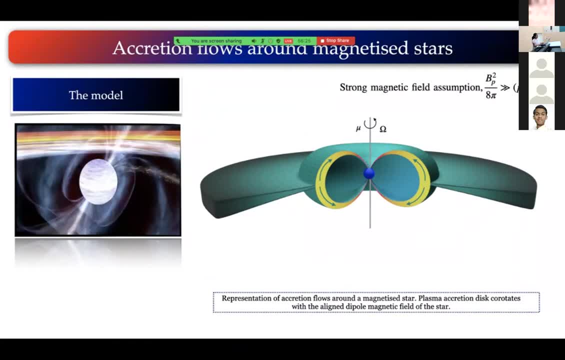 model this mainly to understand the underlying physics. so we are going to model this mainly to understand the underlying physics that is present in the systems. but modeling of these accretion flows is not trivial, and hence we took recourse to certain assumptions. the first assumption is that we consider the 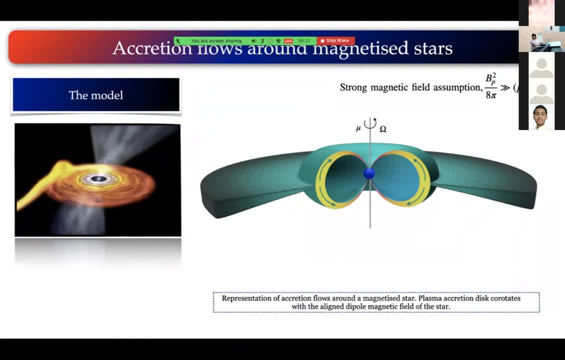 magnetic moment to be co-aligned with the rotation axis of the star. and the second thing is that we assume strong magnetic fields. so because of this, uh, strong magnetic fields, uh the matter, so there is no slippage between the matter and the magnetic field lines. and the second thing: 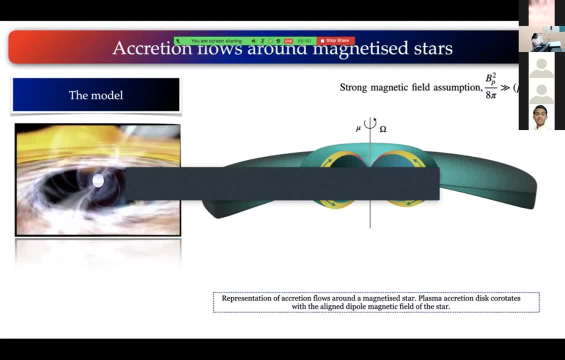 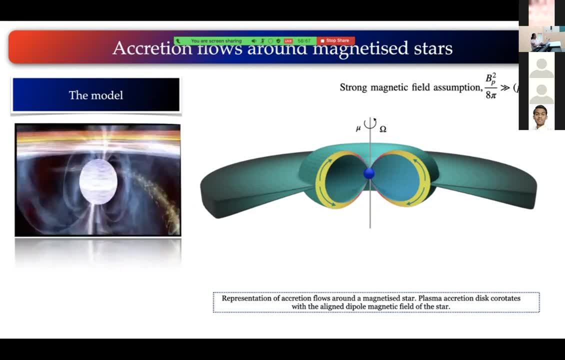 is that? uh, because of uh, since these field lines are strongly anchored to the neutron star surface, these magnetic field lines, as well as the matter, they co-rotate with the same angular velocity as that of the star. so, zooming into this section a bit more, so the matter accreted from the 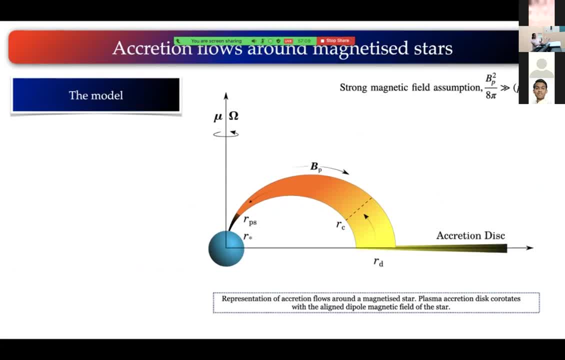 accretion. this is basically subsonic in nature, but as the matter is accreted further because of gravity, this subsonic matter becomes supersonic after crossing a certain sonic point. and then this supersonic matter, because of the hard surface of the neutron star, it forms a shock. 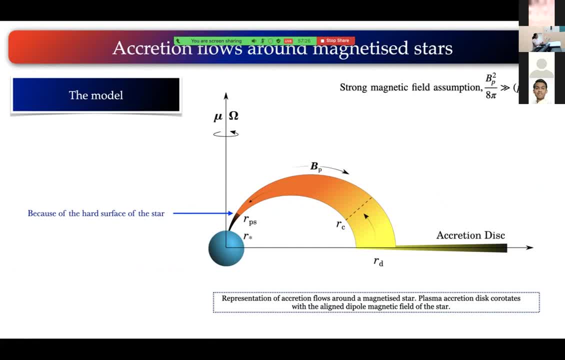 which is also called as the surface shock or the primary shock. so basically, this forms because of the hard surface and after this uh, the supersonic matter. it becomes subsonic and all the kinetic energy of this matter is radiated into the form of different emission processes, after which it slowly 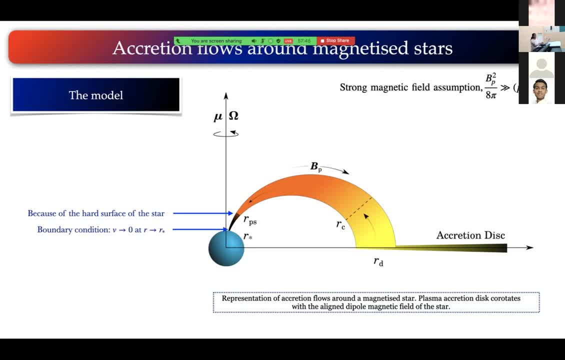 settles down onto the surface of the neutron star, satisfying the neutron star boundary conditions. that is, velocity zero at uh radius equals to the star surface. so most of the work that uh has been done till now they consider only this uh particular funnel uh, mainly because more than 95 percent of 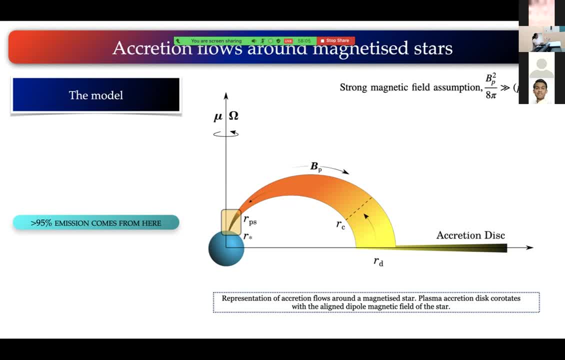 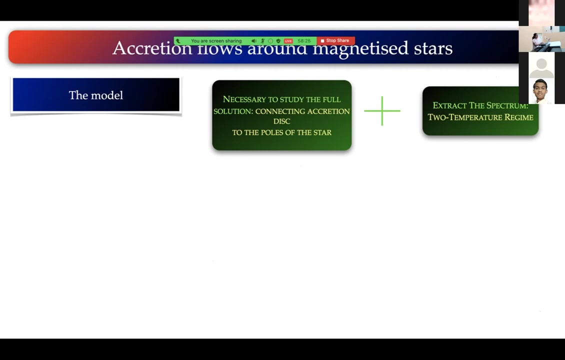 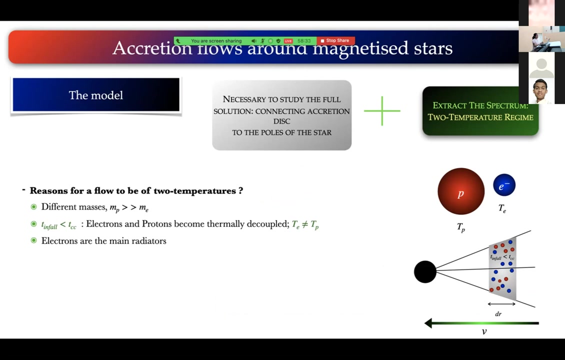 the emission comes from this region, uh, but as i will show you that there are distinct spectral signatures from this pre-shock region as well, so there is a necessity to study the full uh solution, or, uh, what makes a flow to be of two temperature, uh, so, mainly because, uh, there are different. 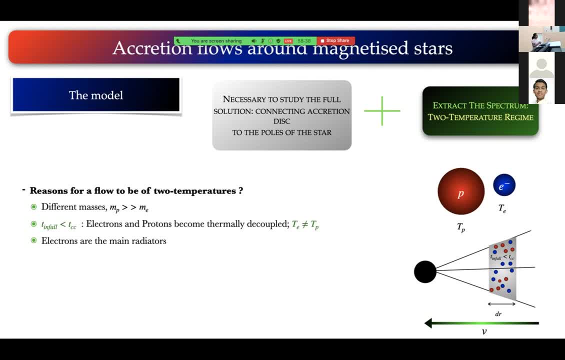 masses of uh because protons and electrons they have different masses and hence uh they will be prone to different emission mechanisms. the second thing is that the info times shorter than the cool uncoupling time scale. so cool uncoupling time scale is the time scale in. 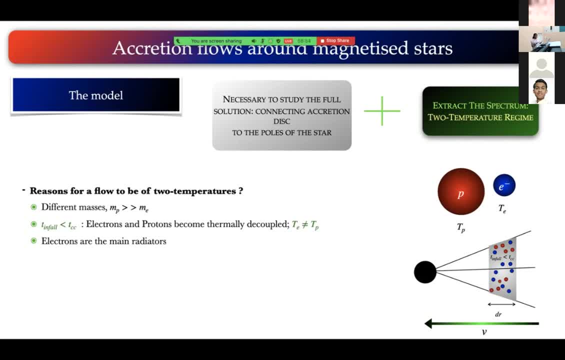 which, uh, the electrons and protons. they interact with each other and settle down into a single temperature distribution. so, before that interaction time scale, if the matter falls to the central object, then the electrons and protons. they will be thermally decoupled and they will possess two. 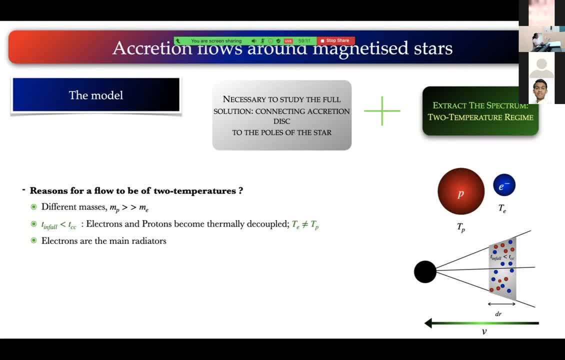 different temperatures and since uh. the third point is that the electrons are the main radiators, because brainstorm, synchrotron and everything they uh mainly means electrons are more prone to this radiative mechanisms. the temperature of the electron is bound to be different from the propane. 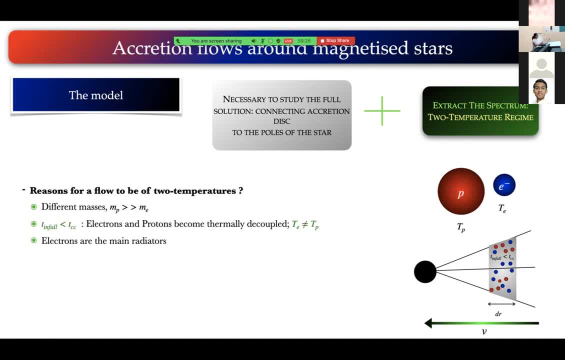 so we expect a temperature flow in the system. so, uh, these types of flows are generic in nature and since we have information of the electron temperature, it helps in computing the spectrum. so these types of flows are more realistic in nature. and now there is a serious problem. 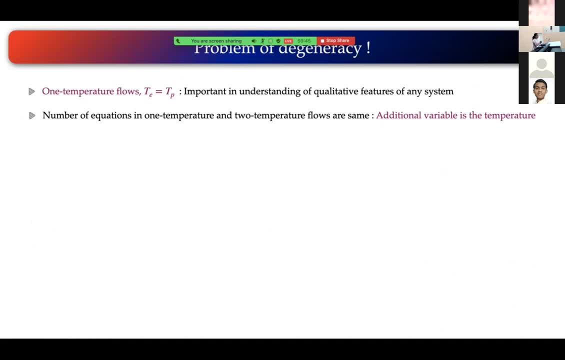 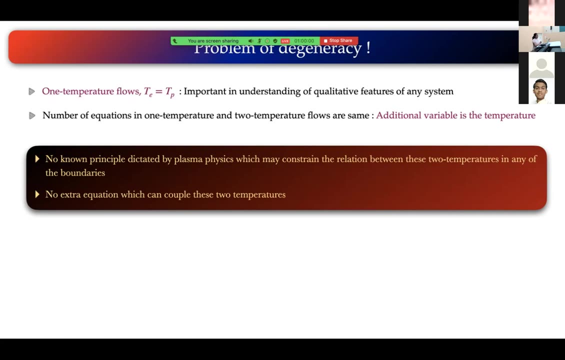 that exists in temperature flows. so one temperature flow is when the electron and proton have a single temperature distribution. so when we come to the two temperature regime, the number of equations doesn't change, but there is an additional variable, which is the temperature. so this says that uh. 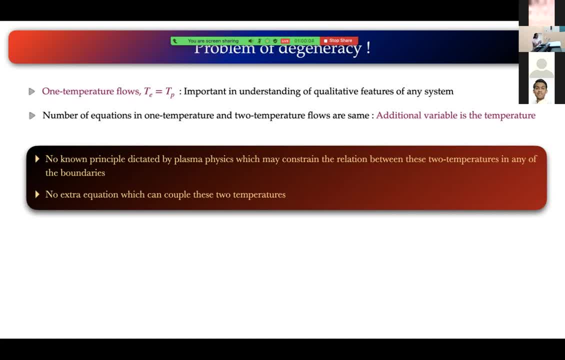 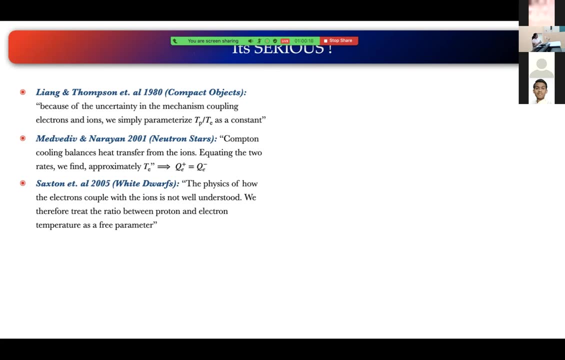 there the system is degenerate because we do not have any principle uh which may constrain the relation between the two temperatures, or no extra equation is there which may constrain the temperature region. so, uh, this problem is indeed serious because uh a lot of work have uh quoted these. 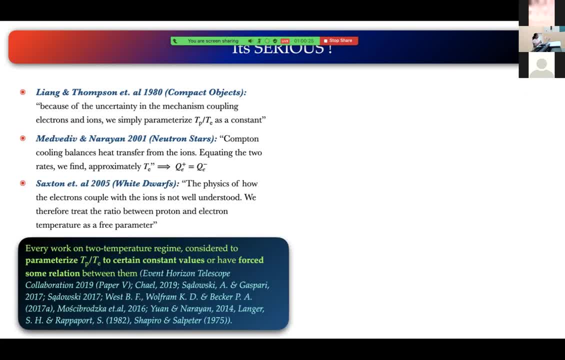 things, that there is a degeneracy problem. um, starting from 1980, and it is still, uh, the people tell that yes, there is a degeneracy. so how this degeneracy was removed in earlier works is that, uh, either they parameterize the proton and electron temperature to certain ratios or, uh, they 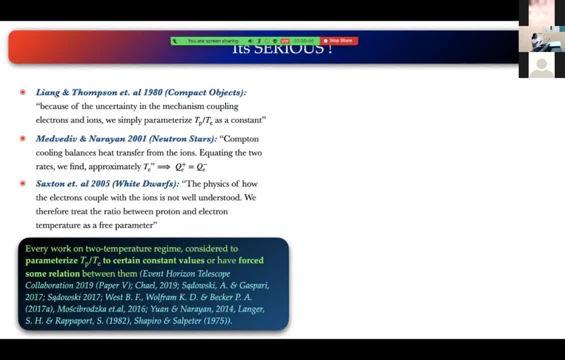 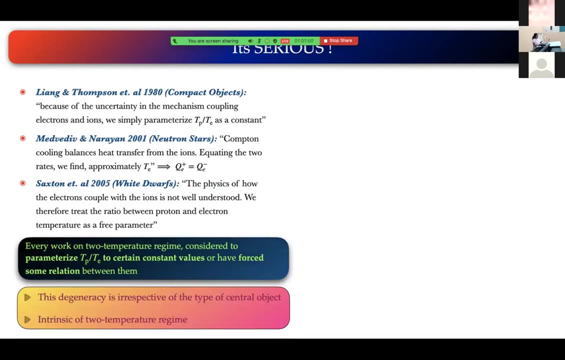 have some uh relation between them. that is, they have insisted some equation that, like the heating of the electrons is equal to the cooling of the electrons. so this uh made an additional equation because of which they could obtain the temperature. but this uh uh, so this degeneracy is irrespective. 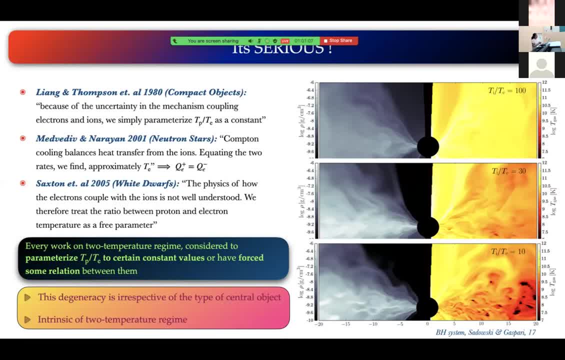 of the nature of the central object and it is intrinsic of two temperature regime. but this thing is not uh. uh means that this uh being like, uh parameterizing these things is not consistent. so in a recent simulation uh done by these people uh for accretion flows around black holes, you can see that they parameterize the 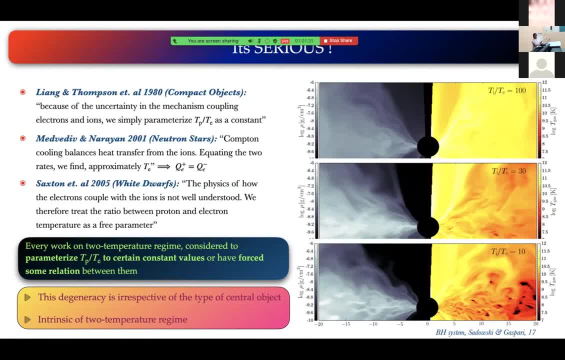 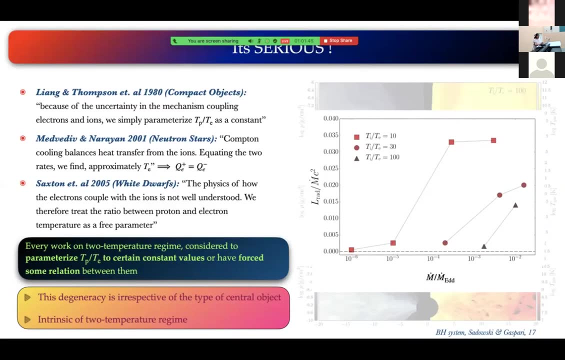 ion and electron temperature to different values and we can see that the topology of the system actually changes, actually differs, if we take different kinds of arbitrary parameterizations. even when they plotted the efficiency with respect to the accretion rate, we can see, uh suppose, for the 10 to the minus 2. 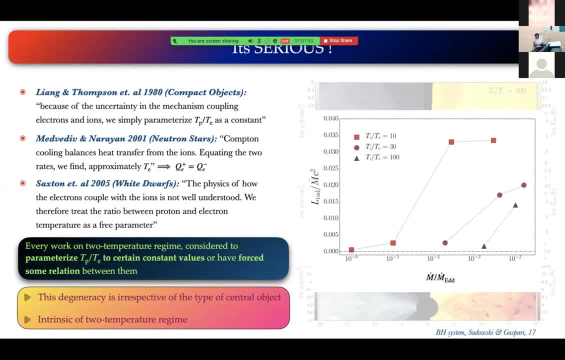 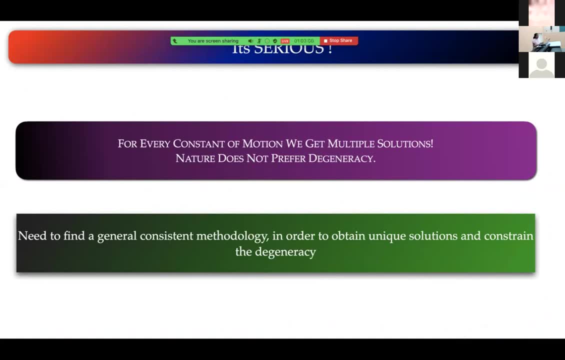 errington rate we can see with the different values of ratios the efficiency of the system changes. but this should not be the case. uh system should not be degenerate. for a given constant motion there should be a given solution. so there is a need to find a general, consistent methodology. 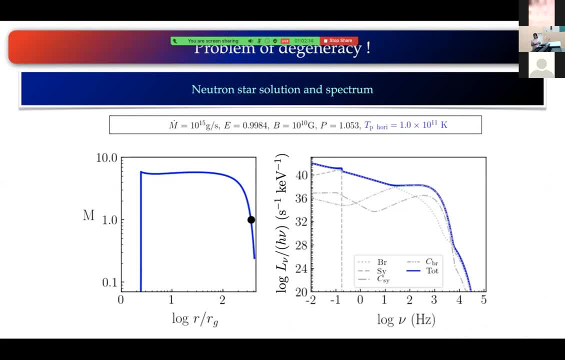 so, coming back to the uh neutron star case, uh, so this is uh what we call the mach number versus radius plot. so this is a neutron star uh accretion solution where the matter starts from subsonic values, crosses the sonic point, becomes supersonic and because of the hard surface, as i've said, 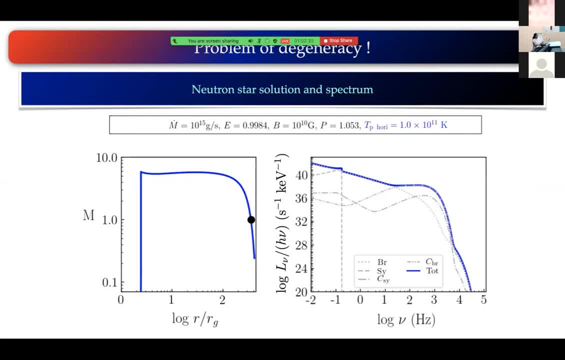 it undergoes a strong shock near the surface. and this is the corresponding spectrum obtained, uh from the different radiative processes like brimstone, synchrotron and their comptonizations. so these are the constant set of constants of motion. but for the same set of constants of motion, 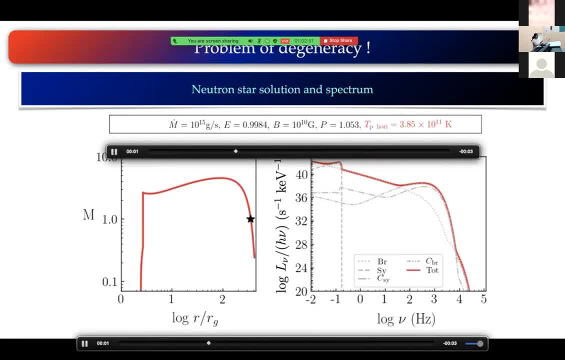 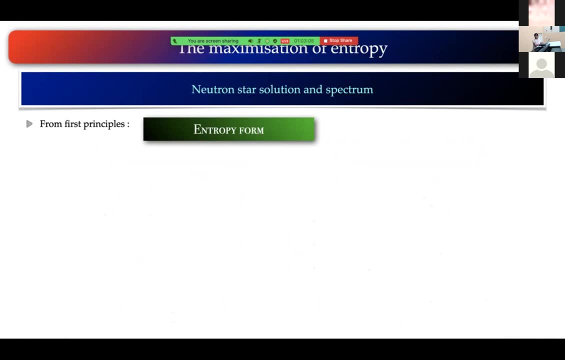 we can see that there are different solutions, where few solutions passes through the outer sonic point, few through the inner sonic point and few even harbors a shock and correspondingly, correspondingly, the spectrum also changes. so what we did is: uh, we found an entropy accretion rate. 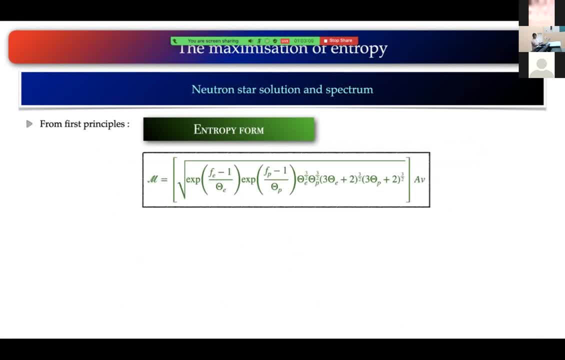 formula which is given like this. so we have validated this entropy accretion rate formula, that formula in case of black holes earlier. But the catch is that since the system is dissipative, so this entropy accretion rate form can be only obtained, the entropy measure mainly. 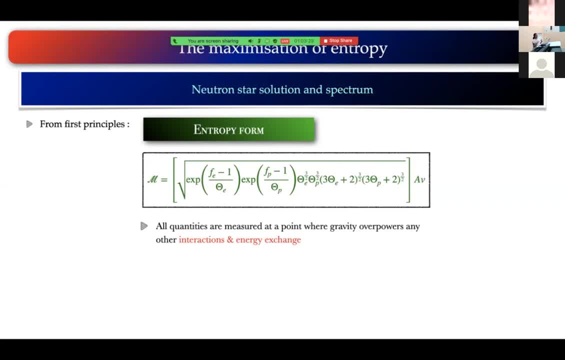 can only be obtained at a point where the gravity overpowers any other interaction, So the interaction timescales are very much larger than the in-fall timescales. So in case of black hole it was very easy and it was the event horizon when we could measure. 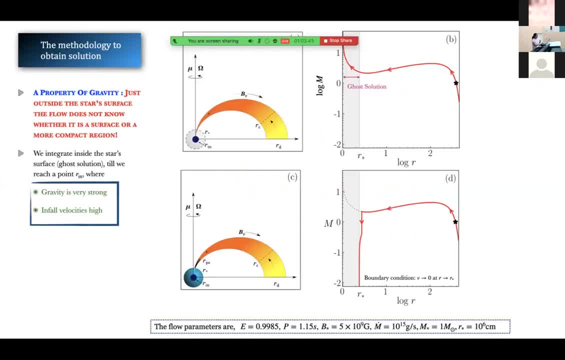 the entropy. But in case of neutron star this is not the case, because at the surface of the neutron star the velocity is actually zero and not the velocities are higher, where the in-fall timescales would be larger. So what we did is that we integrated the supersonic. 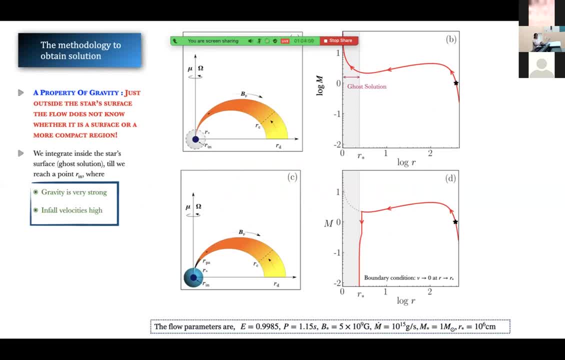 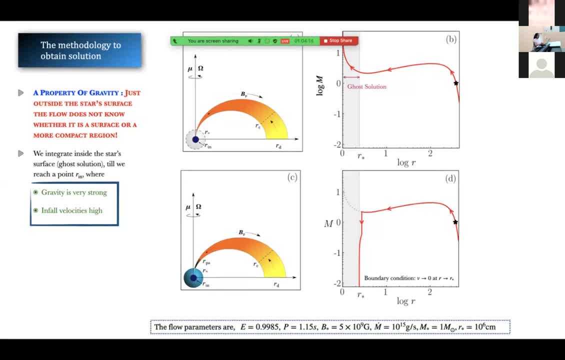 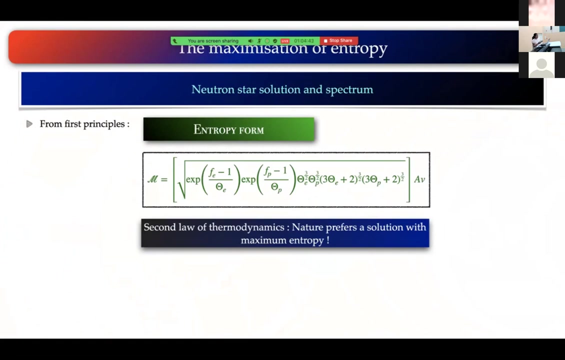 this is the entry chipsillage and this is the rapid flow inversion of this graph And the rotation keys to the integrating the belongs right now to derives from the massive imperfection 27 to the 1st part of this, of all the original solutions. we find that the entropy maximizes at a certain solution and 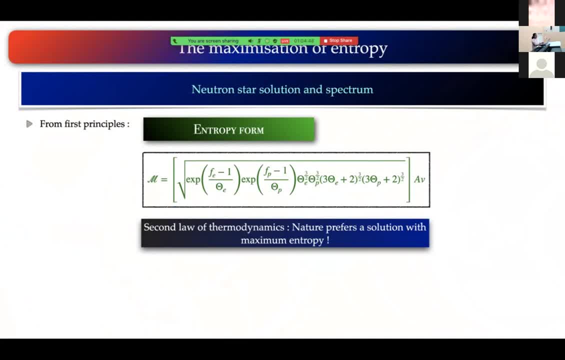 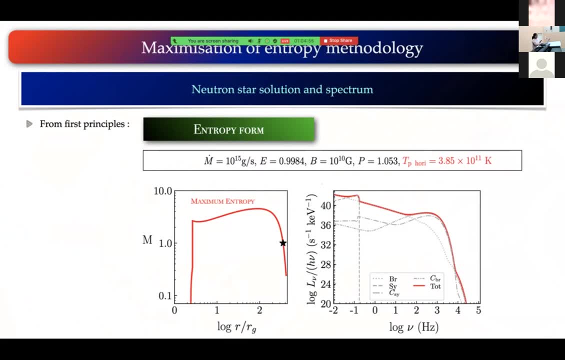 following the second law of thermodynamics, that nature prefers the solution with maximum entropy, we select that solution. so in the earlier set of constants of motion. so this is the maximum entropy solution where the solution passes through the outer sonic point and this is the corresponding spectrum. now this is a typical accretion solution and its spectrum. 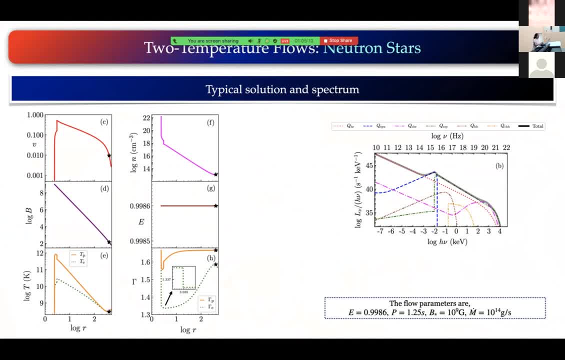 and these are the constants of motion for it. so this is the velocity plot, so the velocity as we can see, near the neutron star surface there is a jump to lower velocities, after which, when it nears the neutron star surface, the velocity decreases and finally it settles down onto the 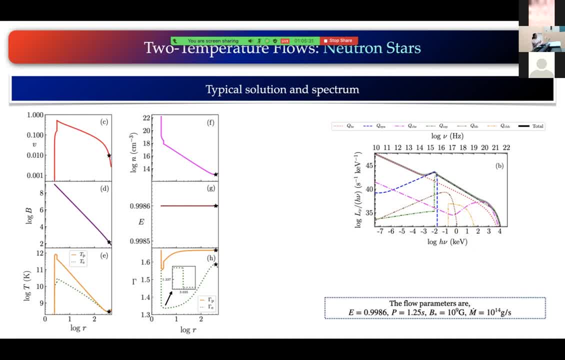 neutron star surface, while the number density increases as the matter is getting accumulated on the surface. and this is a magnetic field and this is a conserved Bernoulli parameter. and this is the. these are the two different temperatures. so this is the proton temperature, this solid line, and the dotted one is electron. 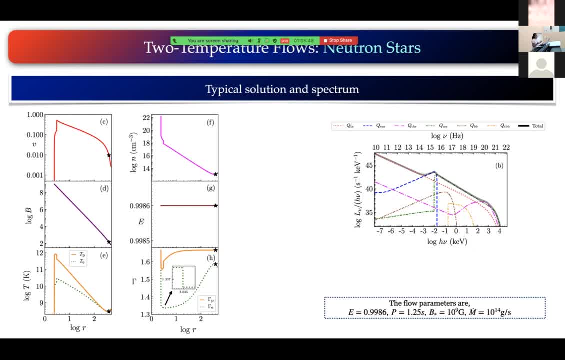 temperature. so we can see that the electron temperature is because it is more prone to radiation mechanisms, the temperatures are less. but when it reaches the neutron star surface, the temperatures of both the protons and electrons they decrease and they settle now onto some constant values, and this is the adiabatic index. 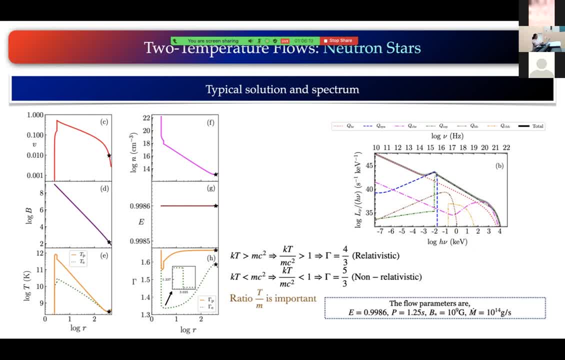 for both protons and electrons. so adiabatic indexes is four by three when the system is relativistic, while it is five by three when it is non-relativistic. so not. so the relativistic means that the thermal energy of the matter is greater than the response energy of the system and 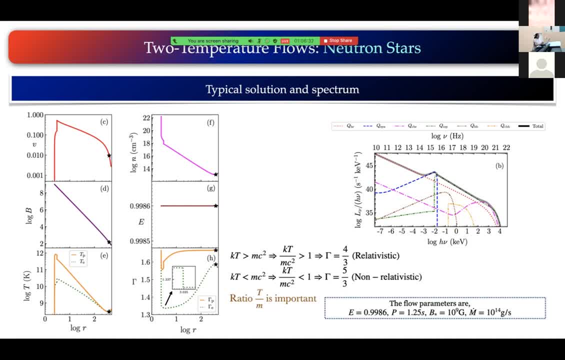 non-relativistic is when it is less so. not only the temperature but also the mass of the species is important. so, since we are dealing with two different species, we actually use the relativistic equation of state for multi-species flow and we can see that the protons and electrons, they are almost non-relativistic, very far away, while 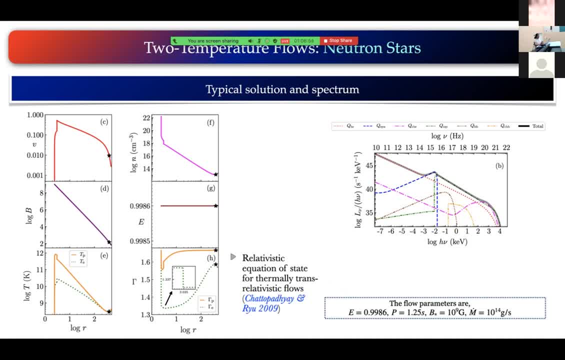 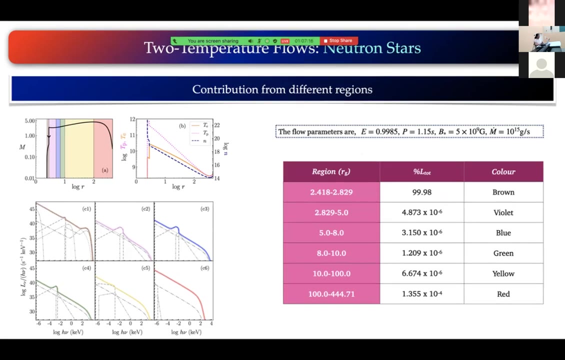 as the matter is accreted, the protons remain mildly relative, non-relativistic, but the electrons become relativistic, so there is a need to start to study these flows using a relativistic equation of state, so coming to the contribution of different regions to the total spectrum. you have two more minutes, yeah, so uh, we, uh, what we do is uh, divide. 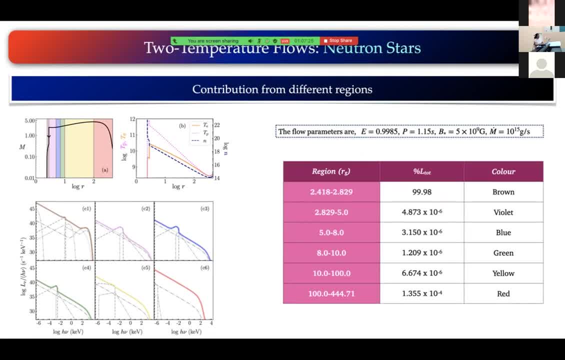 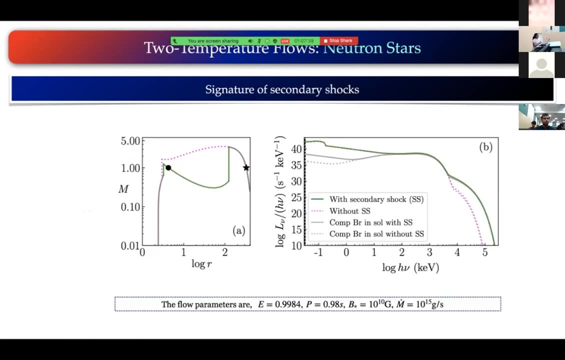 different regions and plot the corresponding spectrum and, as has been uh earlier uh discussed or concluded by most of the authors, we also found a 99.98 percent luminosity comes from a region very loss, that is 2.41 into 2.829. but as i have said earlier that there are signatures uh spectral, 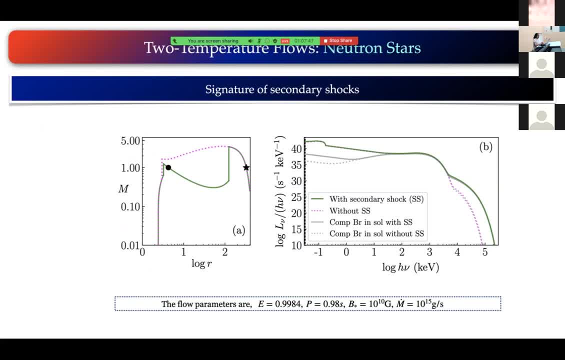 signatures uh of this pre-shock region. so these are the constant of motions which has a secondary shock as well, apart from the primary shock. so if this solution didn't have this secondary shock and the solution only passed through the ultrasonic point and had a primary shock, 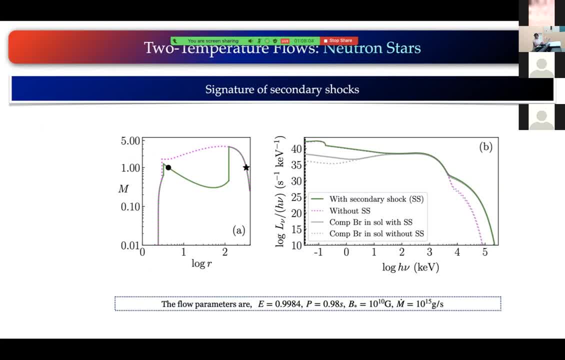 so these are the two spectrum which we get and we can see that there is an extended power load tail when in the pre-shock region we have a secondary shock. so this tells us that there is a need to study the full transonic solution, full accretion solution which connects the accretion disk to the 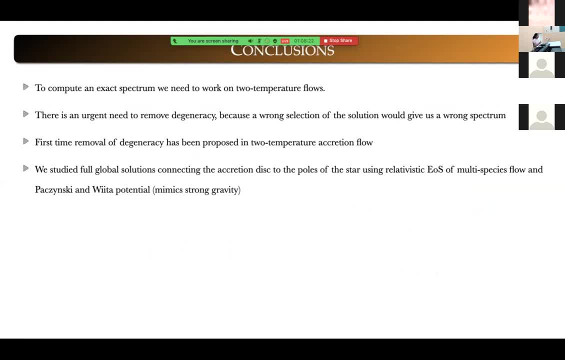 neutron star poles. so to conclude, uh, there is a need to work in the two temperature regime in order to obtain the spectrum and there is a degeneracy problem which we need to attend and get correct information of the system. and we have done that and we didn't. 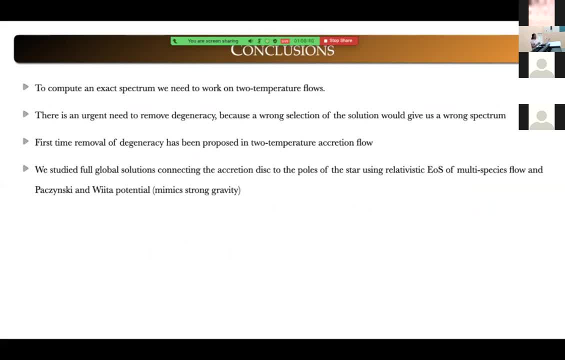 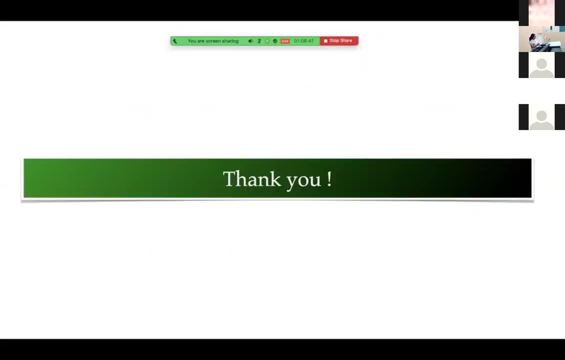 study only the funnel. we actually studied the full global solution and full accretion solution, which is actually needed to get a bigger picture of the system. so thank you. thank you, shilpa. questions from the audience. this work, i was just wondering what one is that. 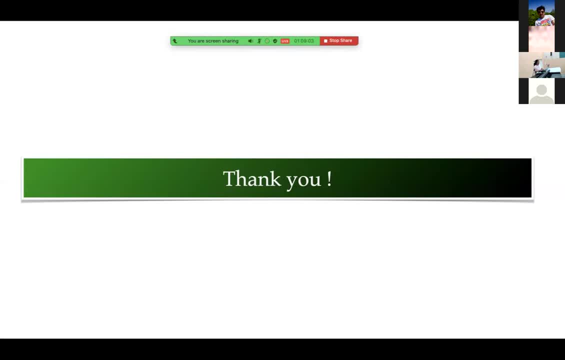 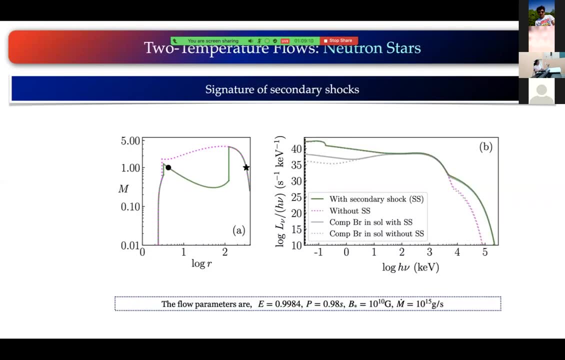 this is 1d, right? yeah, so we know that uh cooling flows. this is basically you have. yeah, so cooling flows sometimes are stable in uh radial contributions, but you could inject non-radiance contributions, for example azimuthal or meridiana, then it becomes unstable. so will it really hold these into? 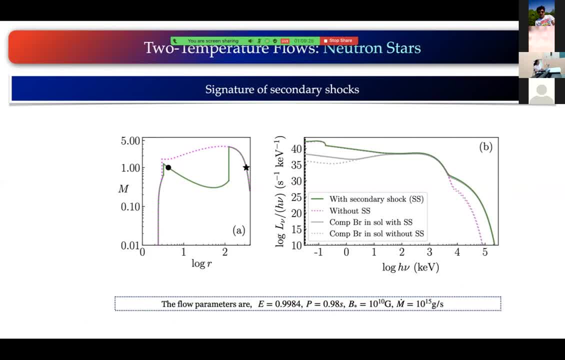 multi-day, like more than one day, and second is that, but these are steady state solutions, so, yeah, so, even if you stability analysis of the stability solution, if you perturb it, then it might be. actually, i have uh done the stability analysis of these solutions and i found that, uh, in context of the entropy, 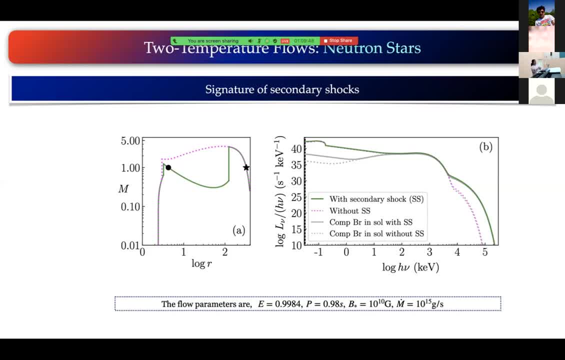 thing because there was many degenerate solutions. so for that i studied the stability of the maximum entropy solution and i found that all the solutions are stable, but the most stable one was the- uh, highest entropy solution. so the stability analysis from the earlier like things like yeah. 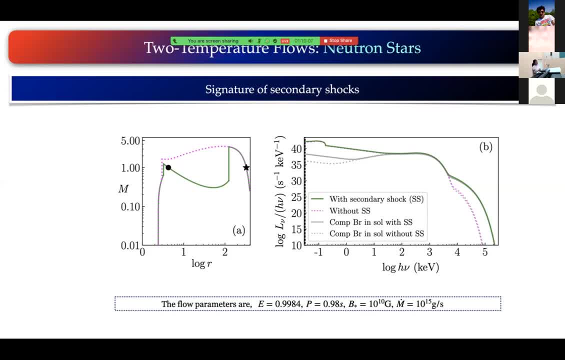 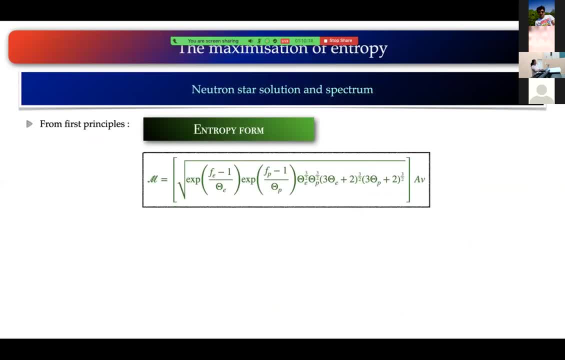 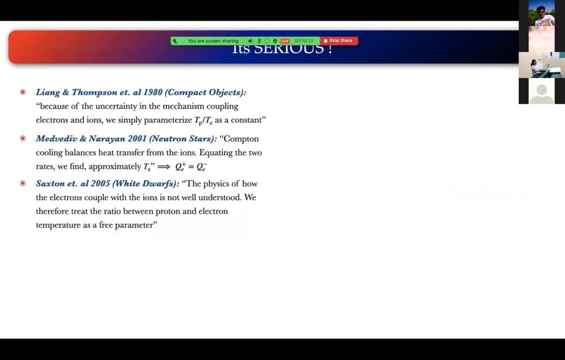 nature prefers the maximum. and second was that, uh, generally earlier works what you mentioned rightly, that they have only considered the push of region, which has been modeled as a parallel atmosphere. yeah, but you are considering the bridge of region as well, then probably a curvature curve will act. 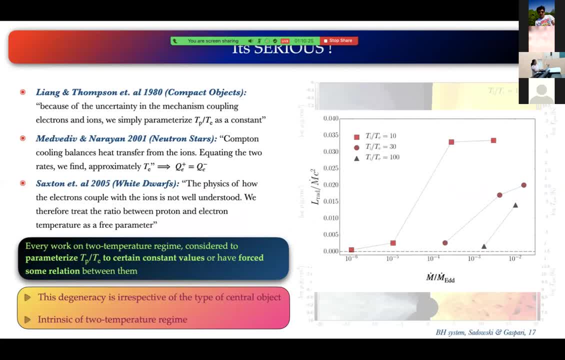 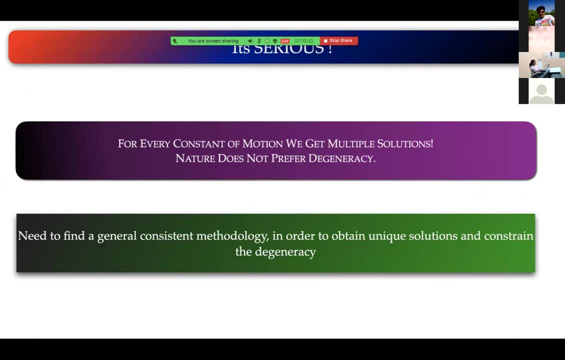 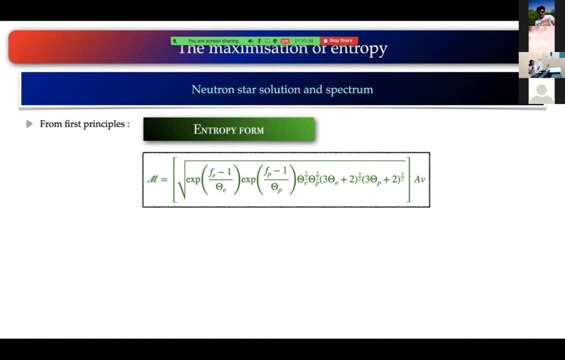 so how are you? how are you tackling it? because it's not really playing parallel atmosphere. it's not good. so it's, since we are assuming the strong field assumption, so actually the magnetic field decides the geometry. so that reduces one equation. so there is only a r theta connection, uh, which gives us the 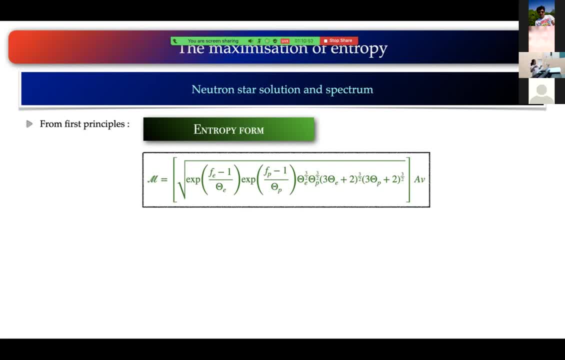 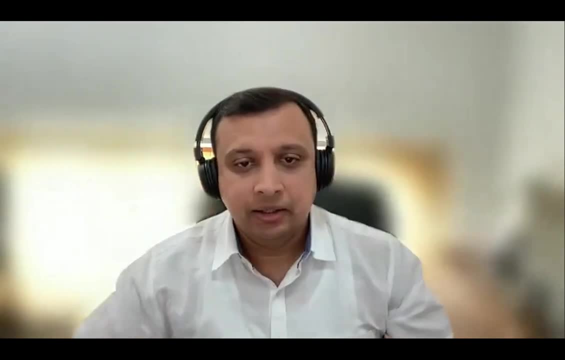 total 1d flow means that 2d, or the curvature term you are talking about, that reduces to a 1d nature. so that's why it's important to think about that. so that's why it's important to think about that. okay, uh, bhargav has a question. yeah hi, shilpa, can you hear me? yeah hi, very nice and an interesting. 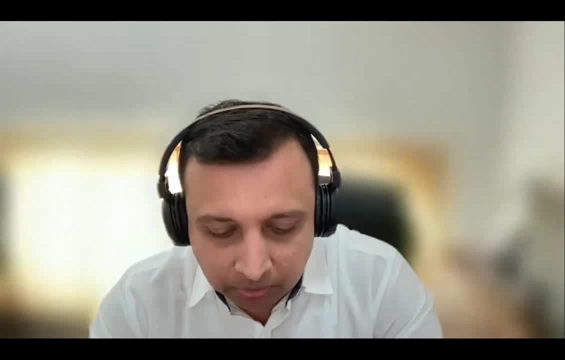 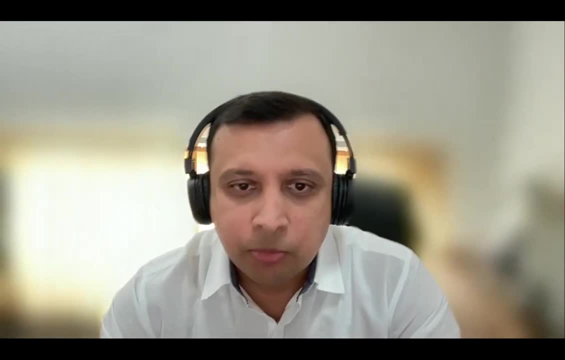 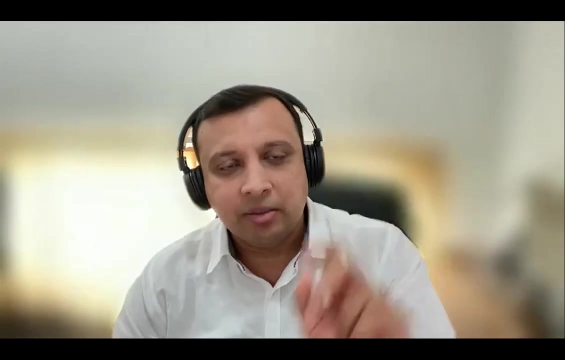 talk. actually, you rightly mentioned that. uh, usually people parameterize in ratio of proton to electron temperature. however, in your steady state calculations, since you basically start from the outer boundary by injecting some parameters and you basically go inside, and since you have two temperatures: the temperature and temperature of the temperature, of the temperature, 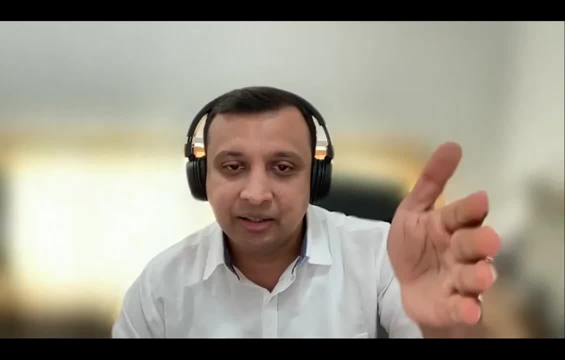 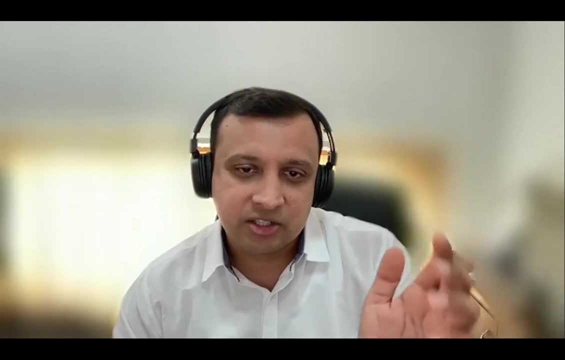 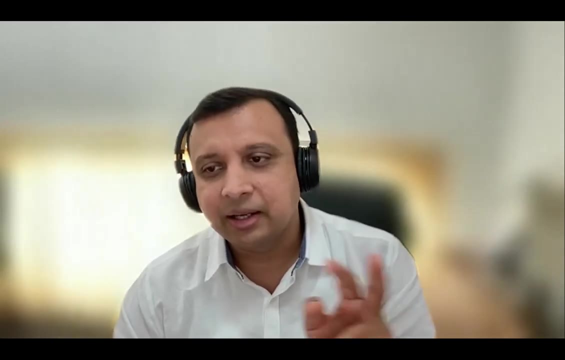 pv, you must need to enforce certain boundary conditions at the at the inner point. so how critical are those boundary conditions? because does those boundary conditions govern your formation of secondary shock? and what if? the first question is: what do you put for those boundary conditions and whether they govern your formation of the condition? inner boundary for te. 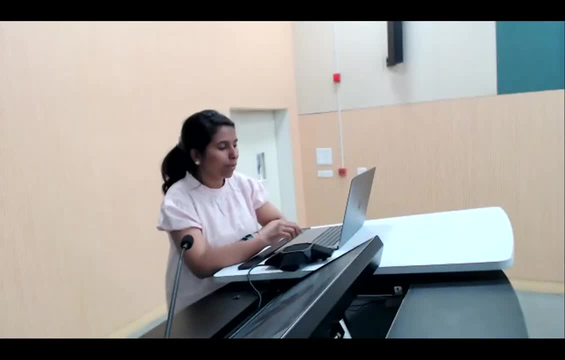 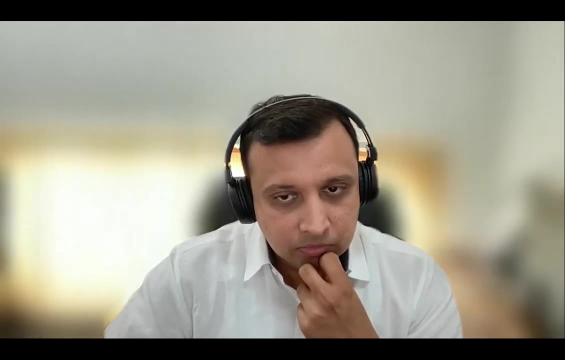 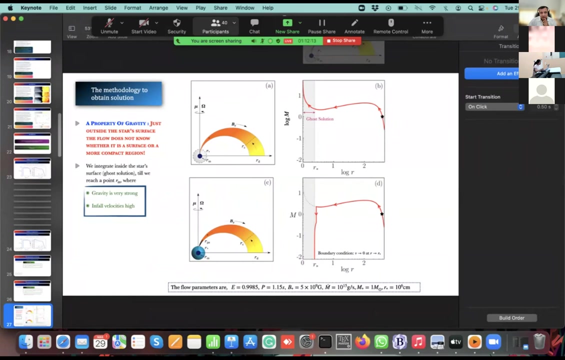 and tp. okay, so actually in the inner boundary, only we start from the inner boundary itself. so from here we start. um, um. Thank you, Hello Shilpa. Yeah, I think there is a problem here, Bhargava, can we discuss it later? 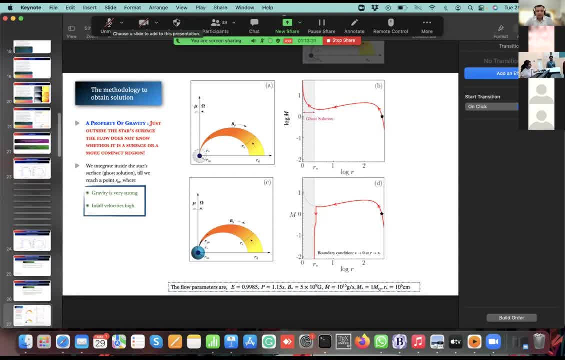 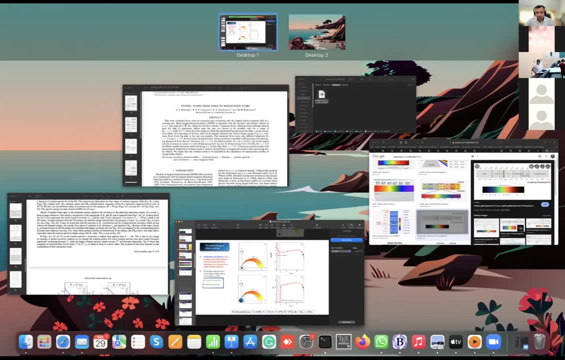 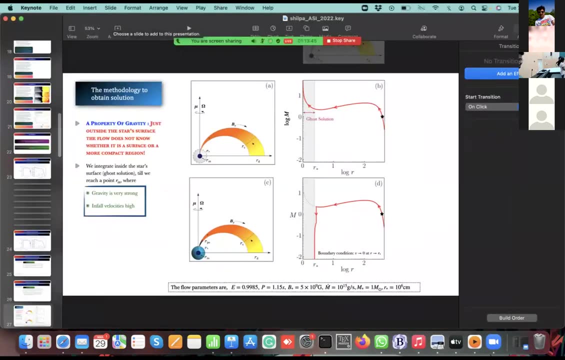 Yeah, I think it's better we discuss it later. Yeah, thank you. thank you. Are there any other questions for Shilpa? Okay, if there are no more questions, let us thank Shilpa and invite the next speaker of this session. 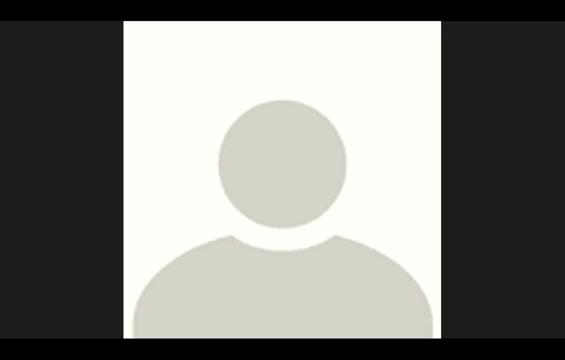 The next speaker is Zahoor Malik, So is he giving the talk in person? Yes, it's easy. Okay, So Zahoor will be talking about model-independent rate shift estimation of BL-like objects through very high-energy observations. Okay, 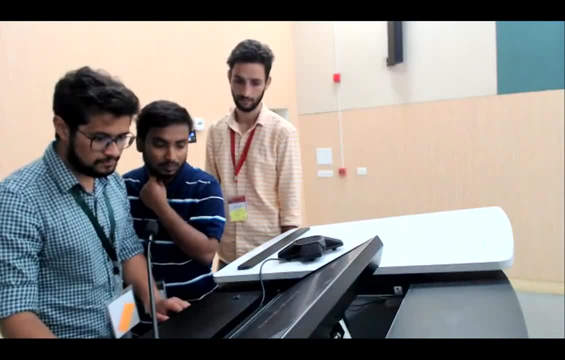 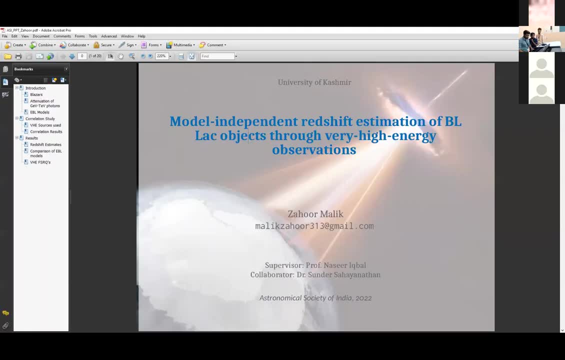 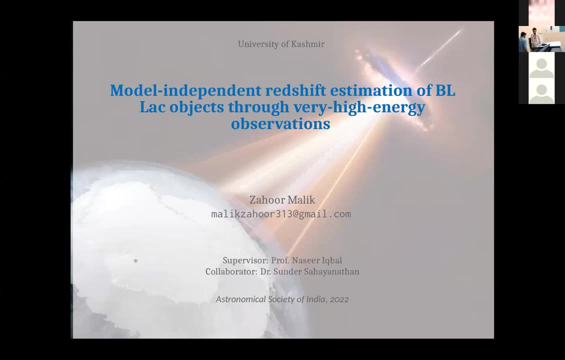 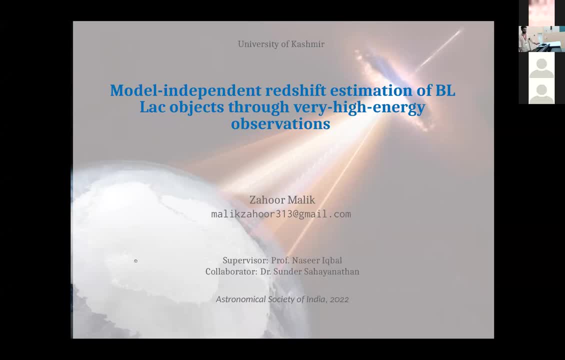 Okay, Okay, Okay, Okay, Okay, Okay. Good afternoon everyone. My name is Zahoor Malik, from the University of Kashmir, and I'm doing my work with, in collaboration with Dr Sundar Saharathan from the Baba Atman Guild Centre, Mumbai. 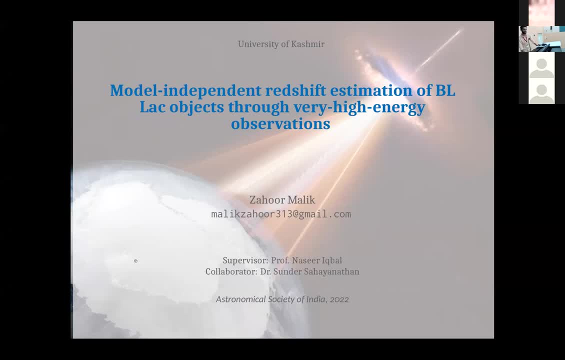 I can see the tiredness on the face of all the participants who have come back to do So. I will now try to give a quick overview. Okay, I will try to not make you feel bored for the next 15 minutes, so please bear with me. 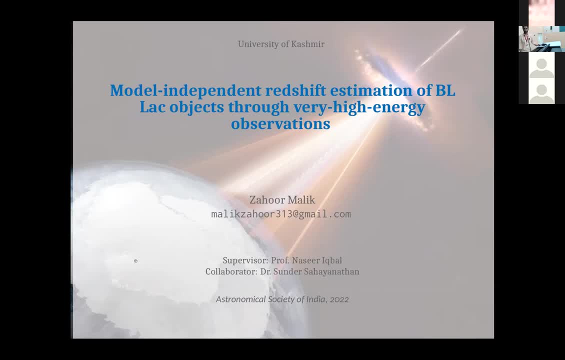 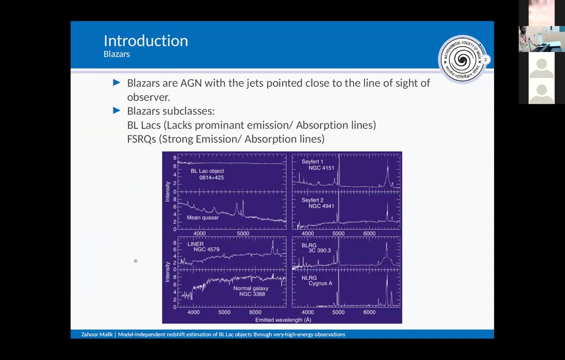 So just have a look at the title. I am going to explain it in the next slide. So you have heard about these active-objective nuclei from previous some days, so I'm not going to detail. There are this subclass of radio-loud active-objective nuclei which we call as blazers. 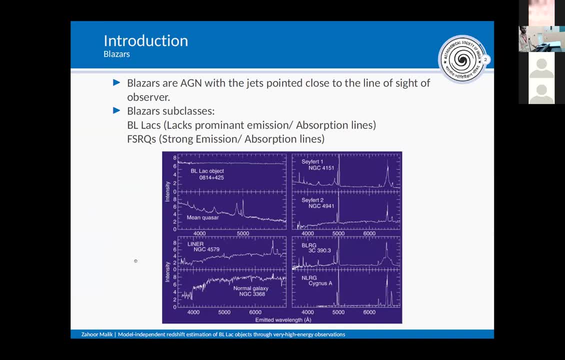 So blazers are the objects having jets pointing towards our line of sight, And these blazers are further divided into FSR cubes and BLLAC objects based on the strength of the emission and absorption lines. In case of FSR cubes, they are having strong emission absorption lines and in case of BLLAC, 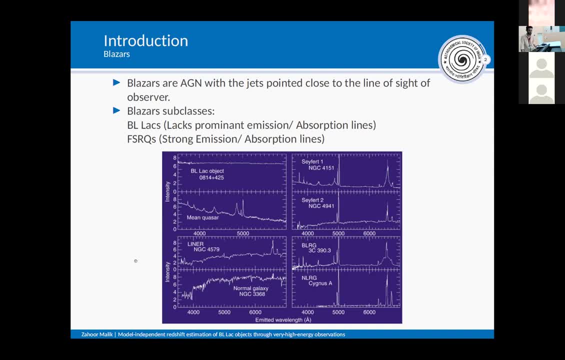 objects, they are having this emission or absorption lines absent. You can see from the left top that there is a BLLAC object here and you can see the spectrum. it is a featureless continuous spectrum. The absorption or emission lines are, as compared to other objects, they are not there. So, like this feature we use, 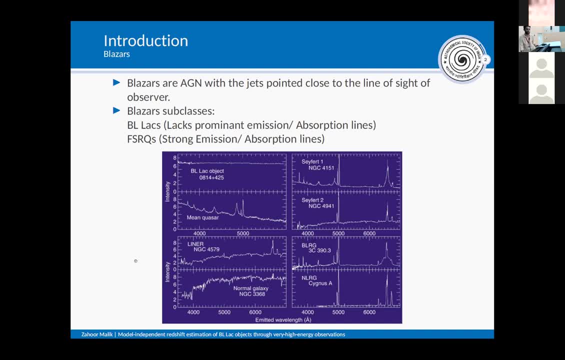 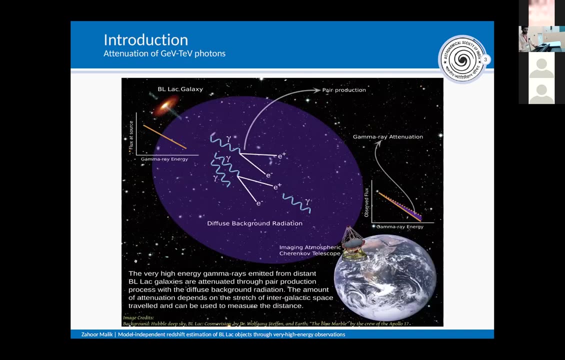 to calculate the redshift, like the distance estimation of these objects. So if the emission or absorption lines are not there, so you will not be able to. it is very difficult. So this is the main problem I have addressed in this work and how we are doing it is since 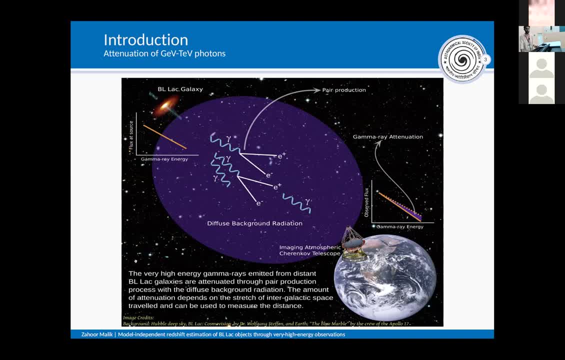 this redshift is a spectroscopic parameter. So here we are using VHE astronomy. that is a totally independent, different approach we are using from spectroscopy. What we are doing is: you can see that. consider that. can you see my pointer? 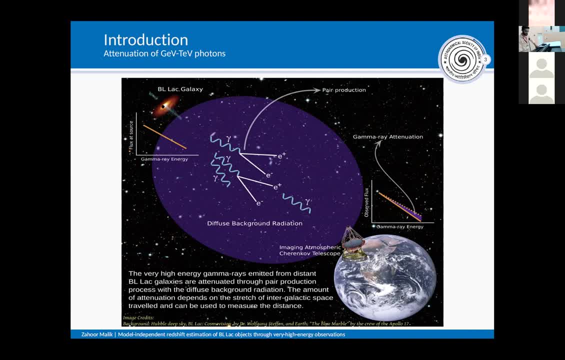 So this is a Bialik galaxy- and Jack is pointing towards us and this dark blue patch. it is a diffuse emission radiation in the universe, Particularly here it is the extragalactic background light, the second dominant diffuse radiation after the cosmic microwave background. 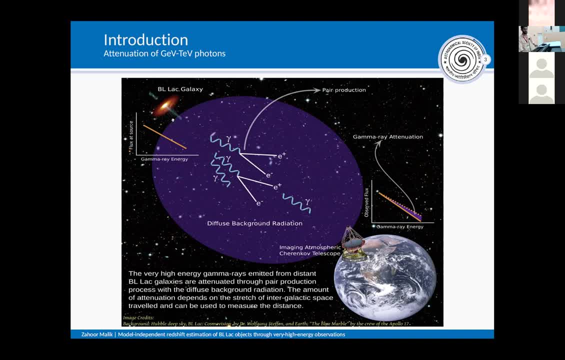 So these Bialik galaxies? they are sources of VHE photons in the universe. So what happens is this: the photons, they are the sources of VHE photons. So what happens is these photons, they are the sources of VHE photons in the universe. So what happens is these: 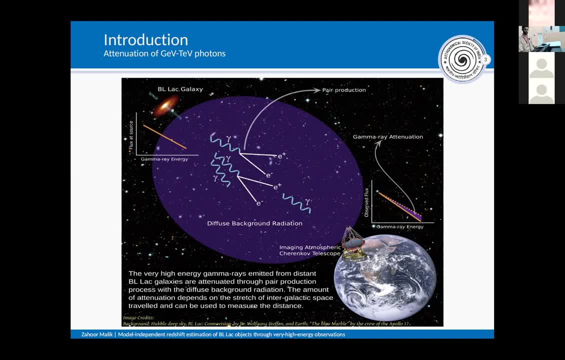 photons, the VHE photons, come from this Bialik galaxy and they interact and root with this extragalactic background light photons and PR production occurs. So the spectrum will change. For example, here it is the source spectrum. it will be without attenuation from. 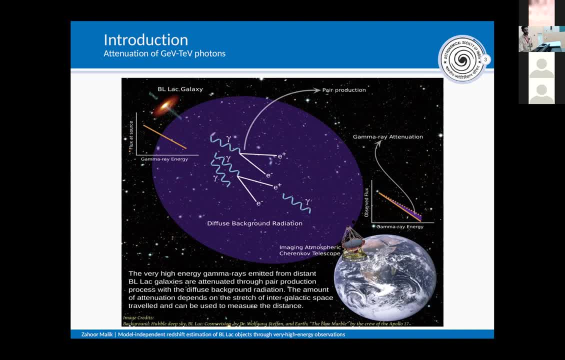 extragalactic background light and what we are collecting here is the observed spectrum which will be after the attenuation. So the spectrum, for example, if it is having some slope here, the index, here it will steepen up because of the attenuation. here you can. 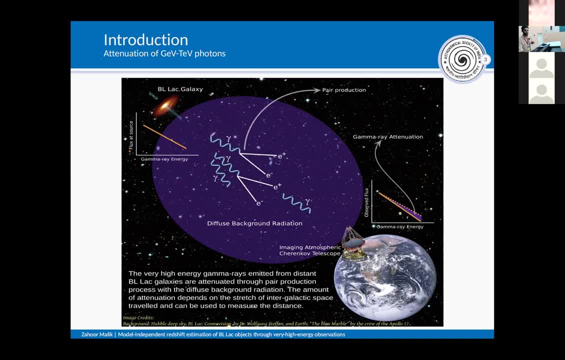 see. So it will steepen up because some of the photons will be attenuated And this feature we are using to calculate the redshift, how I am going to present in next slide. So there are two problems here. First problem is that we do not know the intrinsic spectrum. This 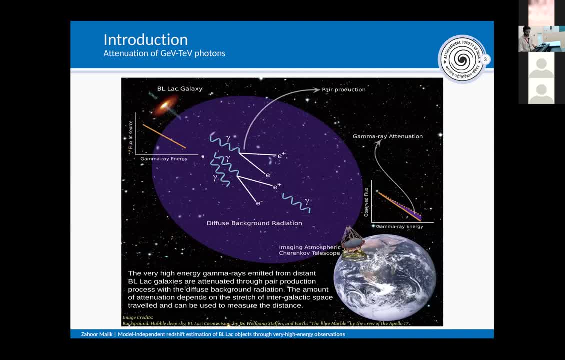 intrinsic spectrum we do not know. and other thing is we do not know accurately the this amount of EBL which is present, Because the direct estimation of EBL is less than the direct estimation of EBL, is hindered by the foreground emission from our own galaxy. 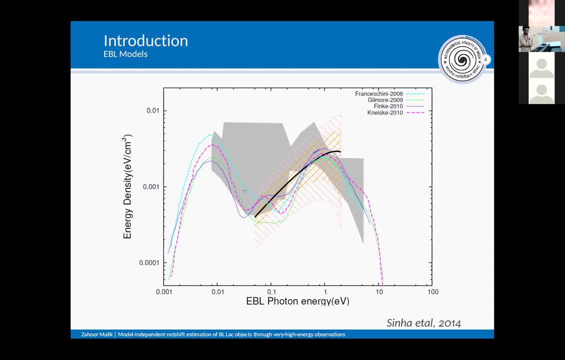 So and so, since I told you that this is hindered by the foreground emission of our own galaxy, So we are going to the cosmological models, EBL cosmological models. You can see these lines. these are different cosmological models which are giving us the EBL amount of EBL. 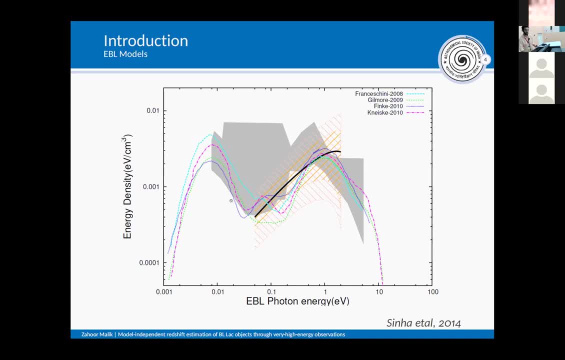 which is present in the universe, And in this work, like I am addressing this, like on the right hand side. So the EBL is present in the universe and in this work, like I am addressing this, like on the right hand side, And in this work, like I am addressing this. 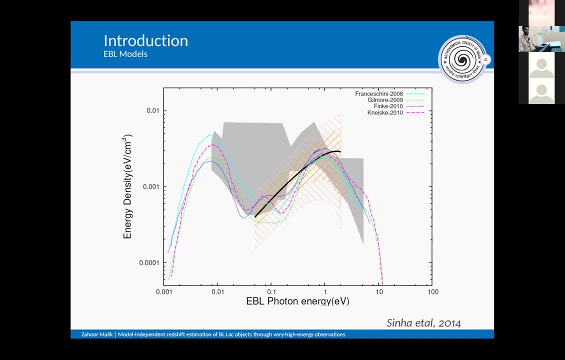 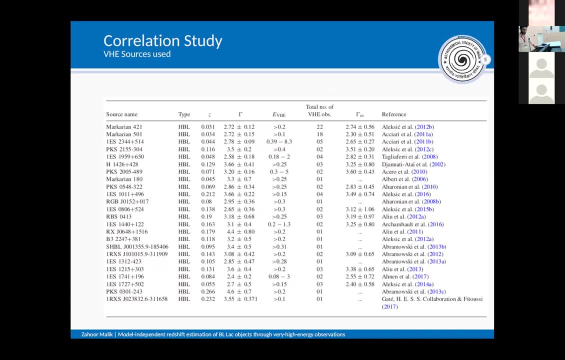 side And in this work, like I am addressing this, like also how valid they are. So these EBL models are based on some approximation assumptions. I am checking that also in this work. So the study starts from here. we have taken all the sources which are detected. 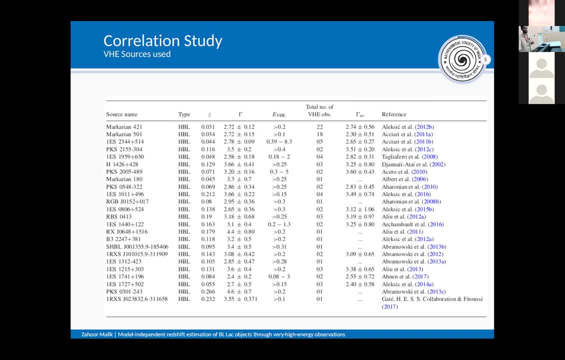 at VHE, Okay, and which are having certain redships, And I am checking a correlation with the index, spectral index. I told you before that spectral index should be straightening information. I am taking from EHC, from these tables, I am taking from nutrition and I am 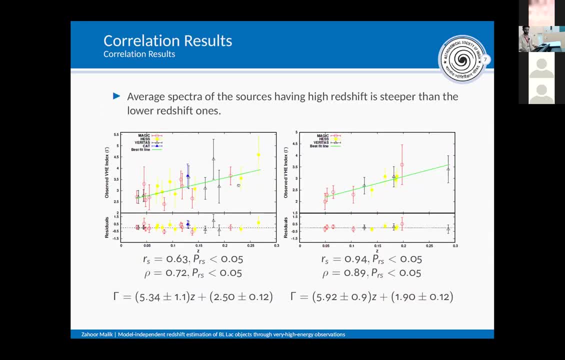 checking the correlation for all the sources. The first plot on the left side you can see this is for pure HPLs, energy picket places- and you can see that there is a nice correlation, although error bars are very high. but you can see that there is a nice correlation and see for the sources. 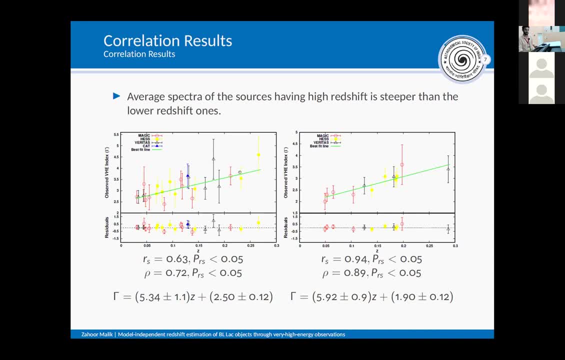 which are at higher redshifts. the indexes are higher. that means the spectrum is steeper. okay, and for EHVLs, extreme initial loss. you can see that there is a nice correlation here and these are some correlation parameters. you can see for both we are getting a nice correlation and where 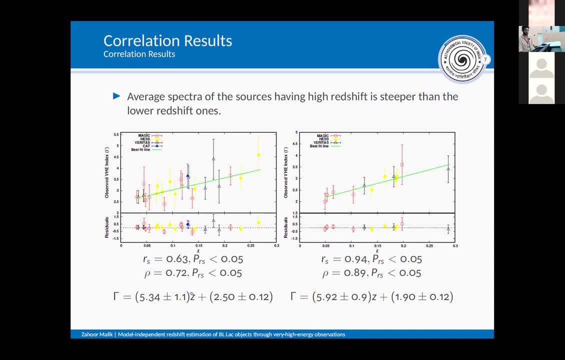 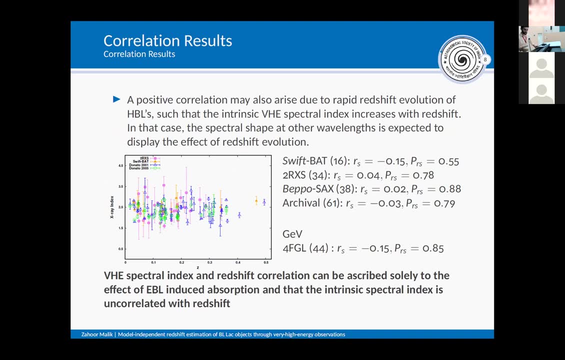 we have fitted a function to get the signature. So this signature we are telling it is because of the extra galactic background light on it. okay, to cross check this. what we are doing is we are checking it, like for the other wave bands, because we want to see. 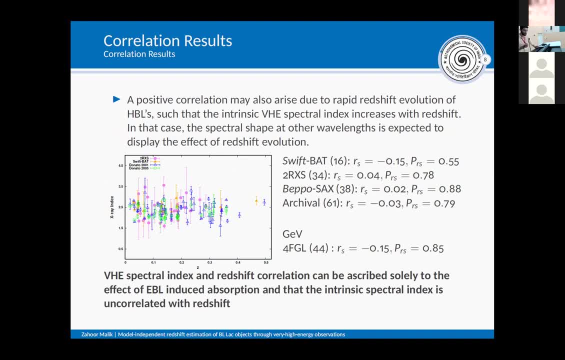 is this because of the evolution of the inverse? it can be due to the like intrinsic spectrum can be related to the redshift. for that case, we are checking with lower view bands and we are checking for x-ray and low energy gamma rays. here we have used four catalogs: x-ray catalogs and one of four. 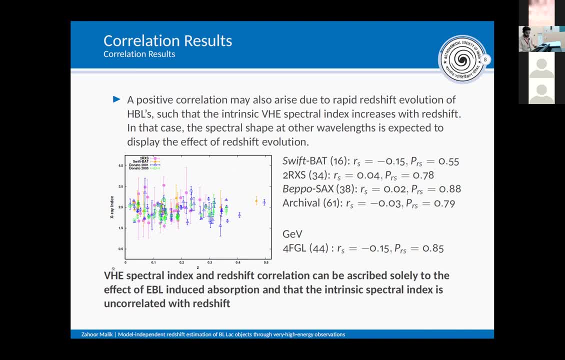 FGL catalog for low energy gamma rays. we see that there is no correlation at all and you can see from the plot also that correlation is not there. so that further assertions that the correlation in VHE is because of the extra galactic background light and we are checking for X-ray and low energy. 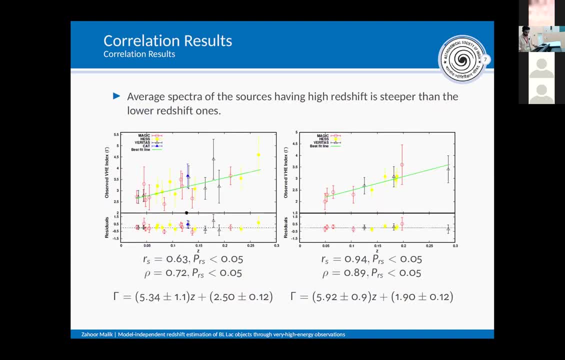 gamma rays and the function we fitted here. this function is a simple approach, but see like this can be used without any. you can use it anywhere if you know the index, if you know the spectral index, and using this function, you can get the redshift at any, any, any index for these sources. okay, so, 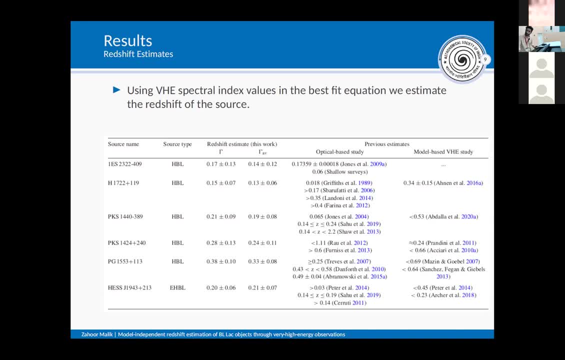 using this best function, best fit function. we have a Redshift of six super sources which are there and they are having the some previous estimates, also some spectroscopic estimates like upper limits and all see. you can see here that industry, like InSpite, our approach is totally different but still our estimates are matching with the. 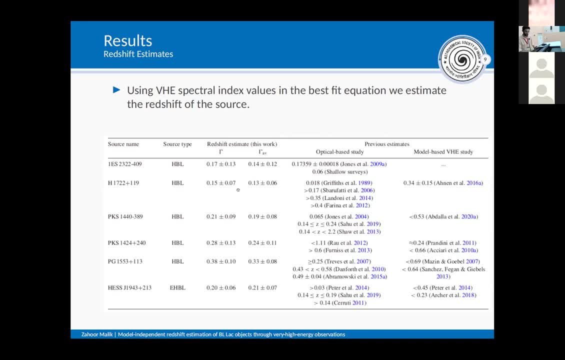 previous estimates. okay, I want to add here that I told you before also that is the spectroscopic parameter. redshift is a spectroscopic parameter. we are calculating it here using the VHC astronomy And certainly our estimates are matching with them. You can see, these are the previous works. 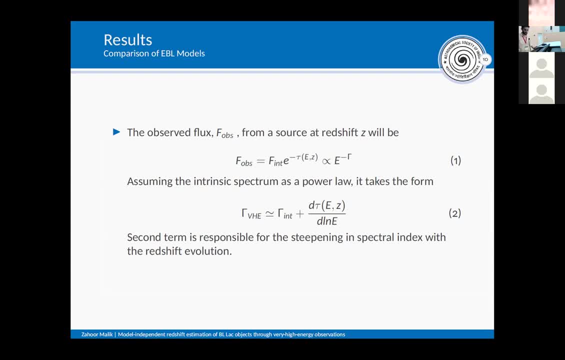 And the other part of the work is I am checking the validity of the EBL models. We know that the observed spectrum is given by fluxes, given by the intrinsic, And this is the e raised power minus tau factor is from the opacity due to EBL. 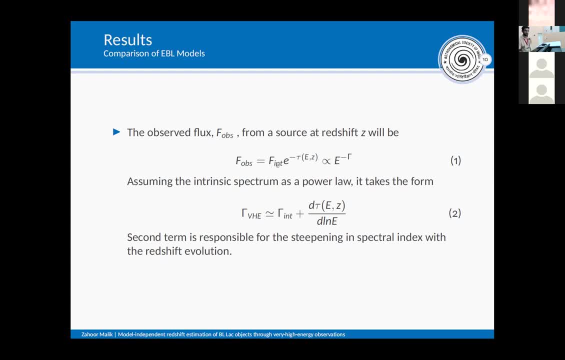 And here we consider the intrinsic flux is the power law, because this is an observational feature only. So we are seeing that most of the sources are having this power law behavior in VHC And we are considering intrinsic flux as power law also. And then we reach here that observed index. 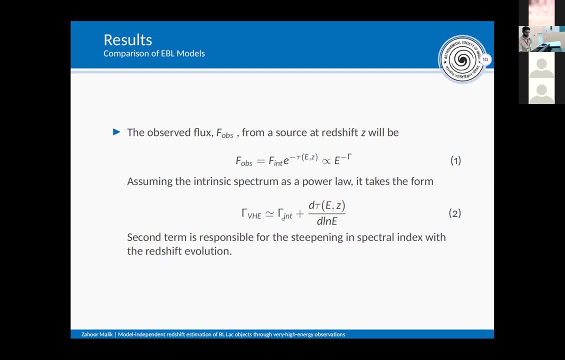 will be given by the intrinsic And this is the tau by delawney factor, which is the opacity factor. So I told you before also that we don't know the intrinsic spectrum And this tau by delawney. we are using cosmological models. 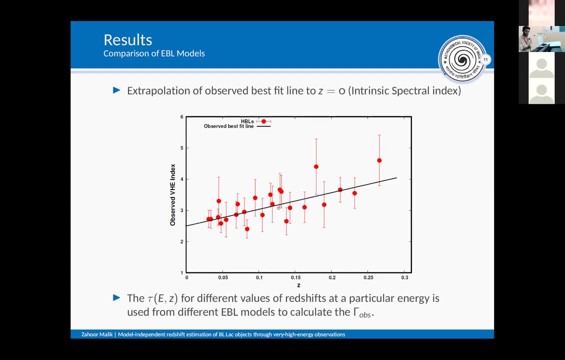 For this first term. What we are doing is we are extrapolating that best fit line to z equal to 0,, redshift to 0. And y at 0, you will see that the distance will be minimum And we are going to the source to measure. 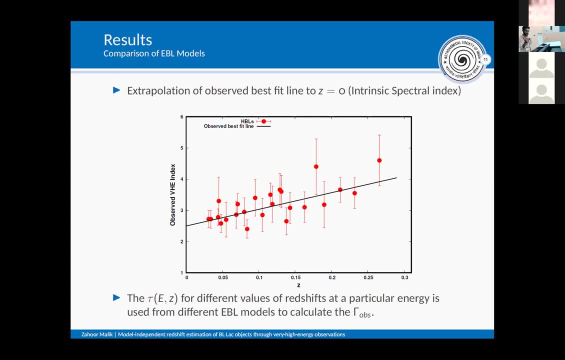 That form is the intrinsic index. This is the assumption we are extrapolating, we are using as an assumption And that intrinsic we are getting from the index And the tau values we are taking from different cosmological models And we are comparing with the observations. 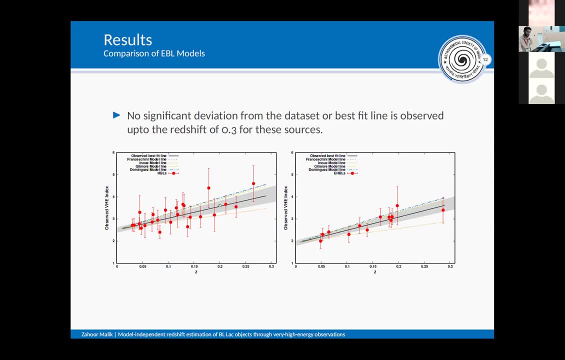 Here you can see that This black line is the best fit line And these different colored lines. they are intelligence also. You can see these are some different cosmological models. You can see up to 0.3 redshifts in both for HPLs and HPLs. 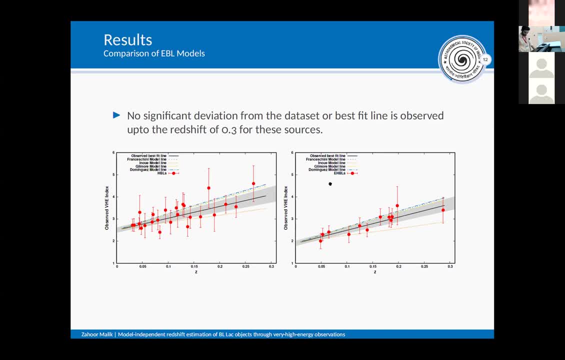 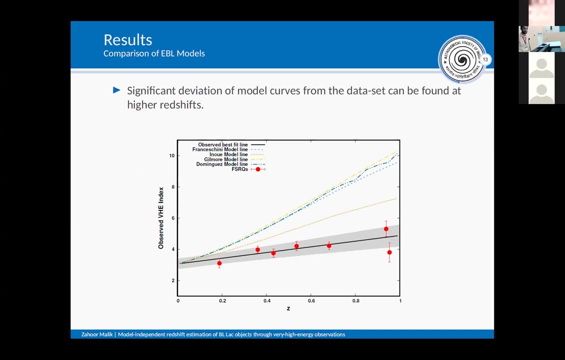 You can see that models fall within these error paths. And to check the behavior of these EBL models that have redshifts, what we have done is we have taken FSR clues. There are only seven FSR clues detected in VHE. 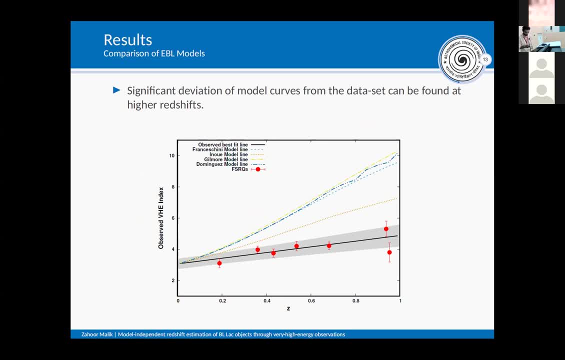 And I have taken FSR clues. I am going to talk about that also. So you can see that these- although number of sources are very less, but you can see that these models deviate quite significantly. So here at higher redshifts, 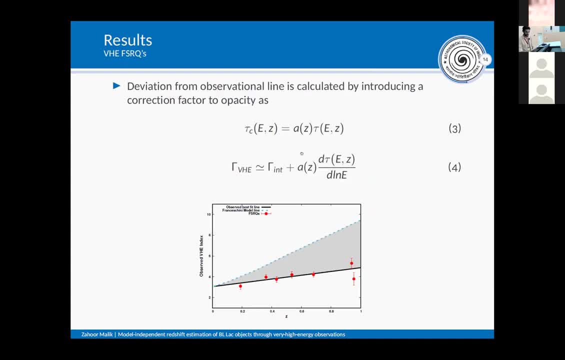 What are we doing is we are calculating this deviation. We are adding a correction factor to the existing EBL model so that the model line here, the model line- it comes to the observational line. We are including this redshift dependent, this correction. 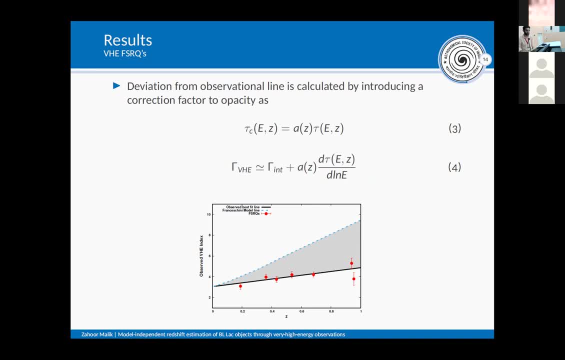 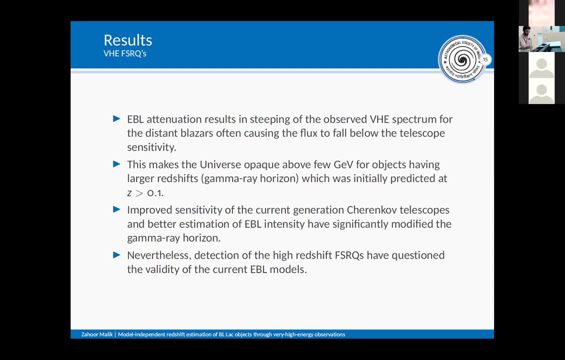 factor here And we are updating that EBL model, existing EBL model. We have used a recent EBL model And this is the last thing I'm going to talk about. is that this EBL, since all these EBLs, what our work is. 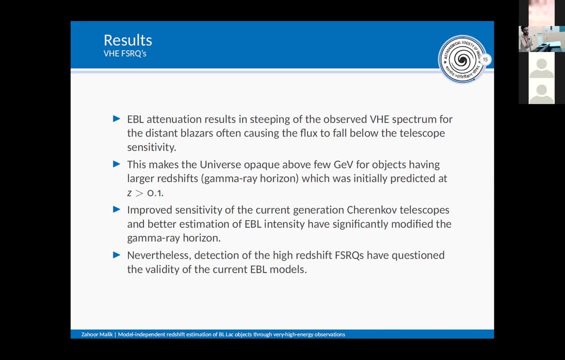 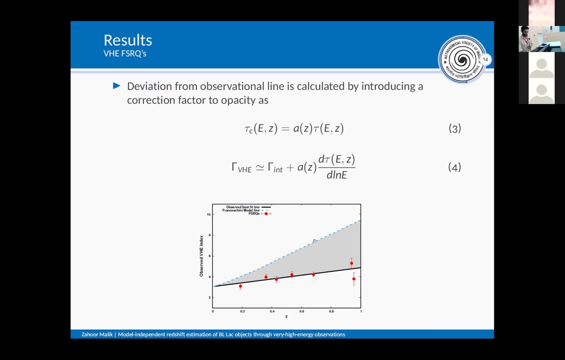 saying is the EBL is less as compared to what we are estimating using these EBL models models. You can see this from this line: the EBL is more using this model and our model is very less Because of this EBL like high EBL. what these models say that we cannot 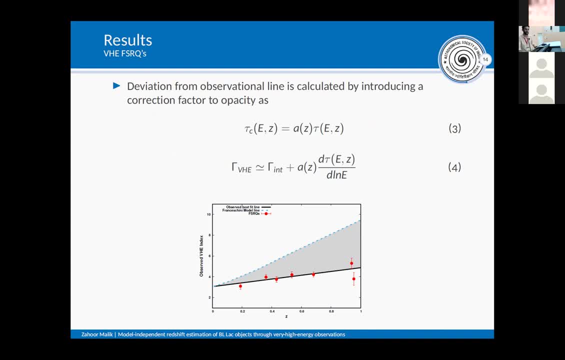 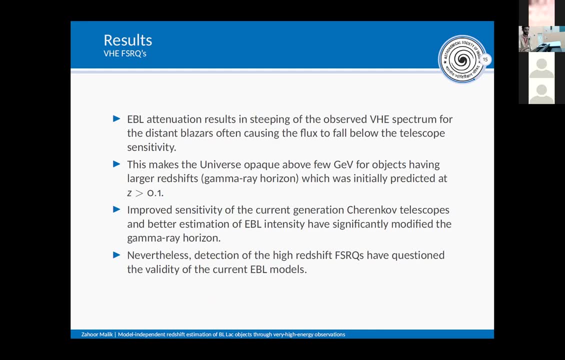 see the sources beyond some redshifts in VHE. That makes the cosmic horizon and that I am explaining here. Before it was 0.1, redshift was 0.1 that they were saying we cannot see after 0.1.. Nowadays it is updated because of some recent instruments in VHE, but it 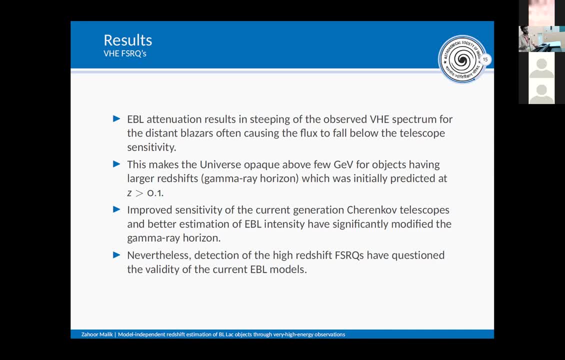 is settled. But we have found the FSRQs which are detected at like 0.9 redshifts. that itself talks about these models, how they fail at higher redshifts. So we have updated and we have taken care of the correction using observations and we are using that updated. 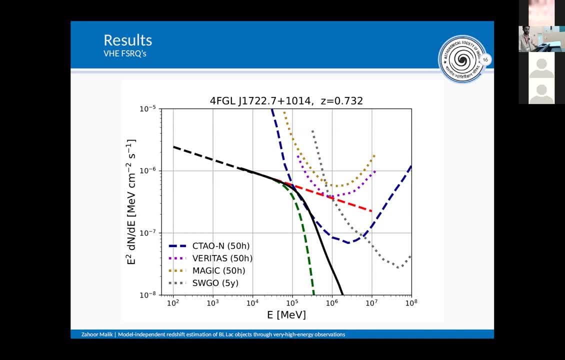 EBL and we are seeing for FSRQs which all we have taken All the FSRQs which are detected till in from the Fermi catalog. we have found that there are 744 FSRQs which are detected at Fermi And what we are doing is we first should. 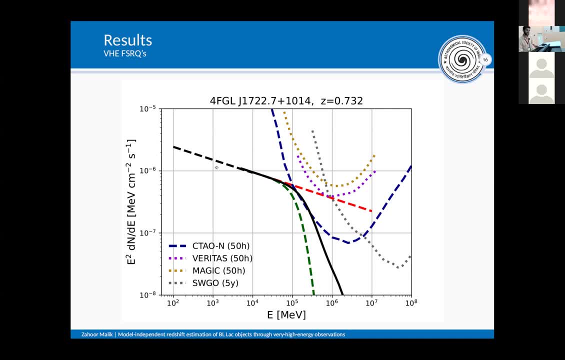 know the intrinsic index. We are making an assumption, we are extrapolating the intrinsic spectrum from the Fermi towards VHE And then, since this is the intrinsic index, we have to make the EBL correction. and we are making the EBL correction using our updated EBL model. 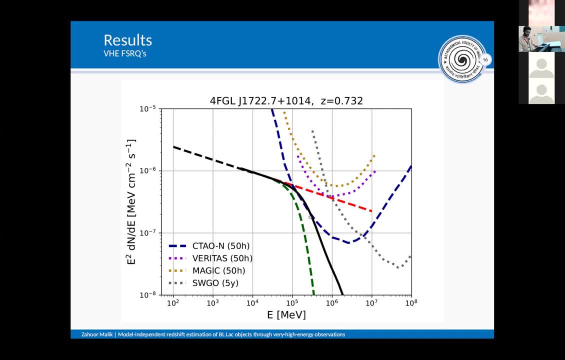 As well as the original EBL model. You can see here clearly that this black line is our EBL model, which is saying that EBL is less as compared to the original model here. And then we are over plotting the different sensitivities of different telescopes. We are actually checking. 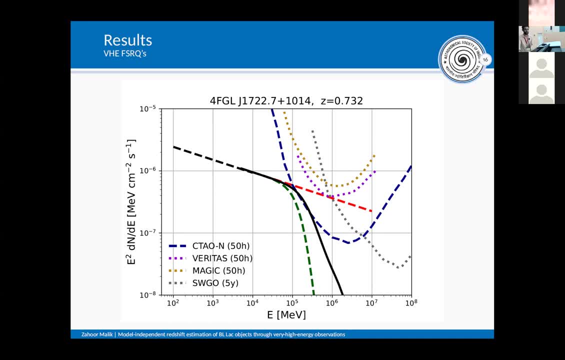 for the possibility, detection, possible detection of these sources, because these ICTs are pointing telescopes. You have to be sure like which source can be detected. So you have to point that telescope towards that source. So you have to be sure like which source can be detected. So you have to point that telescope towards that source. So you have to be sure like which source can be detected. So you have to be sure like which source can be detected. So you have to be sure like which source can be detected. So, after over plotting the 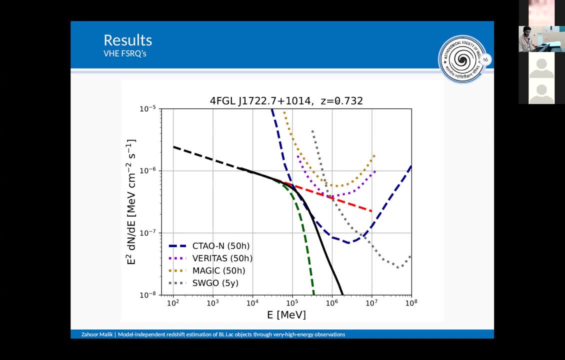 sensitivity curves of different telescopes. you can see these sources at redshift 0.7.. And the original EBL model- this green dotted line- says this cannot be detected, but our EBL model is saying that this can be detected by the upcoming CTA And we have checked these. 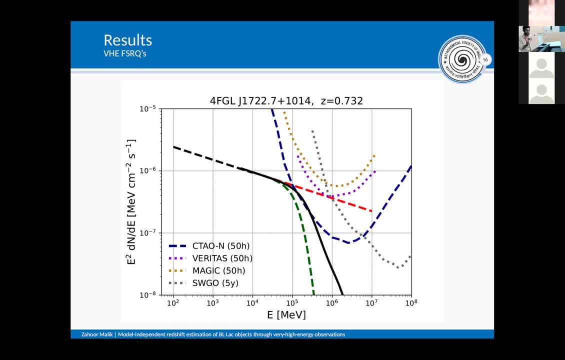 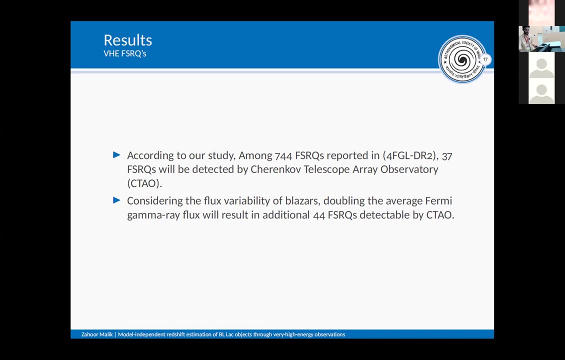 results with the existing 9 FSRQs which have been detected and we have seen. our results are favoring. So all the 7 that can be detected with the telescopes. that was the cross-check of our work And among 744, we have seen that there are 37 FSRQs that can be detected by upcoming. 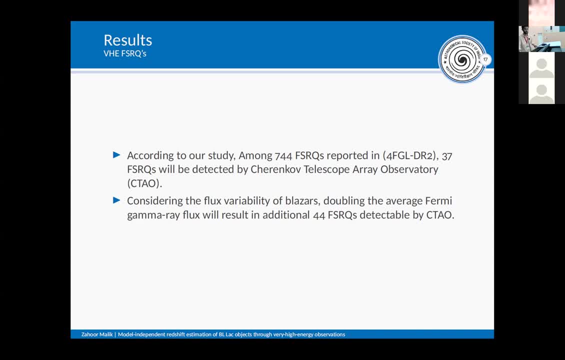 Chern-Kau telescope array And since considering the blazers are very like, they are very variable objects, so sometimes the flux becomes 10 times also. so we are considering here in a situation where the flux doubles, it becomes two times, and in that case there are. we found that 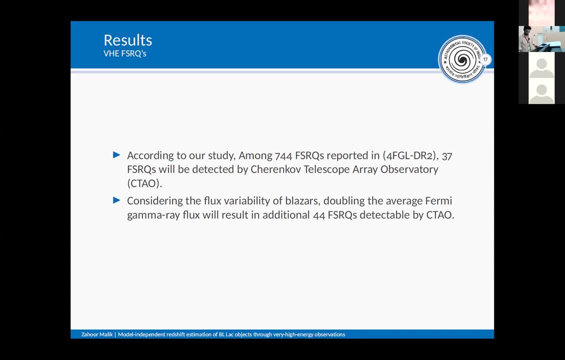 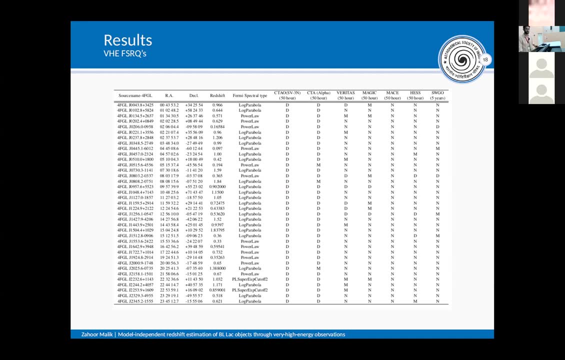 there are 44 additional sources which can be detected by cta, and here we are preparing the catalog for the cta and other instruments. interestingly, we have found that some of the sources can be found by the existing icts and we are publishing this work so that we can cross. 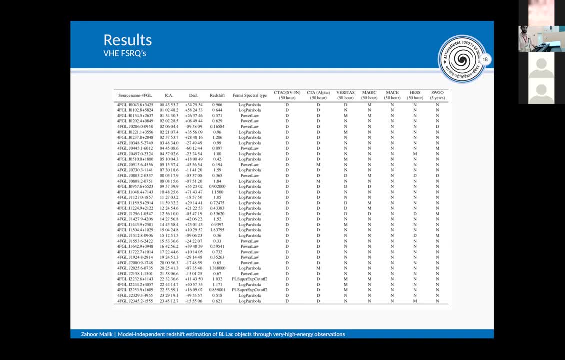 check that and, to summarize, we have like we have used a novel approach to estimate the redshift of objects alternative that is a good alternative to use and we have made a catalog for fsr that can be detected at vfc using icts. thank you so much. 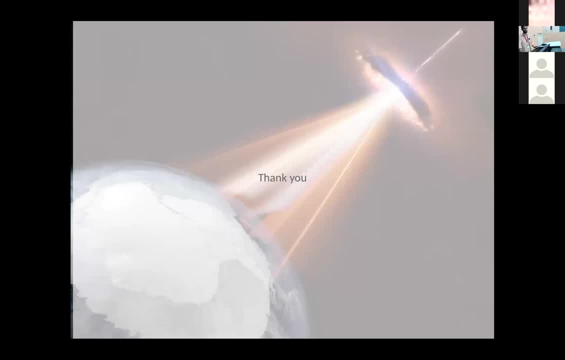 thank you, zahur. any questions for a stock? uh, hi, uh, so you uh like uh develop your own eagle model and you try uh that model with fsrq uh, but in case of blx sources, is uh i think high frequency blx sources you have used, but uh, 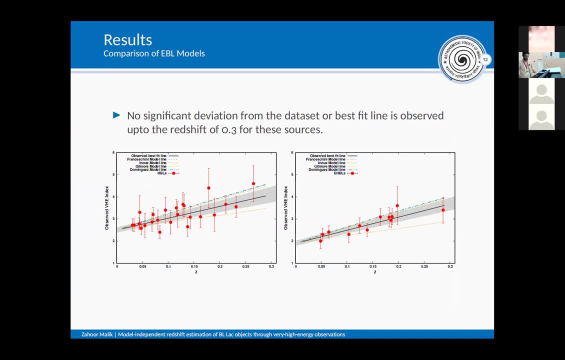 you didn't try that model with hdl sources? yeah, you can see here i was seeing that the existing evn models- they are below, like for blx. you have seen that fsrqs are mostly detected at headships like: uh, i don't know the exact reason, but it is there. it may be because of the evolution or malpest. 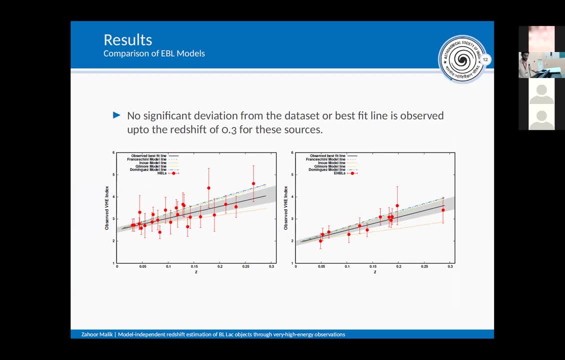 bias. but you can see before 0.3 redshift that these models are behaving well. they are falling within the error bars and they are falling within that, uh, slightly within that error band, one sigma error band. that's why. but here you can see they're deviating from the error band, that's why. but here 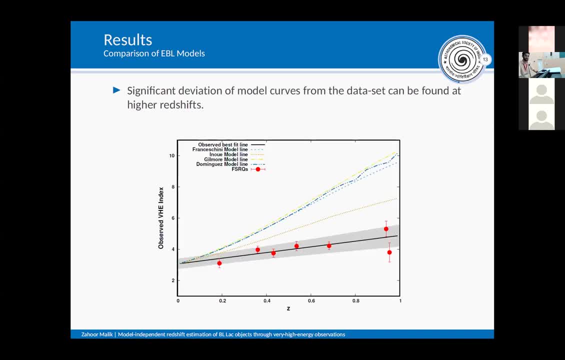 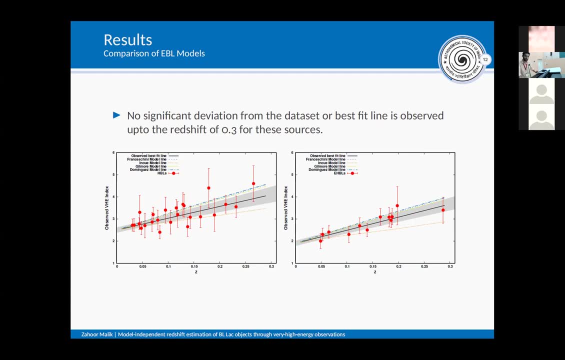 you can see they're deviating from the error band. that's why. but here you can see they're deviating much so that's why we try to have a circuit. have you tried with blx like this new model? yes, we have tried the new model in blx also and we found i have not included that slide. 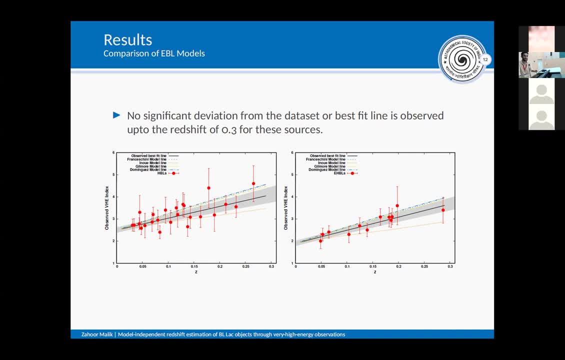 yeah, and that abl model is falling well inside that one sigma, so it it is falling. if you yes, since the abl model is uh. we have uh done that using observations only, so it is mandatory that it should fall. we have uh done that using observations only, so it is mandatory that it should fall. 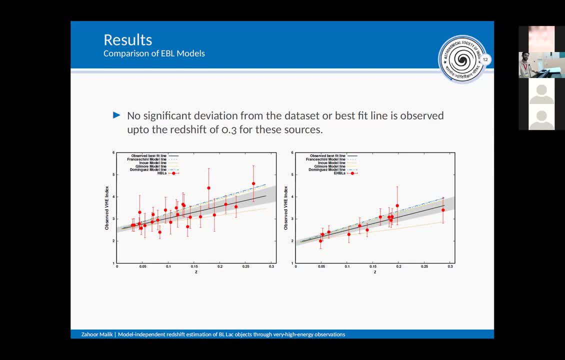 like it's uh like both for hbl and fsl. both it's applicable. yes, yes, thank you. one question from punkage, uh, nice work. so i just want to ask. one thing is like there was some issue with the ebal estimates event that are existing right now. 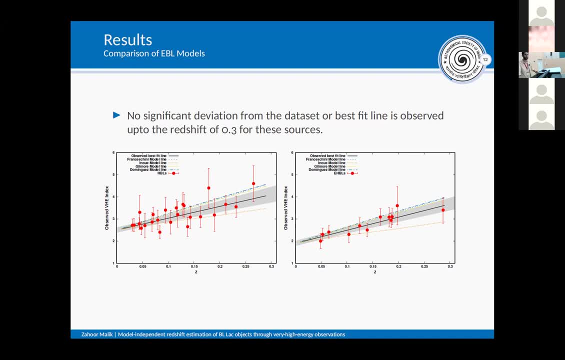 because of which people propose that this, uh, astroparticle physics, people propose the axion like particles and basically we expect ebls, we expect ebl, but we were getting lesser attenuation. so how does this model i mean? you are saying that, okay, you can detect sources up to higher rate. 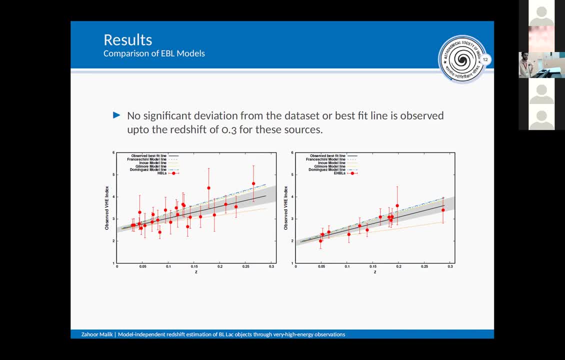 shift right compared to the what is? the existing model is yes, how does this goes with that? those proposed axia, axion like particles scenarios, see they also propose less ebr, like the way your model, i think, is predicting less abl compared to what it is. okay. see, uh, here, this abl model where, uh, we are developing it from observations only. okay, 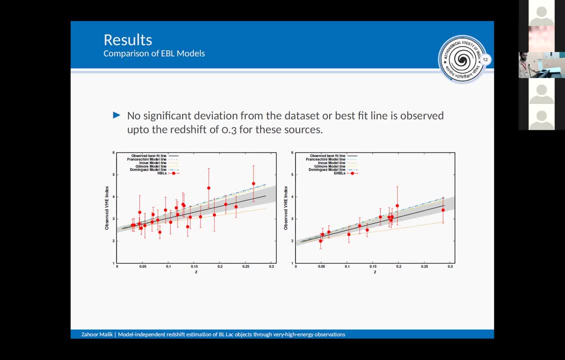 frankly, i will say i don't know much about exam, what you are talking about. but this is totally based on observations and after cross checking we are finding that this abl model- uh uh for the existing, like fsrc. we have checked this and this ebl model works well and it is. 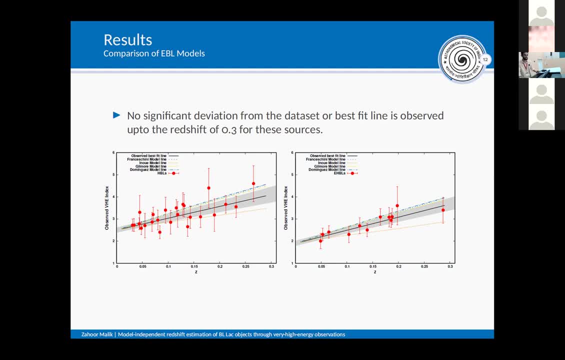 showing that ebl is less only yeah, okay, i mean, that was also the claim. actually, what, observationally i mean earlier? uh, this was exactly the reason that ebl is less compared to what is predicted or what is expected, and that's why the proposal- proposal for this new particle- was there. but okay, 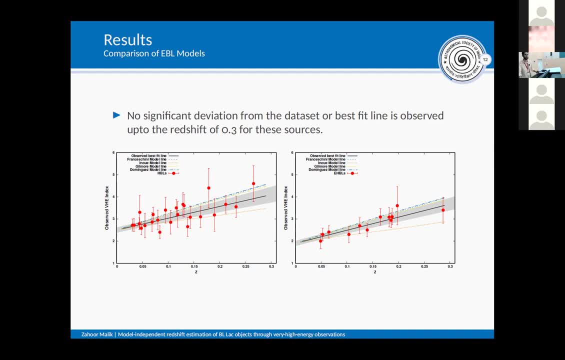 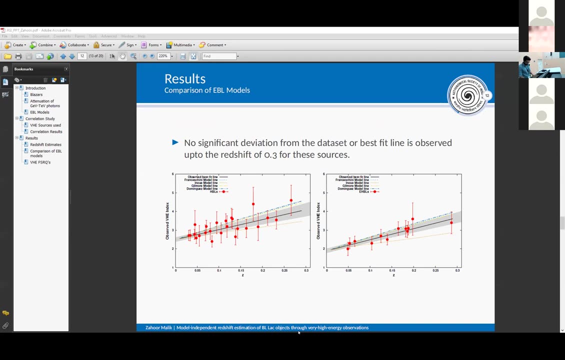 yeah, thank you. okay, thank you, okay, thank you. let us move on to the next talk, which is the last talk of this session, and the last talk will be given by rajesh. he will be speaking about the type 1b supernova sn 2017. iro a- moderately. 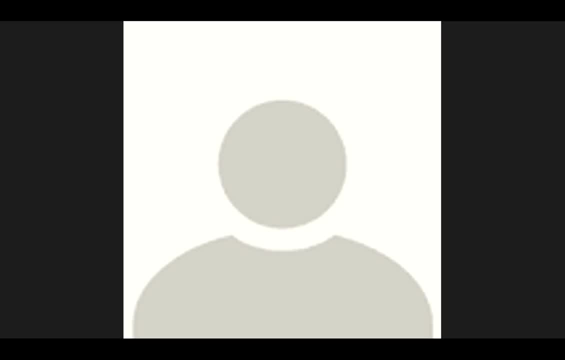 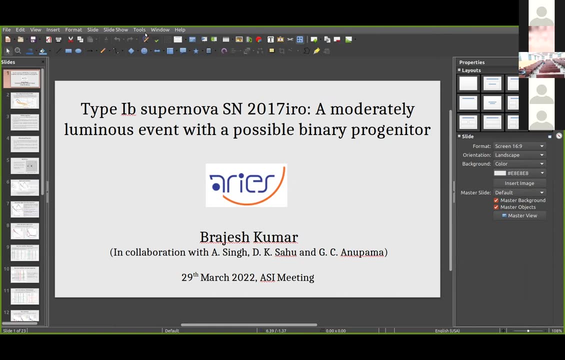 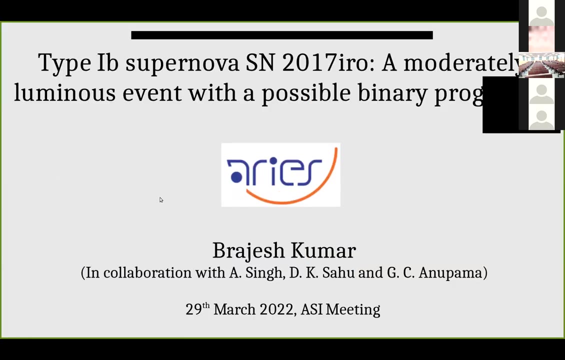 luminous event with a possible binary progenitor. so, rajesh, you will please share your screen. it is fine having whatever. yeah, a little louder, please, hello, hello. yeah, rajeesh, you can start, okay, thanks. so, uh, hello everyone. uh, good afternoon. so this is uh, since this is the last uh talk. 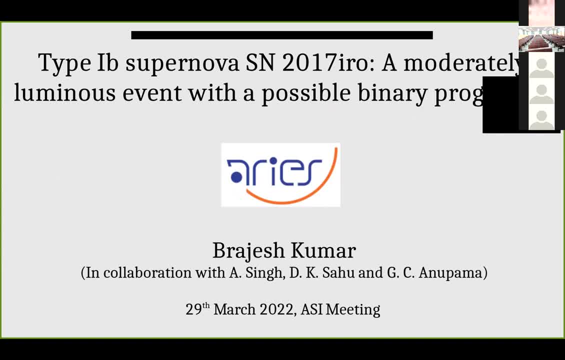 of the session, so i will try to finish my presentation timely. so this is the title of my presentation and this work has been uh taken as a provenania inance. so, ALLAH RAB, smoothen the phenomena. THANK YOU are done with, in collaboration with abhinash singh dk sao and gc anupama so. 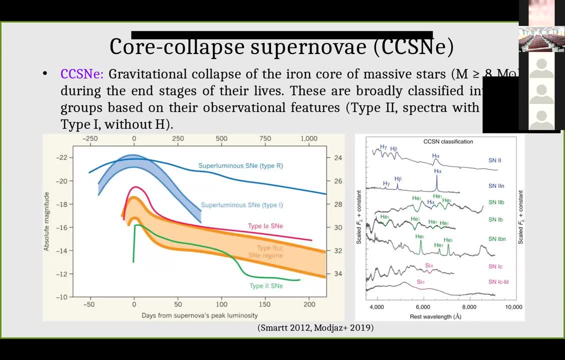 before i go further, let me briefly introduce you about the core collapse supernovae and their progenitors. so just wait it okay. so core collapse supernovae are the gravitational collapse of the iron core of massive stars greater than eight solar masses during the in this stage of their lives, and 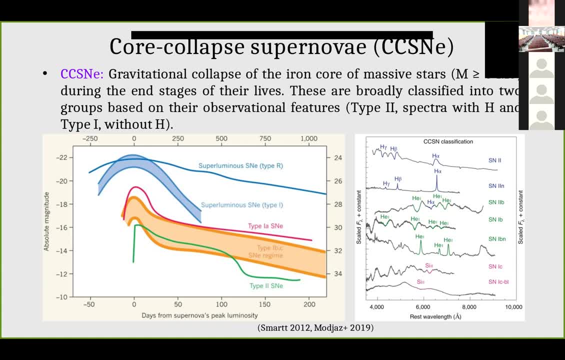 these are broadly classified into two groups based on their observational features. so type two with spectra, their hydrogen in their spectra, and type one without hydrogen in the spectra. so in the left side up here- this figure- you can see that the light curves have diversity and in the right panel the spectral classifications are presented. so you can see that in type two 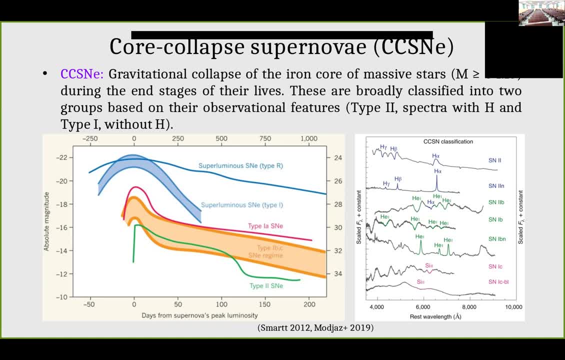 events, hydrogen is very strongly present and in type one events hydrogen is absent, but there could be a presence of helium features mainly in type 1b, type 1b and type 2b and there is another class, type 1c, and broad-line type 1c were. 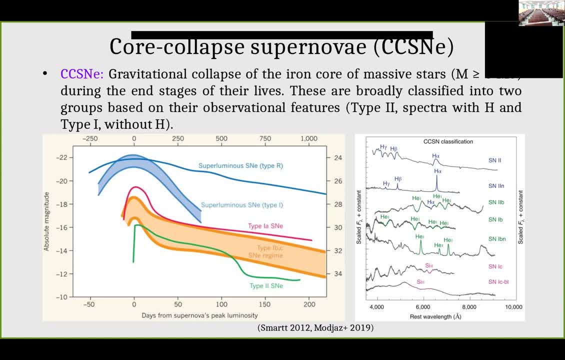 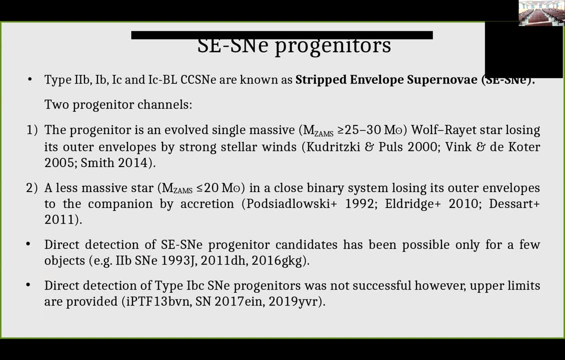 both hydrogen and helium features are hablax en, but strong features of silicon is present. so actually the type 2b, type 1b, type su-one and type 1C broad-Line core collapse region supernovae are also known as strip enveloped supernovae because they are progenitors strip 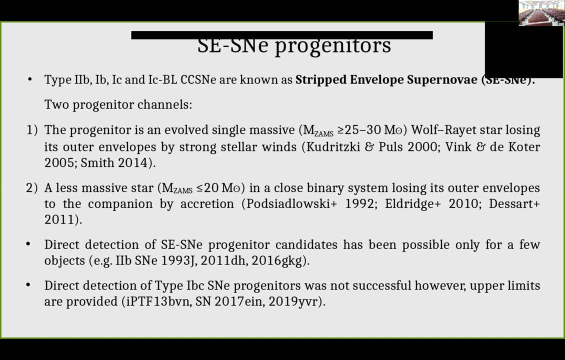 of the outer envelope before the explosion And it is believed that there are two progenitor channels of strip enveloped supernovae. So one first is the progenitor with evolved single massive star greater than 25 solar masses, Ruprecht stars, and these are losing their 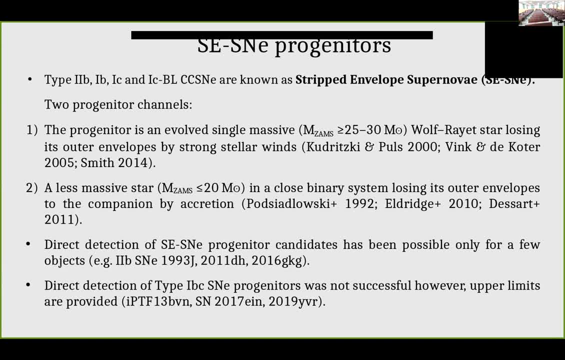 outer envelope by strong stellar wind And the second channel is possibly with smaller progenitor masses, less than 20 solar mass, in a closed binary system, losing its outer envelope to the companion by accretion, And it is interesting to note that this is 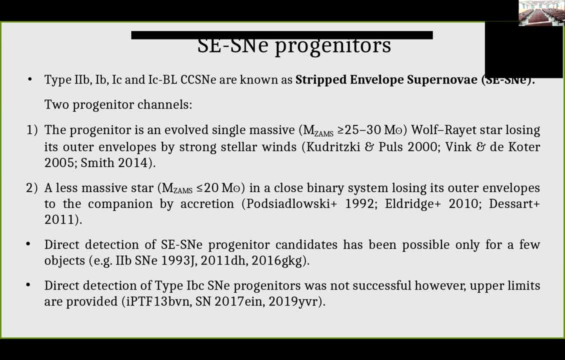 the first-time study to show that direct detection of stripped enveloped progenitor candidates have been possible only for a few cases, for example, supernovae 1993J, 2011DH and 2016G KG. However, direct detection of type 1BC progenitors have not been successful. 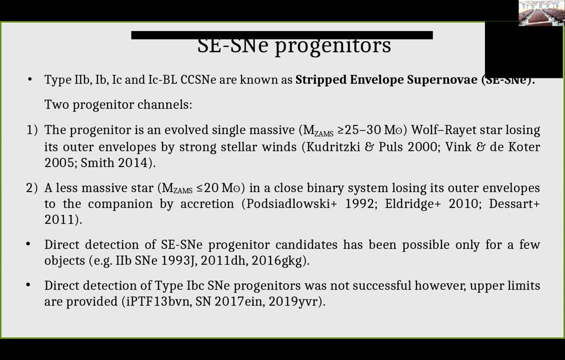 until the date but upper limits have been provided. For example, in IPDF, 13 BBN and 2017 BBN, they have been provided with a higher limit than the upper limit. So this is a good example of a supernovae that are not successful until the date but upper limits. 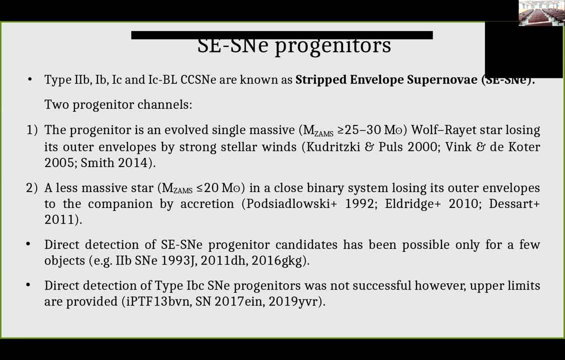 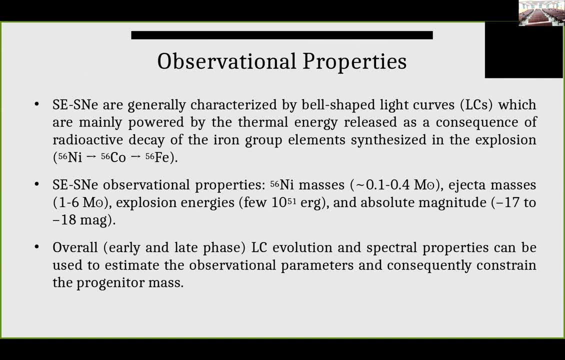 have been provided, For example, in IPDF 13 BBN and 2017 BBN and 2015 BBN- And this is a EIN- and 2019 YBR. So stripped enveloped supernovae are generally characterized by bell-shaped structure, which 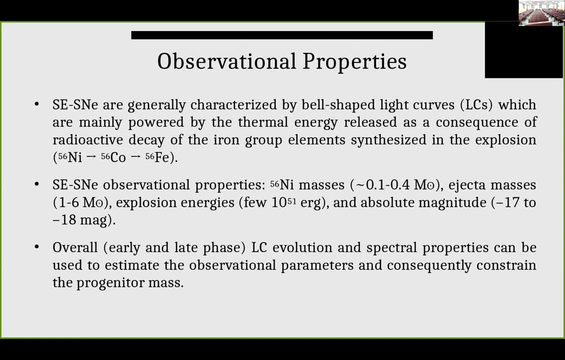 is mainly powered by thermal energy released as a consequence of nickel to cobalt and iron decay, And the observational properties of stripped enveloped supernovae are diverse, and their nickel masses have range of 0.1 to 0.4 solar mass and ejecta mass is 1 to 6, and similarly. 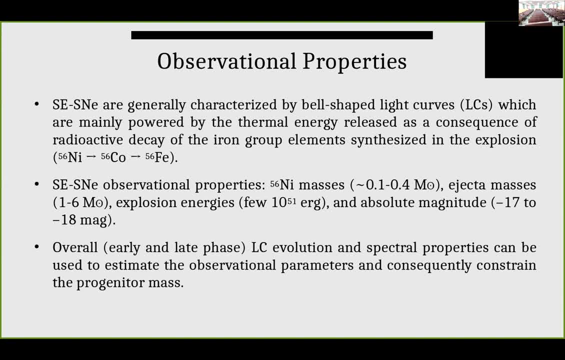 the explosion energy and also the absolute magnitude has a wide range: minus 16 to minus 18 magnitude. So overall the early and late phase light curve values are very similar. In addition, the spectral properties can be used to estimate the observational parameters. 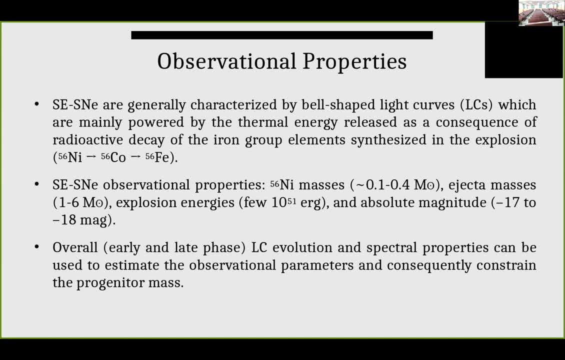 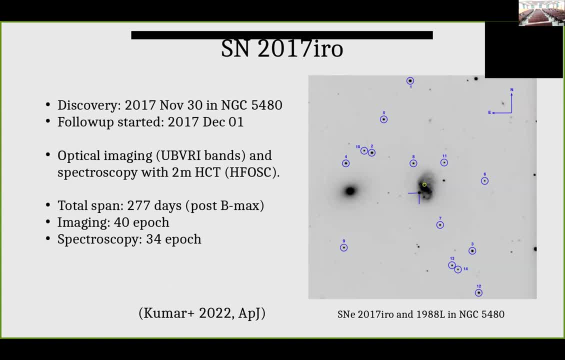 and consequently, we can constrain the progenitor masses. So, considering an opportunity of a nearby supernova type 1b, we investigated its observational properties in detail And this object was discovered on 30th of November 2017 in NGC 5480. 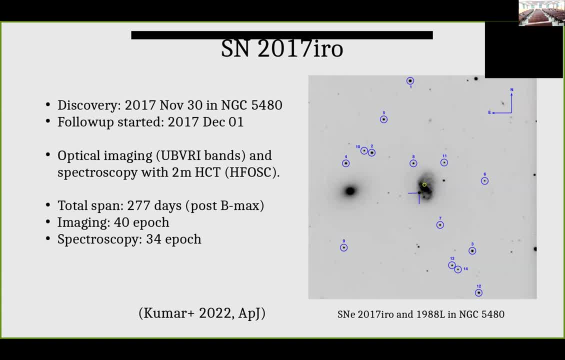 And we started its follow-up from 1st of December, And UVRI optical imaging and spectroscopy were obtained with a 2-meter Himalayan general telescope with HFAS instrument And the total span was around 277 days and we obtained around 40 and 35 epoch of imaging. 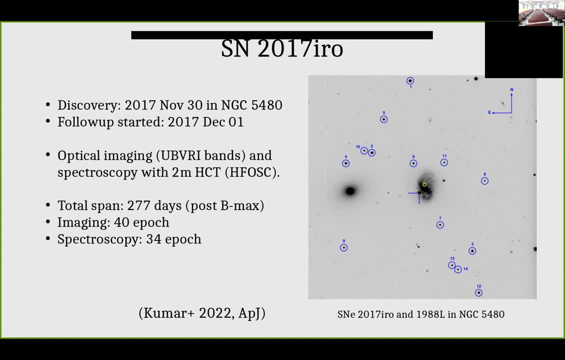 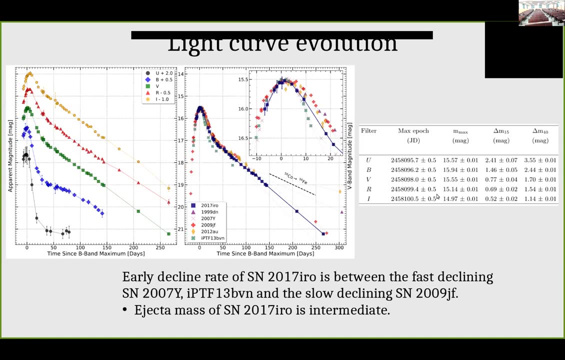 and spectroscopy. In the right panel this is showing the location of the supernova 17.. And another event which was also occurred in the same galaxy: supernova 1998L. So this is the light curve evolution. In the left panel you can see the evolution of apparent magnitude. 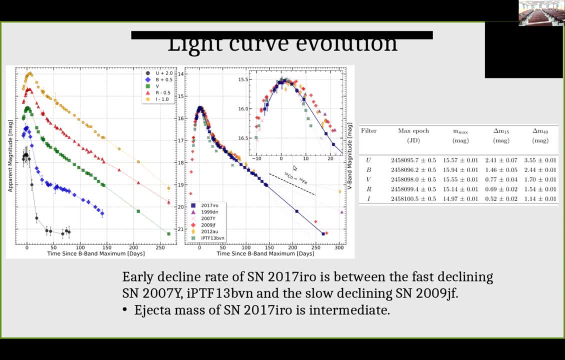 And in the right panel we have compared the event magnitude with other similar type of events And we have a study starting from early phase to the late phase. So this is in this table. I am presenting the various parameters, like delta M15, which 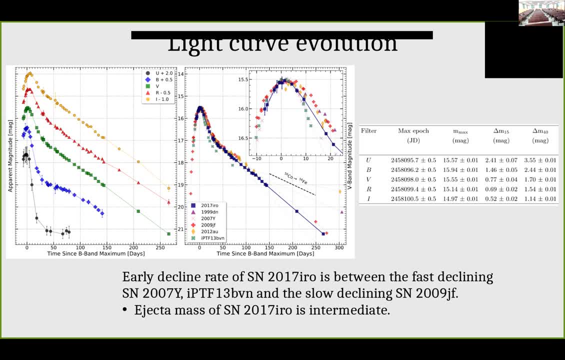 is parameter the decay of magnitude from the maximum within 15 days, and also delta M40 parameters. So, in the right panel, In the right panel, In the right panel, In this legend, you can see that the evolution, early evolution, of 17 IRO is in between the 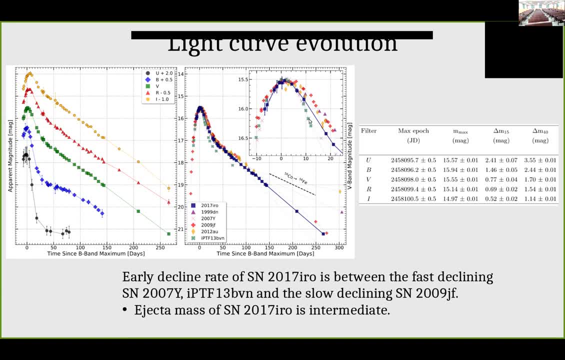 first evolving some of the events like 2007 Y, IBTUF 13, Vivian, and slow declining event like supernova, 2009, JF. So this, kindly, this is a kind of indication, Okay, Indication that ejecta mass up to 17 IRO is intermediate between these slow and fast declining. 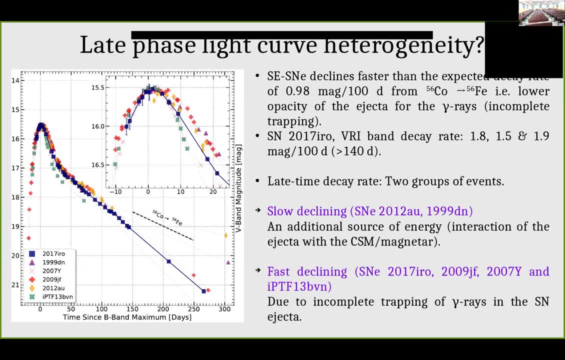 events, And here I am comparing the late phases. So the steeped envelope supernovae: they are declining faster than the expected decay rate. That is, around one magnitude per 100 days. So the steeped envelope supernovae: they are declining faster than the expected decay rate. 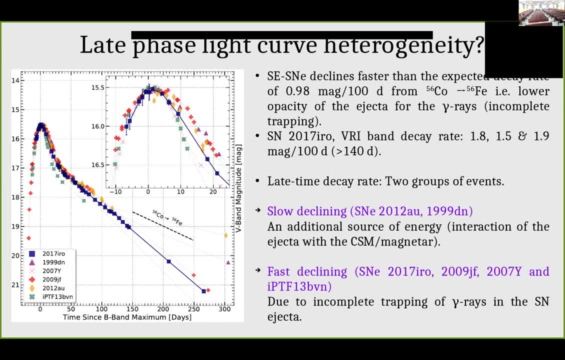 That is around one magnitude per 100 days. So the steeped envelope supernovae: they are declining faster than the expected decay rate. So the steeped envelope supernovae, they are disharmonically. Look through the image. This image is 100 Bain over here. 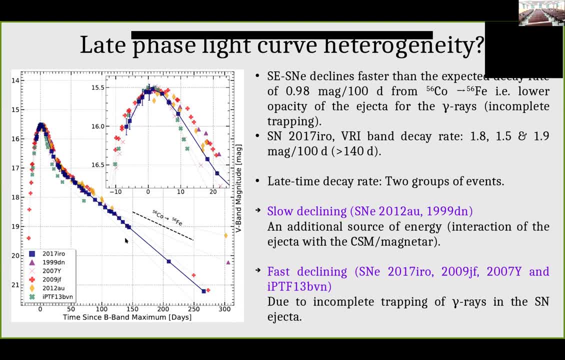 And then look around this frame after around 150 days, there seems that there are two groups of events. so one is fast declining, so fast declining, and another is a slow declining event. so in slow declining events there are two supernovae 2012 au and which one, sorry, 1999 dn, so possibly there is additional. 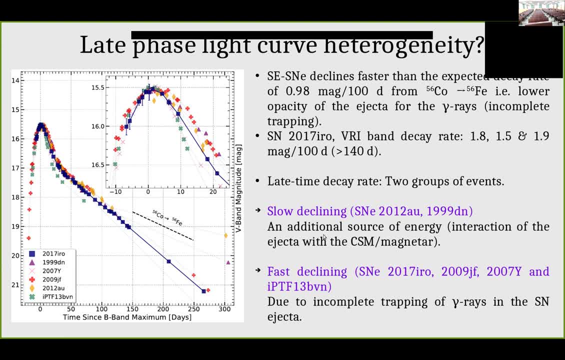 powering source may be interaction of ejecta with the csm and also the magnetar. however, there are another group which is fast declining group and supernova 2017 iro is coming in this group, including 9jf and 27y and ipdf 13- vivian. this could be possibly because of incomplete. 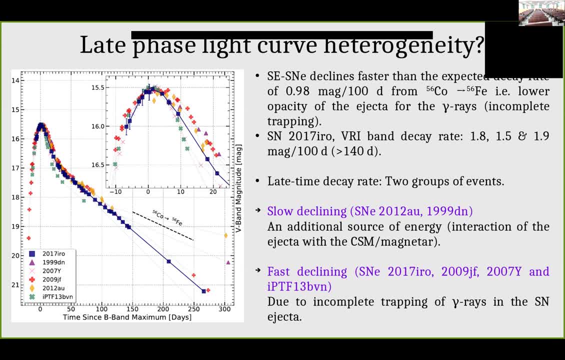 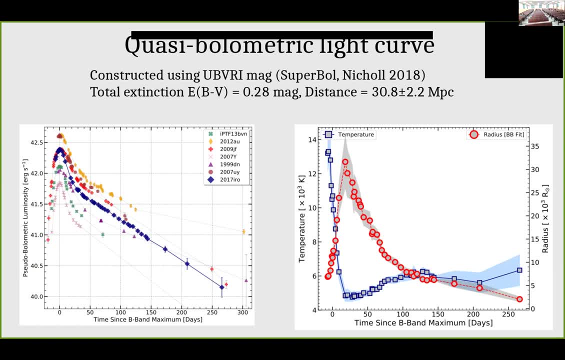 trapping of the gamma region, the supernovae ejecta. so here is the quasi volumetric light curve. so it is constructed using ubri magnitude and to construct the volumetric light curve for supernova 2017 iro we have used total extension of 0.28 magnitude and distance of around 31 megaparsec. and the left panel is 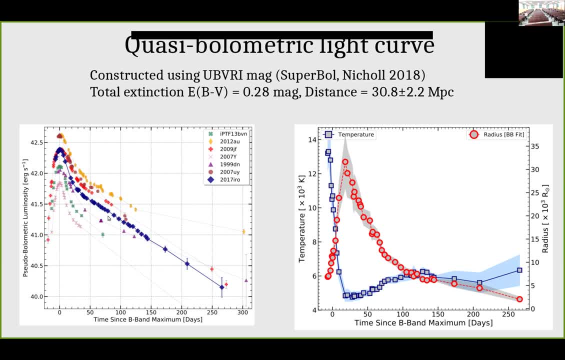 showing the volumetric, quasi volumetric light curve and compared with similar type i events, and you can see that for 2017 ro it is in intermediate between the 2012 ku and other events and the right side is the temperature and radius black body fit and here is the spectral evolution and 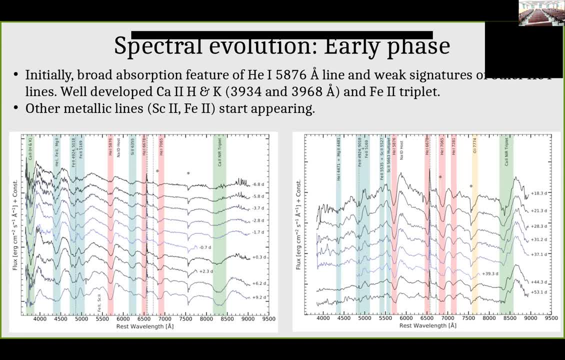 the left panel is the pre maximum to early post maximum phase and you can clearly see that various lines of helium are appearing and indicating that this is a 1v event, and also in the bluer side there are calcium 2, jhk features and also the rn features are appearing. 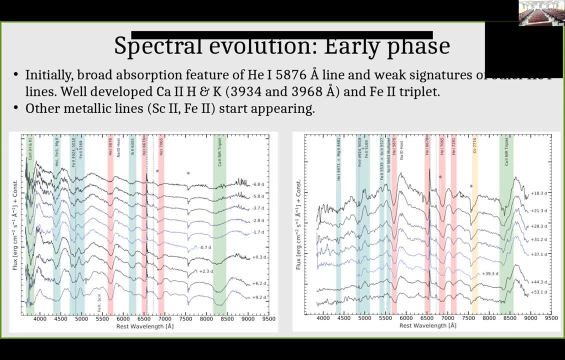 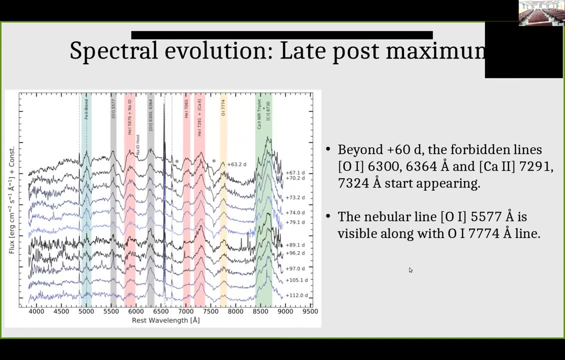 and in the right panel you can see that various features of instantium 2 and iron 2 are starting appearing here. this is a late post maximum spectral evolution beyond 60 days. you can see that the forbidden lines arising due to oxygen, 6306364 and other calcium lines are started appearing. 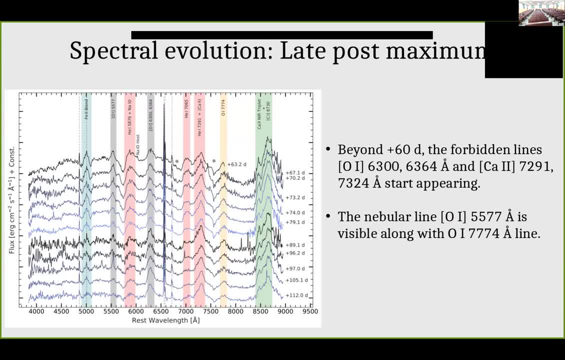 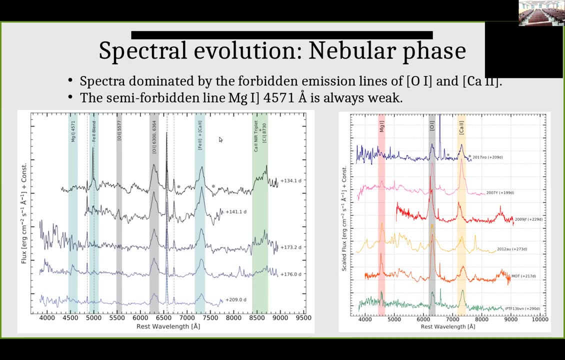 and the nebular line 5577- next term- is also visible with oxygen 1774. this is a nebular phase spectrum and it can be seen that spectra are mainly dominated by forbidden emission lines of oxygen 1 and calcium 2, and also in the right panel, the 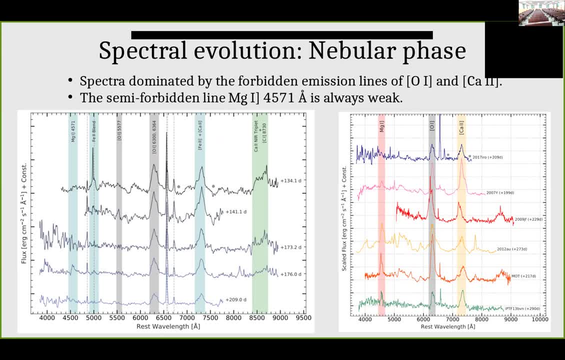 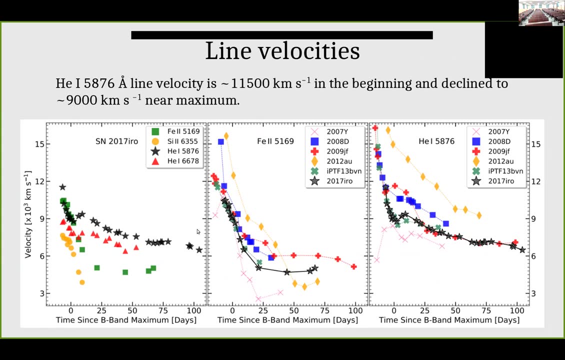 semi-forbidden magnesium line is there but it is very weak in comparison to other similar type of events. and this is the plot of line velocities and different line velocity are estimated here and plotted and the helium 15876 features that is around it reached around 11 000 and the heat is 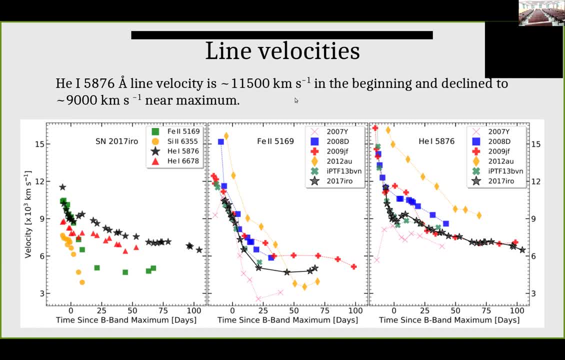 around 16, anesthesia in the area of 11 and is shadows greater than one, and the temperature of the and then declined to around 9,000 km per second. And then it can be also seen that the line velocities of helium-1 of 17 IRO is very much similar to 13 VVN. 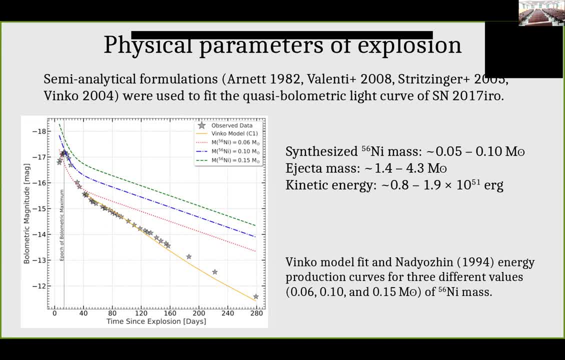 We estimated the physical parameters of the explosion using the semi-analytical formulations of various authors And the plot here is showing the. this is showing the Winko fit model And there are three additional curves which belongs to nitrogen. 1994 energy production curves. 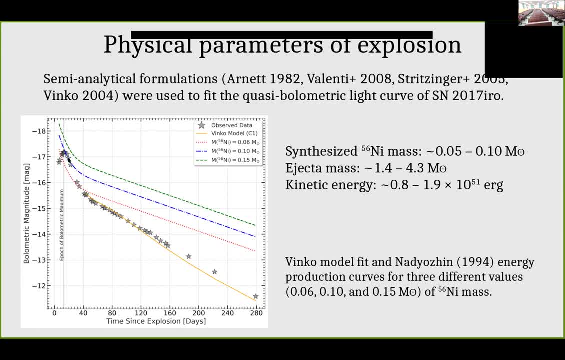 And it can be seen that the best model which is here is 0.1 solar mass for the nickel mass. So using these formulations, we estimated nickel mass in the range of 0.05 to 0.1.. And ejecta mass 1.4 to 4.3. 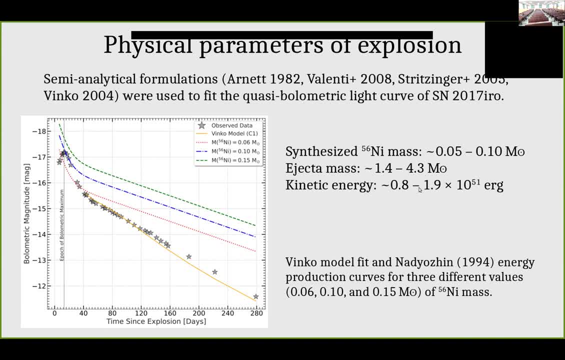 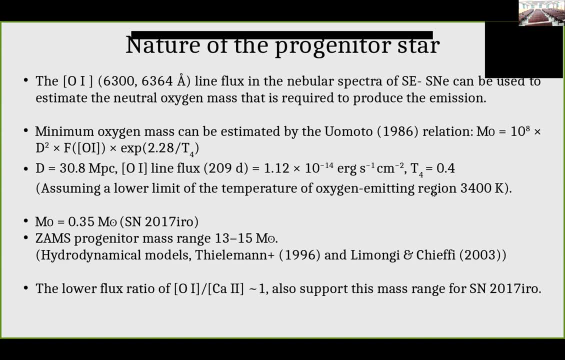 And kinetic energy: 0.8 to 1.9.. 10 to the power 51 Hertz. Here I will discuss about the nature of the pronator star, So basically the oxygen 1 star. 63006364 line flux. 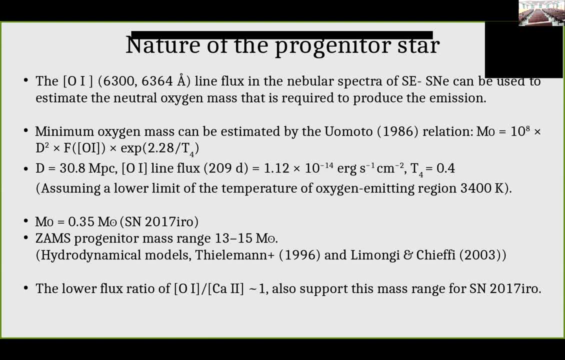 The nebular spectra of strict nebular supernovae can be used to estimate the neutral oxygen mass that is required to produce the emission And using U-MOTO 1986 relation- this relation, we can estimate the oxygen mass, Where MO is the mass of the oxygen. 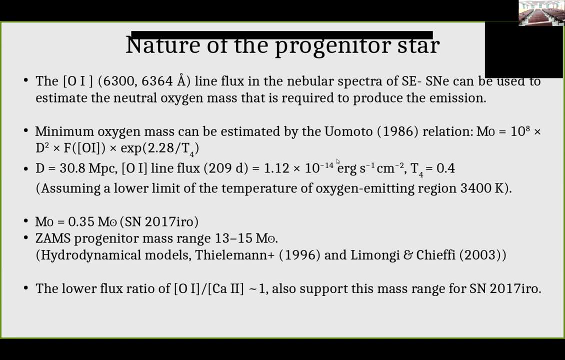 And D the distance, F is the flux of oxygen line And T4 is the temperature, that is, for the emitting region, which is in the units of 10 to the power, 4 Kelvin. So for 2017 IRO we have used distance of 30.8 megaparsec. 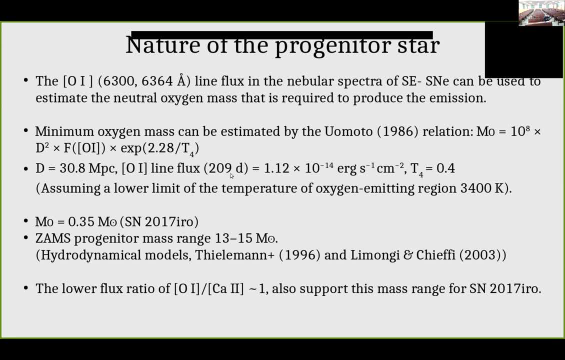 And oxygen line flux Of 2009 day. It's this value And T4 we used 0.4.. And note that we have used this as assuming as a lower limit of the temperature for oxygen emitting region, That is, 3400 Kelvin. 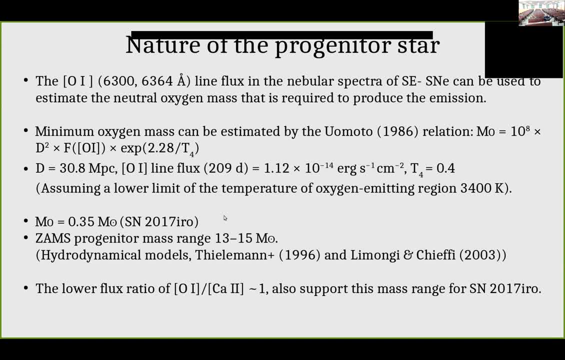 And in this way we estimated oxygen mass of 0.35 for this object, Which is for a progenitor range, progenitor mass range of 13 to 15 solar mass. And it should be also noted that we can use oxygen to calcium oxygen 1 to calcium 2 ratio to constrain the progenitor mass. 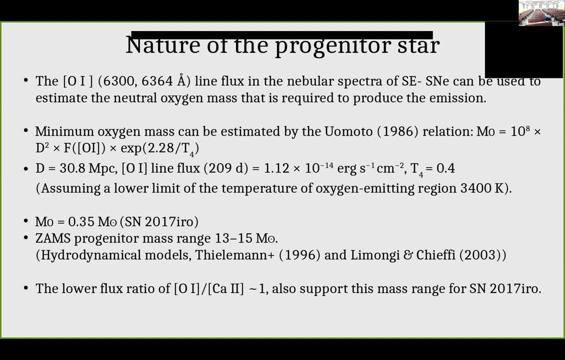 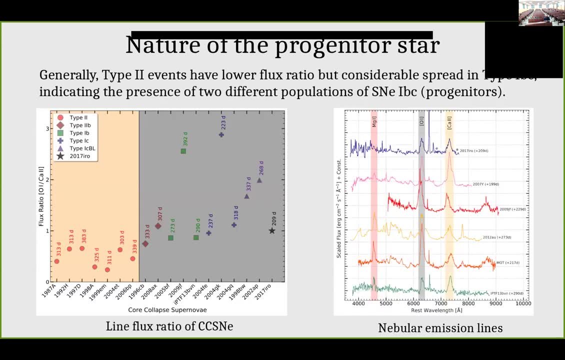 And for our object, 2017 IRO, This is around 0.1.. Sorry, it is around 1.. Which again support that this estimated mass range for 2017 IRO is towards the lower limit. And now again, nature of the progenitor star. 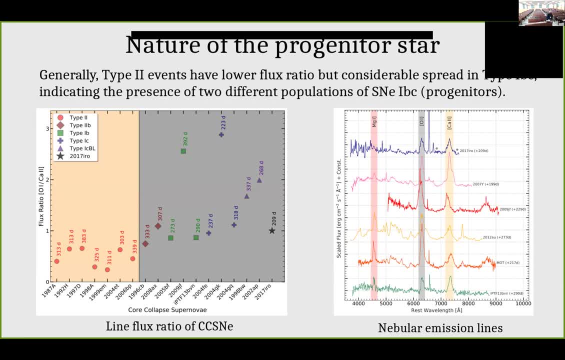 We have plotted the flux ratio of various type 2. Type 1 BC supernovae in the left panel And it can be seen that generally type 2 events have lower flux ratio And there is considerable dispersion in steep, even left supernovae. 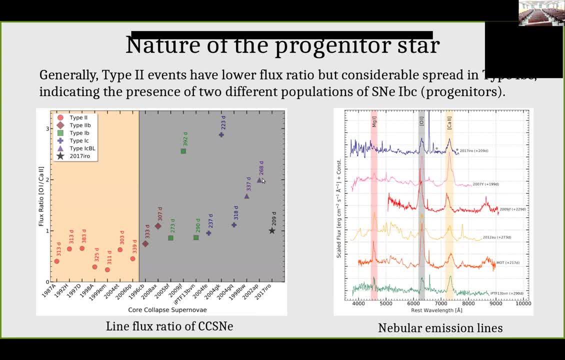 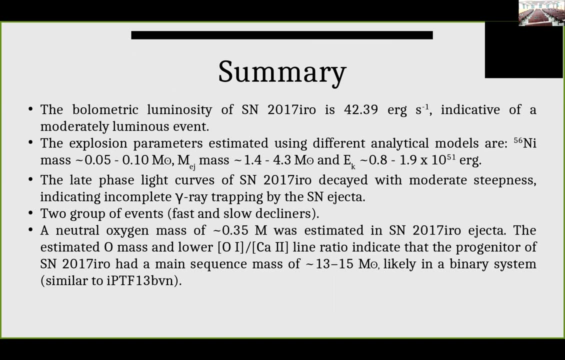 So again indicating that there is possibly there are two different populations of 1 BC And consequently they are progenitors. So, with all this, this is the summary of my presentation. The volumetric luminosity of 2017 IRO is around 42.4.. 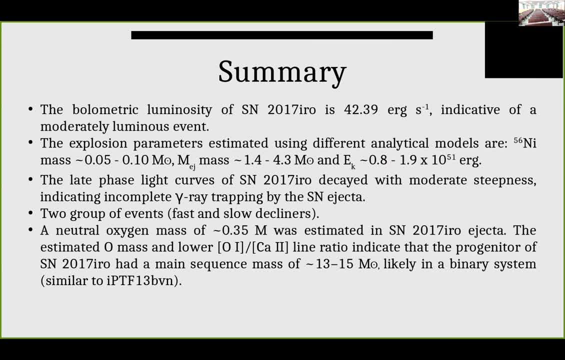 Indicating that this is a moderately luminous event And the explosion parameters are in this range. The late phase light curves decay with moderate stiffness In complete gamma ray trapping by the supernova ejector And possibly there are two group of events. 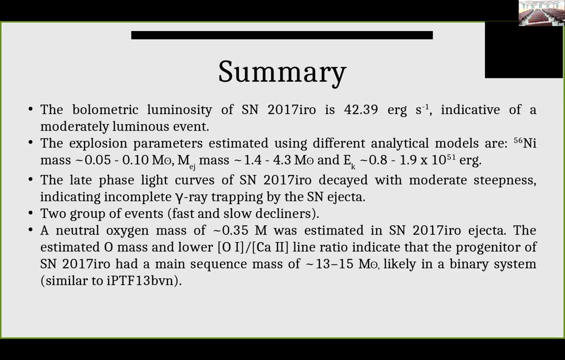 Fast and slow dictanders. And neutral oxygen was estimated around 0.35 solar mass And using the lower line ratio of oxygen, 1 to calcium, 2.. And the neutral oxygen mass, We constrain that supernova 2017 IRO had a main sequence mass of around 13 to 15 solar mass. 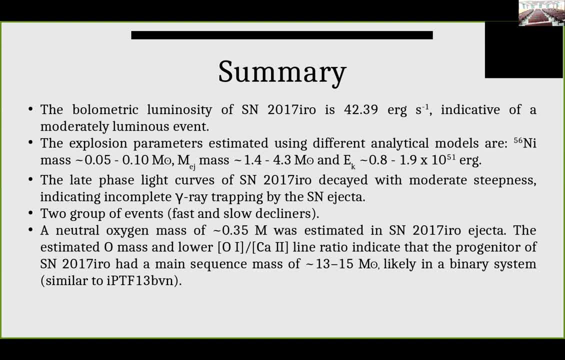 Likely in a binary system Which is very similar to supernova IPTF 13, Vivian. So thank you from my side. Thank you, Brijesh. Questions from the audience in the lecture room. Any questions from the online participants? Hello?